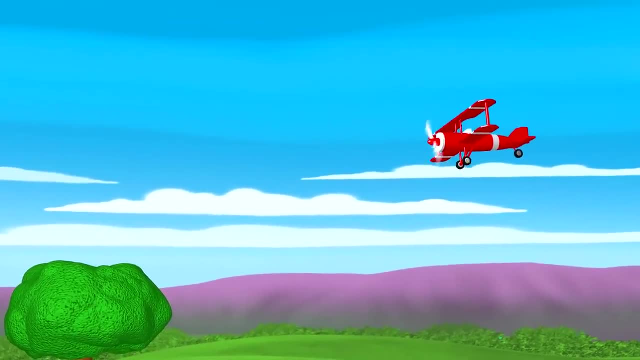 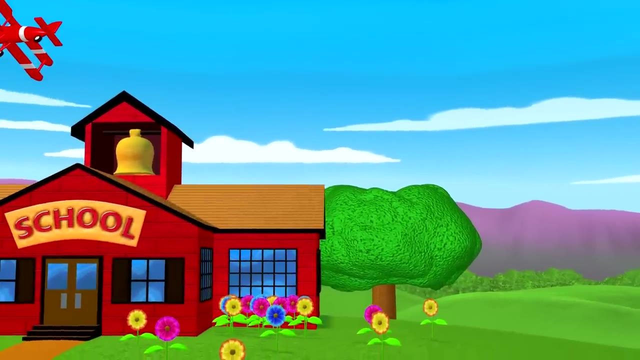 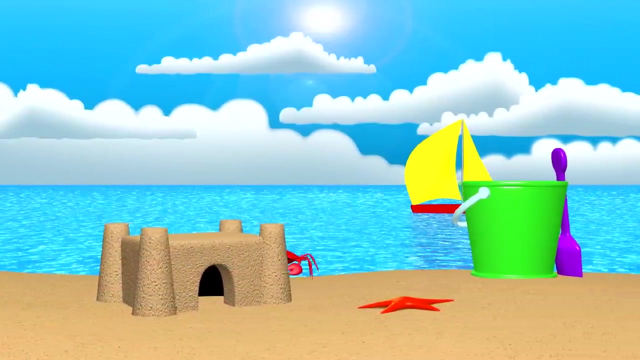 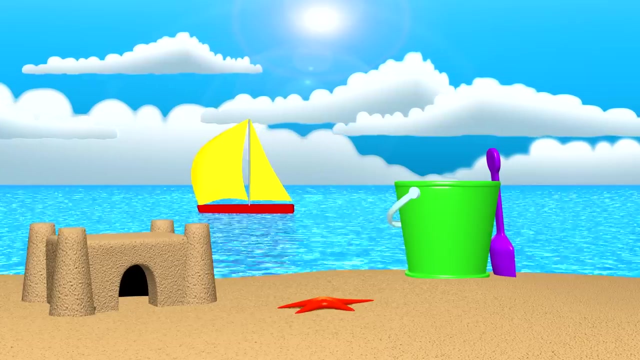 Colors, colors all around, Oh, so many to be found. Colors, colors everywhere For the whole wide world to share. The sky is blue and I can see White clouds above a big blue sea. White clouds, blue sea, Colors all around to see. 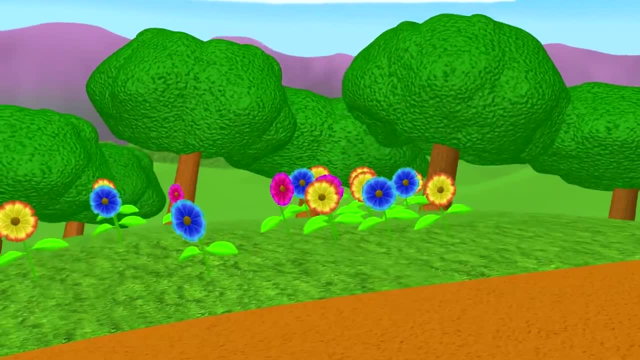 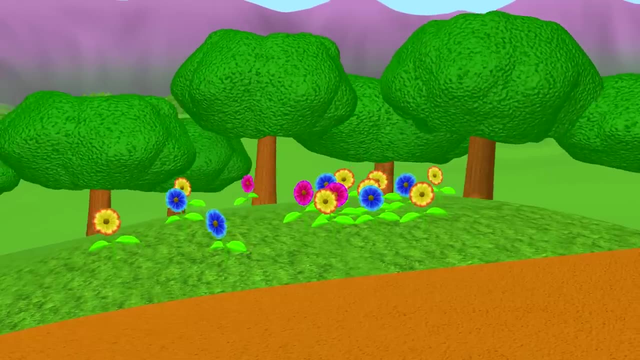 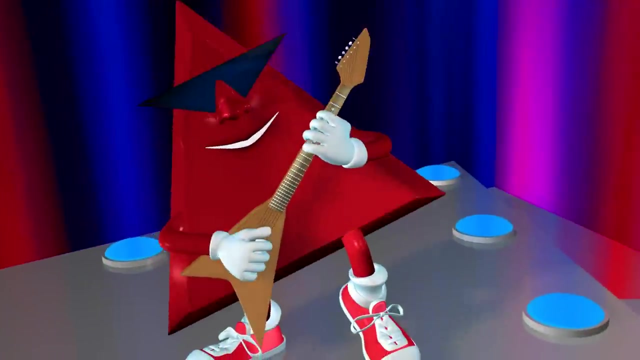 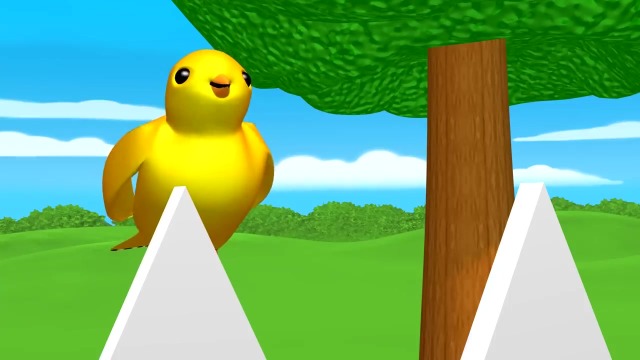 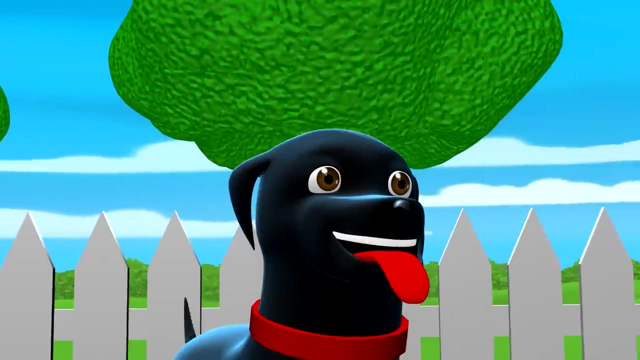 The dirt is brown, the grass is green And so are all the many trees, Brown dirt, green tree Colors all around to see. A yellow bird is singing to an orange striped cat on the ground. The black dog wants to chase him. Colors, colors all around. 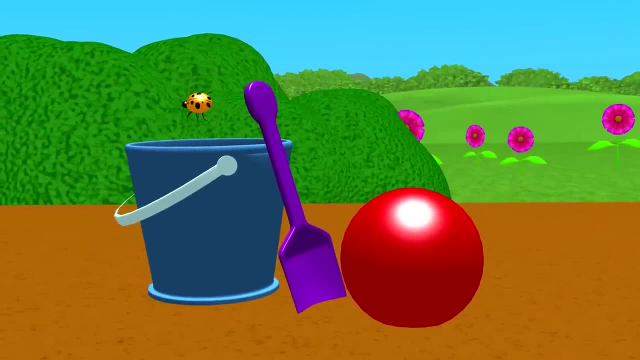 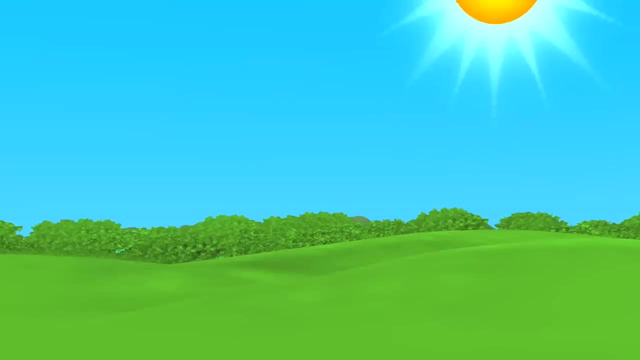 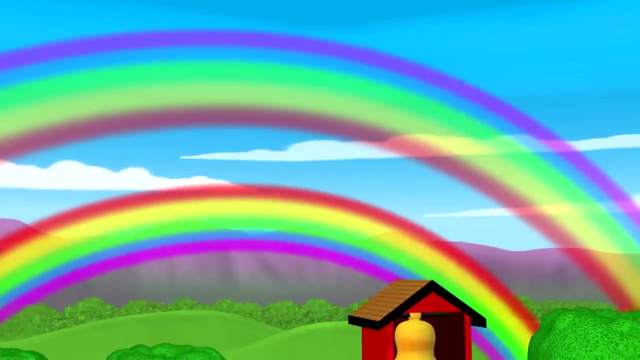 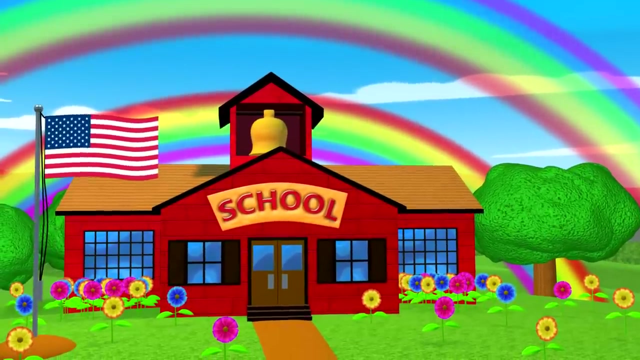 A red barn rolls around today, A purple shovel blocks its way. The sun shines down, it's light of day. It makes me want to say Colors, colors all around, Oh so many to be found. Colors, colors everywhere, For the whole wide world to share. 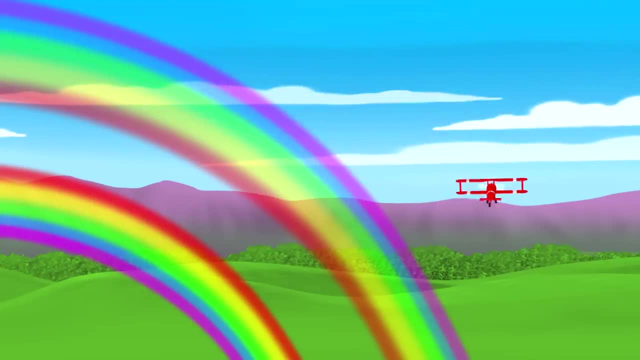 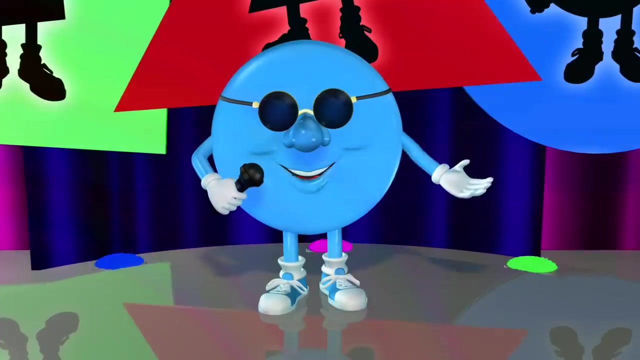 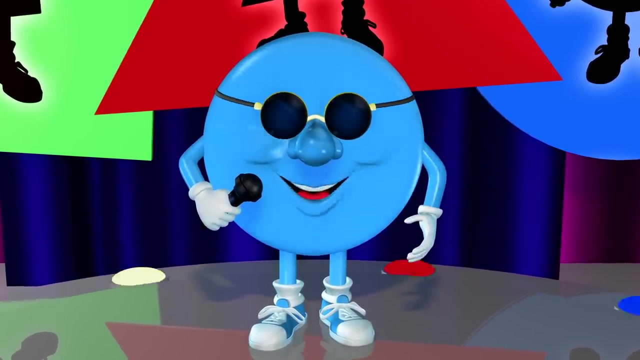 Yeah, yeah, yeah. Colors all around us, They are everywhere. Yeah, yeah, yeah, Yes, colors are all around us in our beautiful world. Let's learn some of the colors by looking at pictures together. This will be fun. Sing the colors with us. 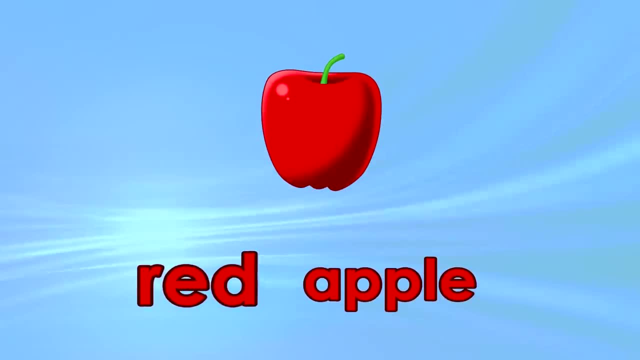 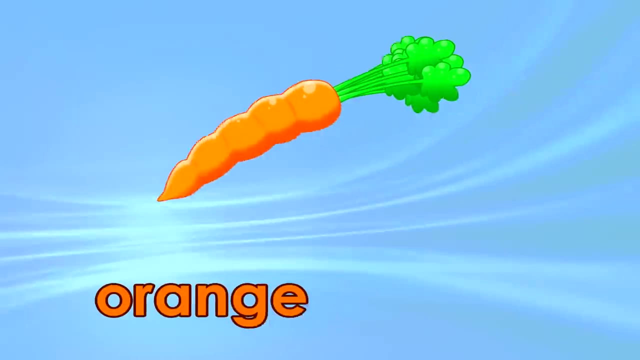 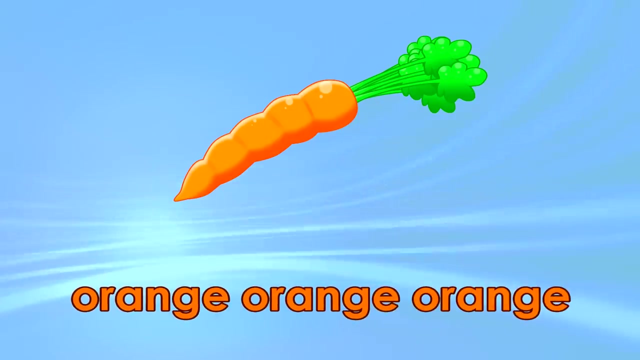 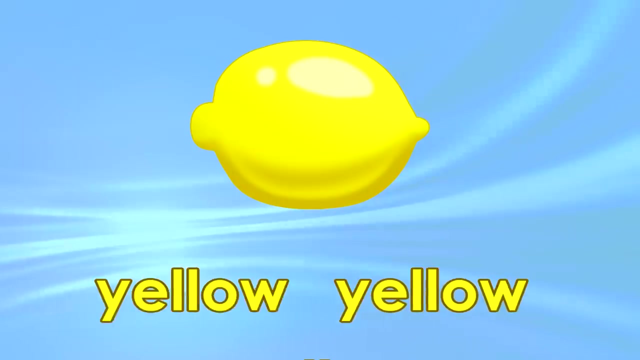 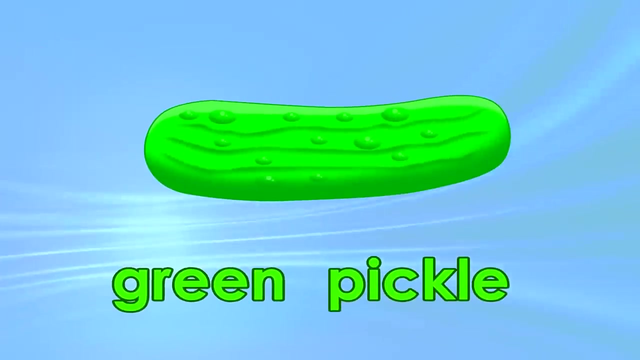 Red apple, red apple, Red red, red Orange carrot. orange carrot. Red red red Orange carrot, orange, orange orange. Yellow lemon. yellow lemon. Yellow yellow, yellow, Green pickle. green pickle. Green, green green. 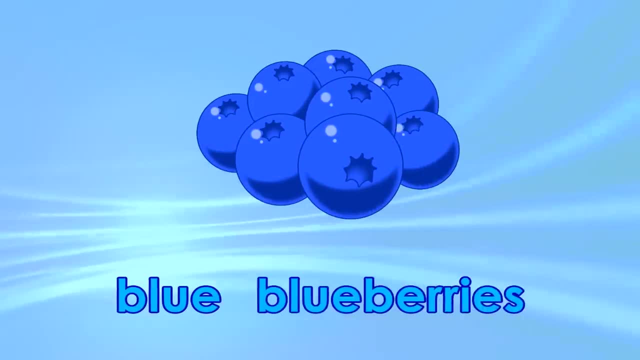 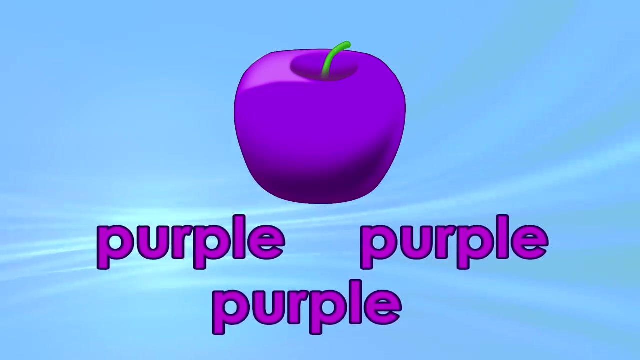 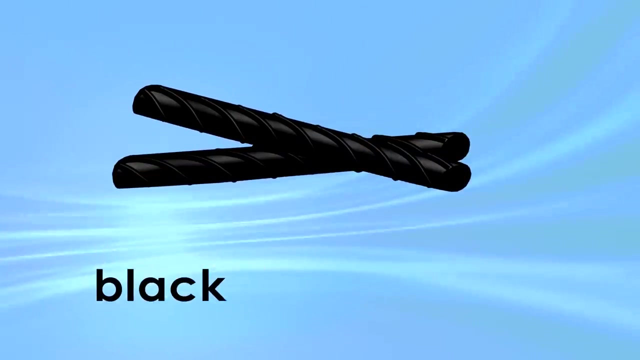 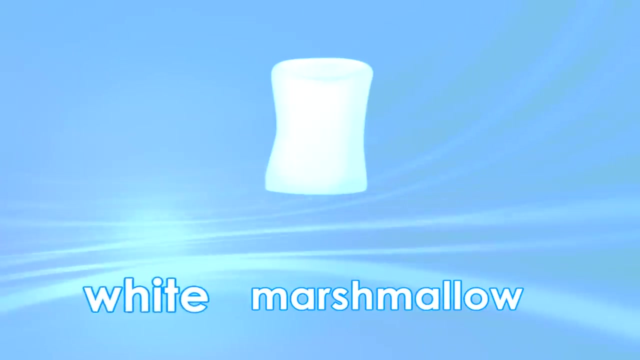 Blue blueberries, blue blueberries, Blue, blue, blue, Purple, plum, purple, plum, Purple, purple, purple. Black licorice, black licorice, Black, black, black, White marshmallow, white marshmallow, White, white, white. 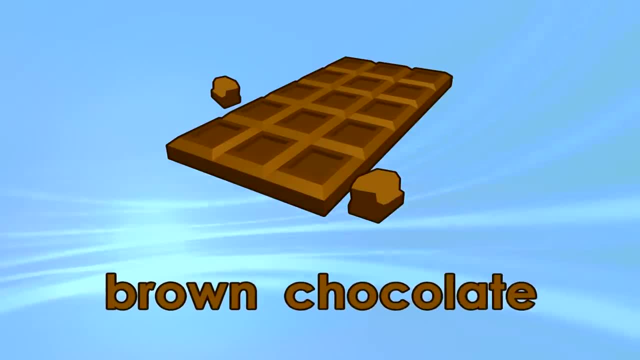 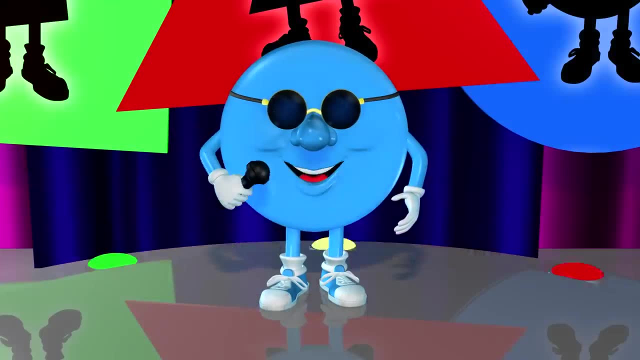 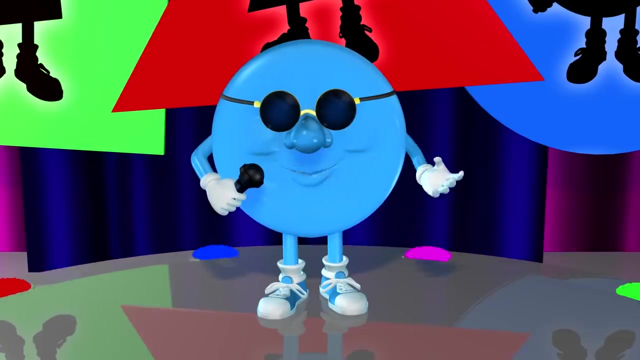 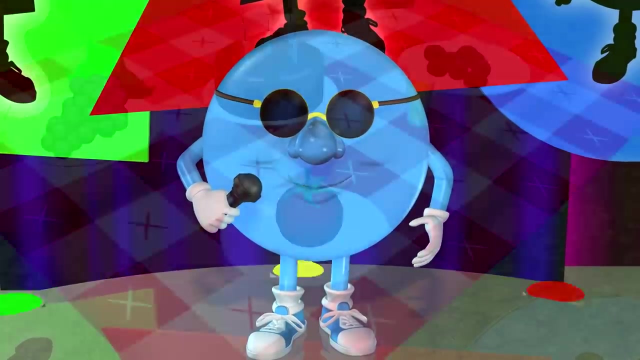 Brown chocolate brown. chocolate Brown brown brown. Wow, you're learning so much. I'll bet you can look around you now and find all kinds of different colors. Be sure to practice telling other people the colors you see wherever you go. 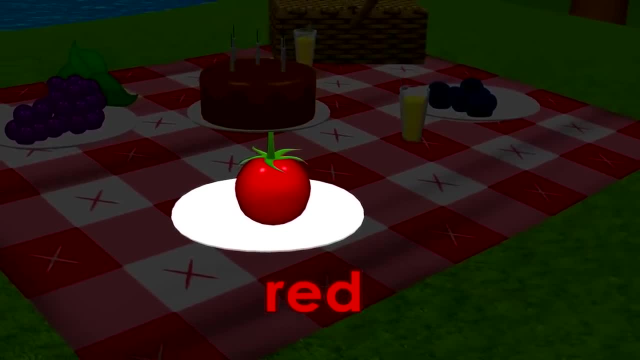 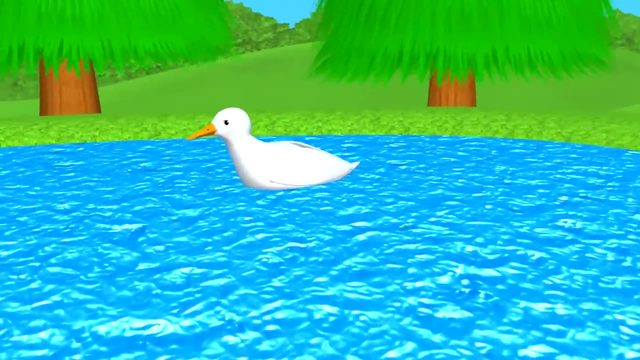 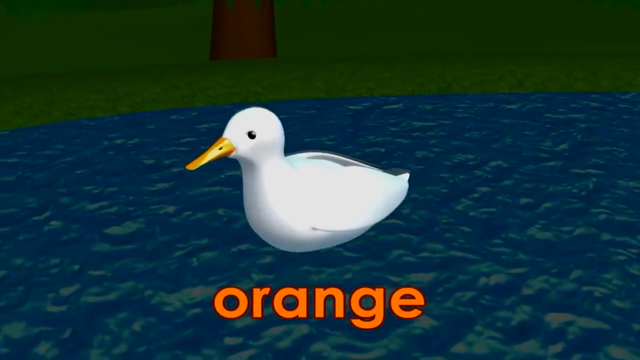 Tomatoes have a red skin, red skin, red skin. Tomatoes have a red skin. Make a salad, put some in. I love eating salad, don't you? Dogs can have an orange build orange- build orange build. Dogs can have an orange- build Colors. give me such a thrill. 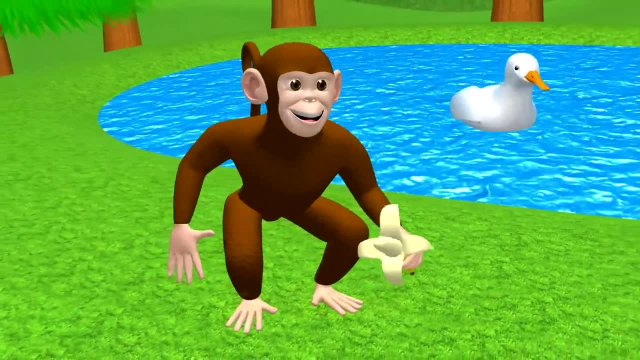 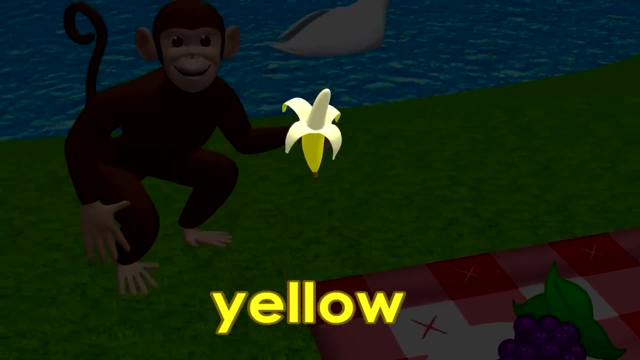 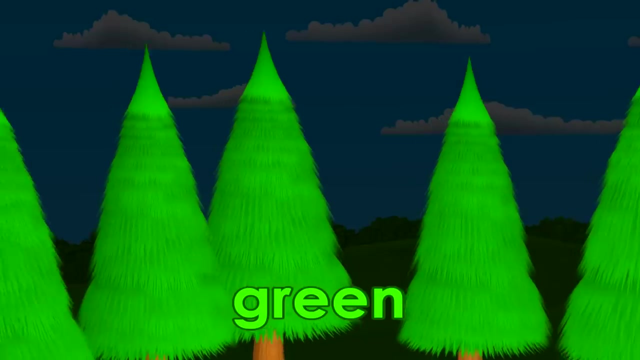 Bananas have a yellow peel, yellow peel, yellow peel. Bananas have a yellow peel and they make the monkeys squeal. The pines are always green, green, green. The pines are always green and they make the air smell clean. 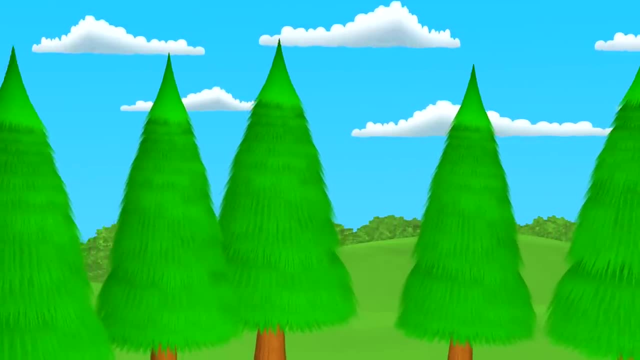 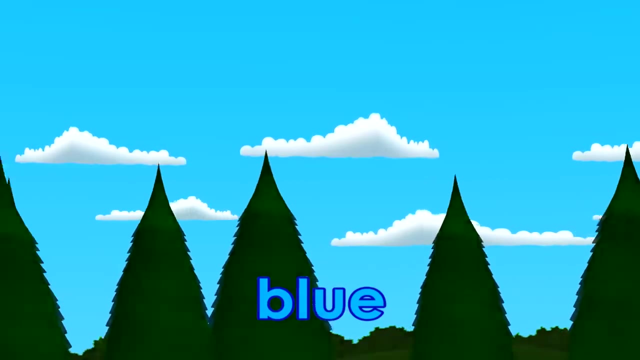 Ah, so clean. The sky outside is blue, blue blue. The sky outside is blue, blue blue. The sky outside is blue, blue blue. The sky outside is blue, and I know a J is too. Oh, look at the blue J. 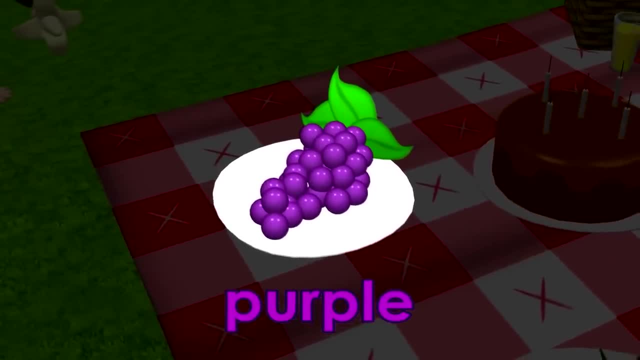 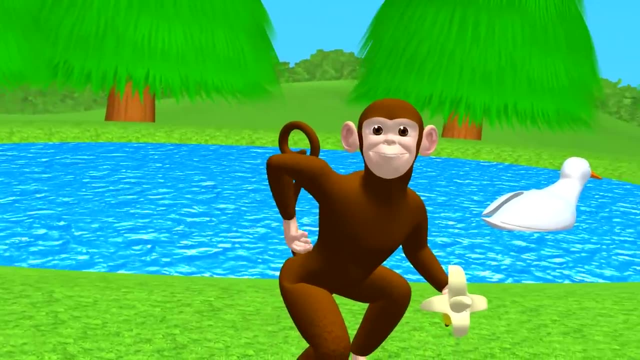 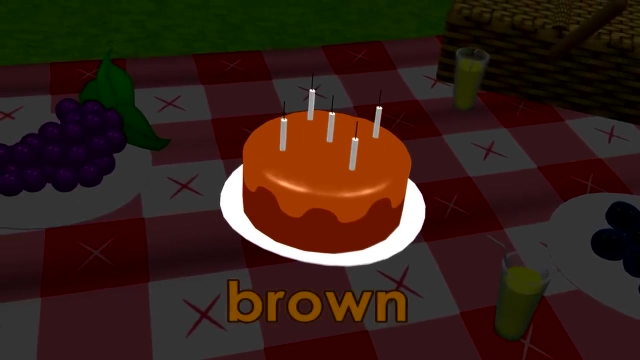 I like to eat purple grapes. purple grapes, purple grapes. I like to eat purple grapes. Then I make a sound like apes. Chocolate cake is brown, brown, brown Chocolate cake is brown. When I have some, I don't frown. 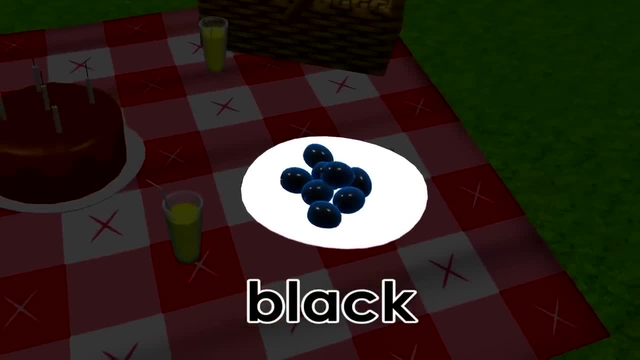 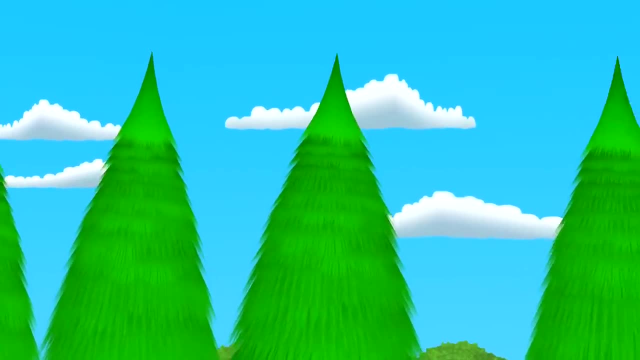 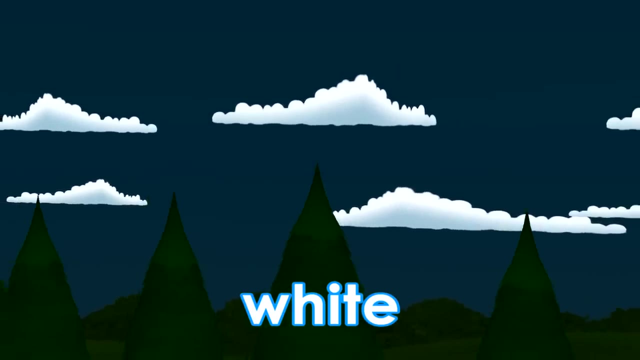 Ripe olives are so black, black, black Ripe olives are so black. I like to eat them as a snack. The fluffy clouds are white, white, white. The fluffy clouds are white In the sky. they look so bright. 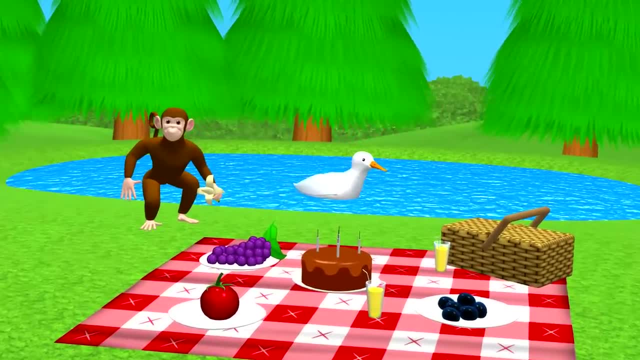 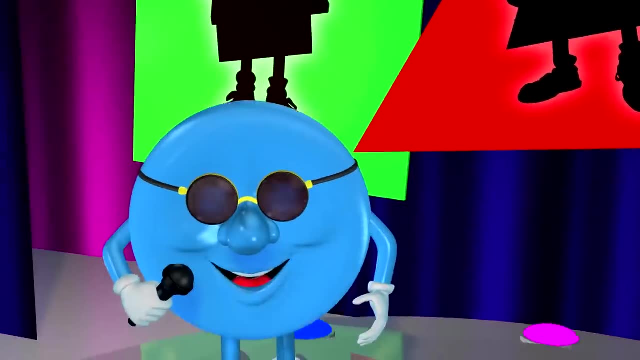 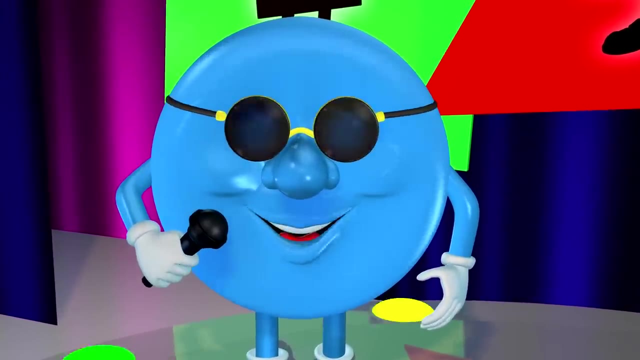 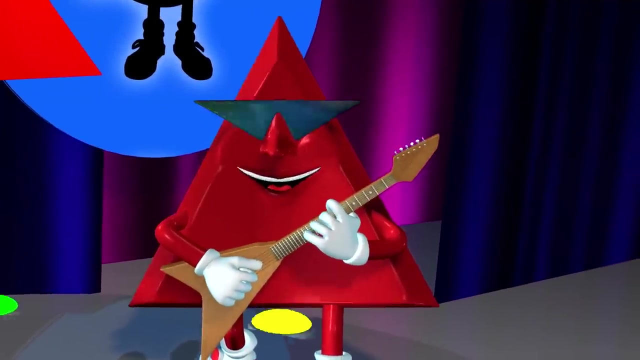 Trolley Triangle. That was really radical. I'm having so much fun learning with you, But now it's time for me to introduce my good friend, Trolley Triangle. Take it away, Trolley. Hey, hey, cool kids, Look all around us. 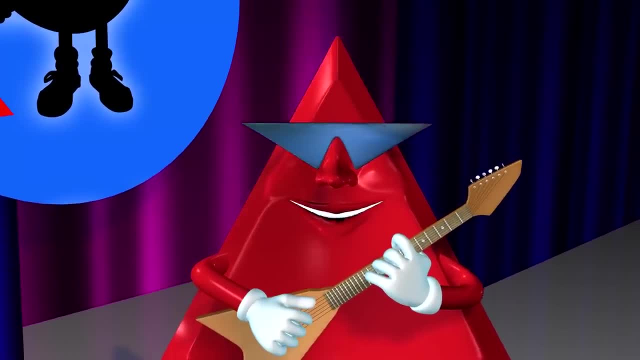 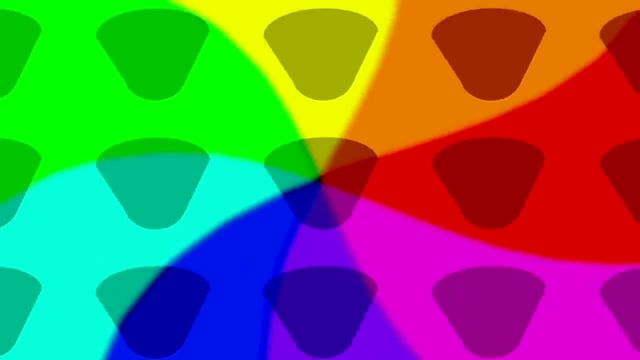 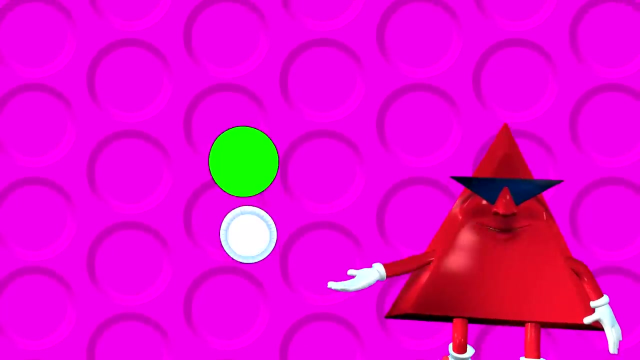 Shapes are everywhere. Let's learn the names of some of these shapes. Come on, everyone, Let's have a super time. We're going to learn our shapes and make a rhyme. A circle is round like a plate, pie or penny. If you look for a flat side, it doesn't have any. 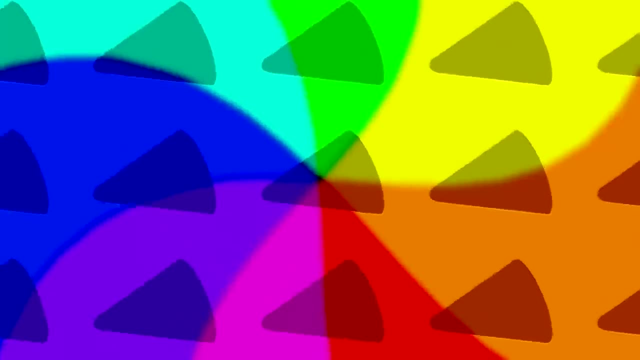 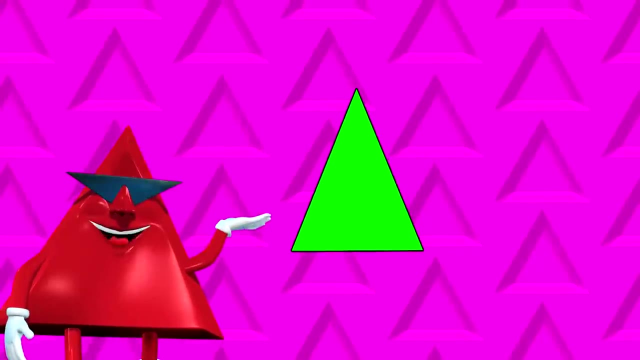 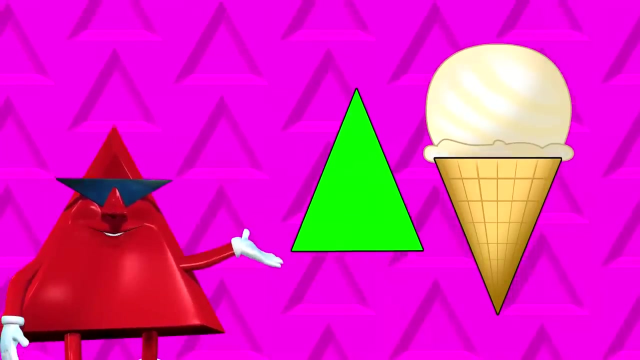 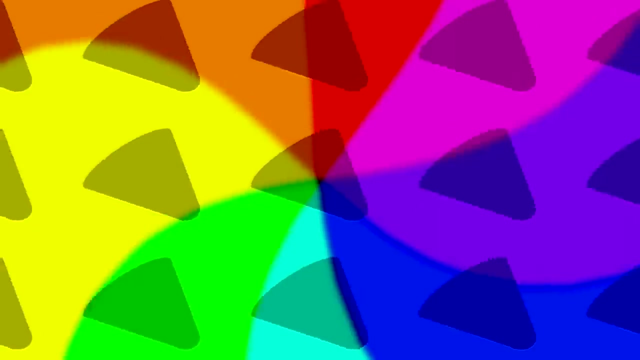 Come on everyone, Let's have a super time. We're going to learn our shapes. A triangle is pointed like an ice cream cone. It has three sides to call its own. Come on everyone, Let's have a super time. We're going to learn our shapes and make a rhyme. 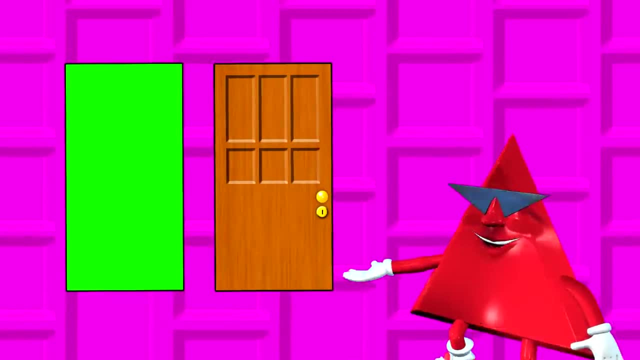 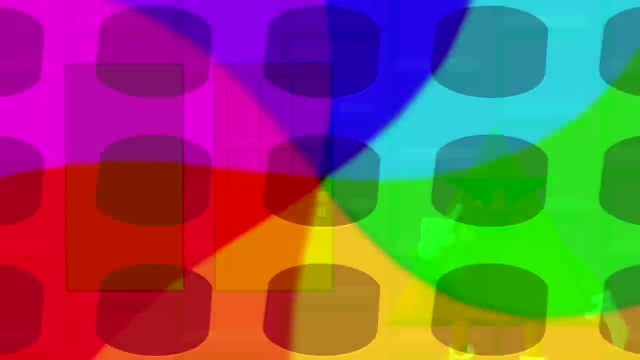 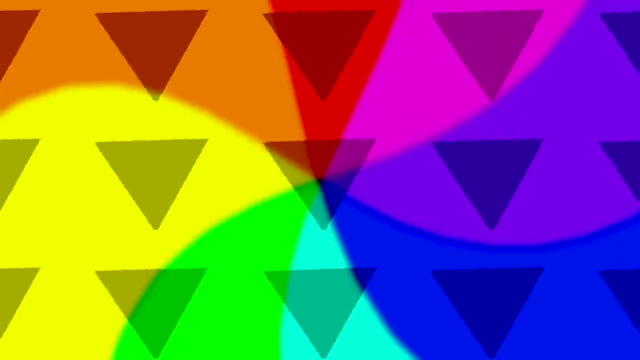 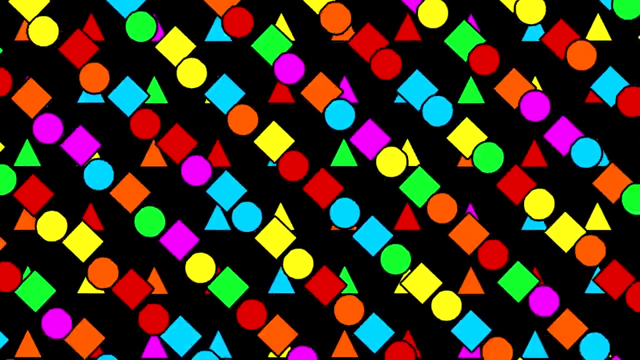 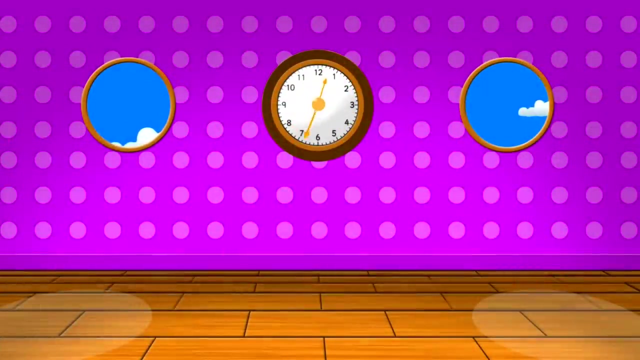 Now, a rectangle is like a door. It has four sides, No less, no more. Come on everyone. We've had a super time Now. we've learned some shapes and made a rhyme. Shapes are all around us for all of us to see. Let's point to some, just you and me. 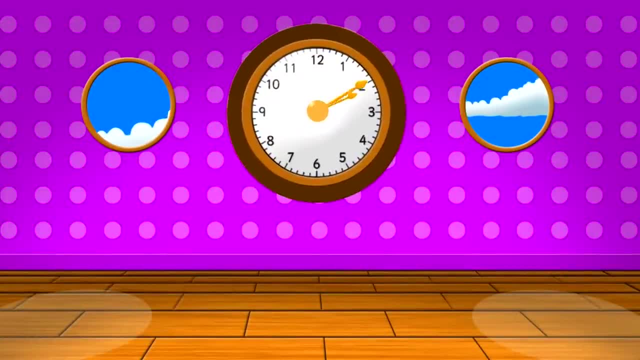 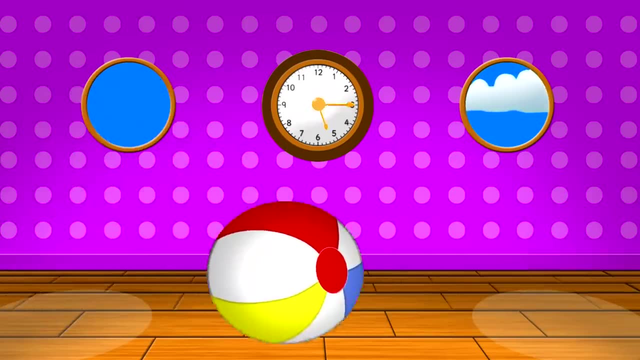 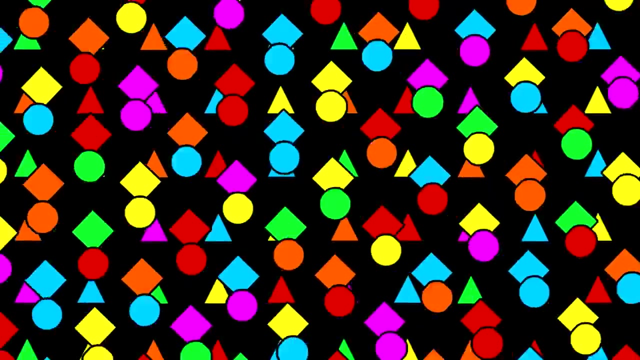 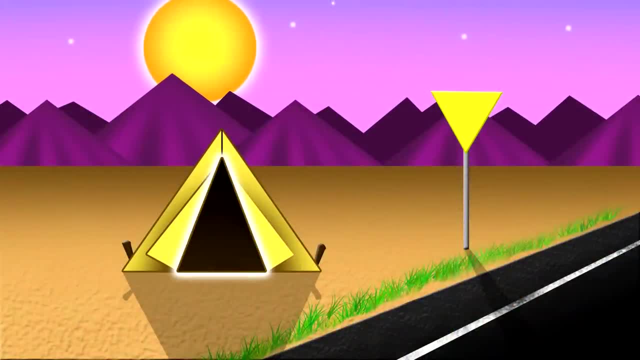 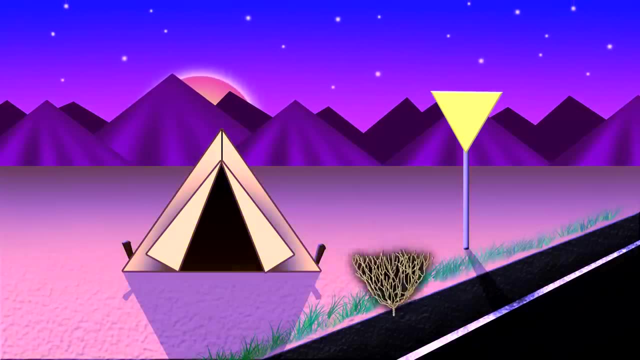 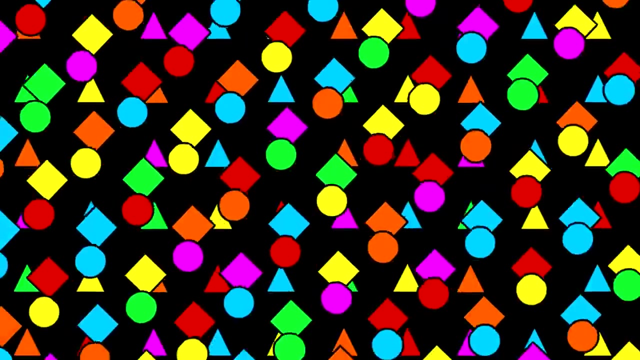 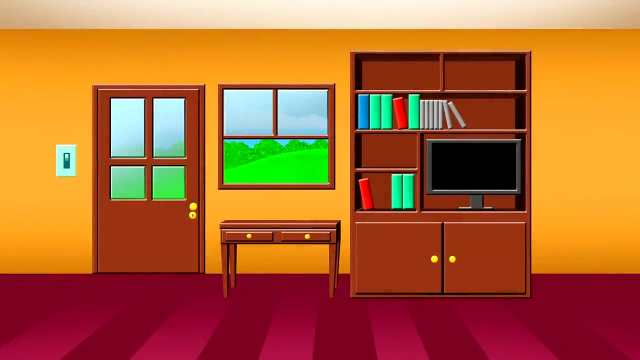 A triangle has three sides. It's pointed on the end like a little tent standing strong against the wind. Shapes are all around us for all of us to see. Let's point to some: just you and me: Shot gun Two one. 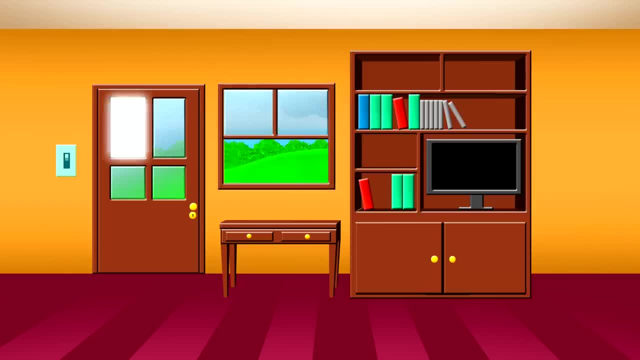 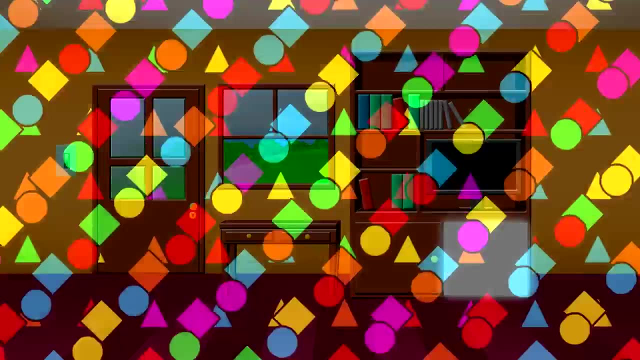 They have four sides. I'll tell you to. just let me be your guide. Rectangles are found in windows and indoors, books and papers. Now let's find some more. Shapes are all around us for all of us to see啊. 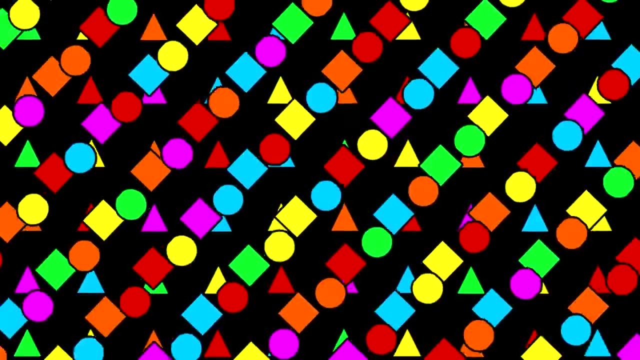 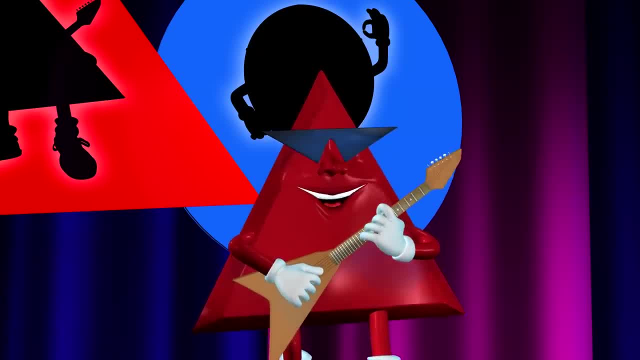 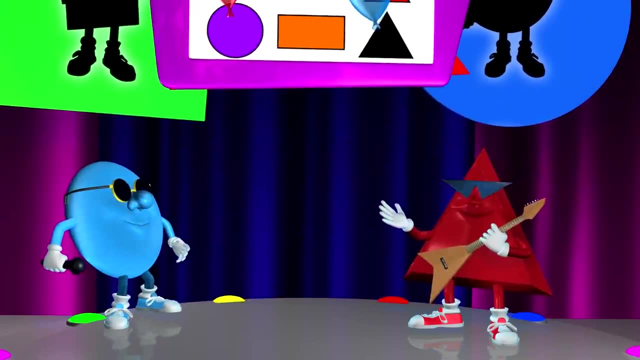 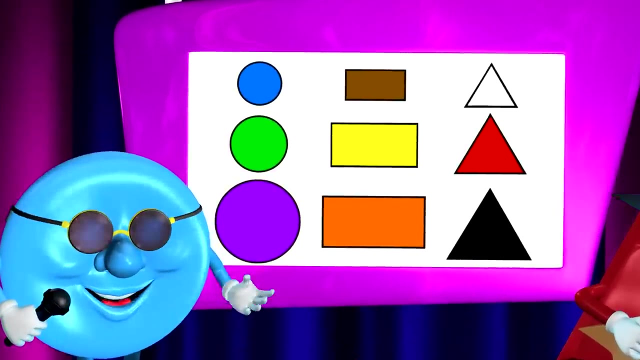 Let's point to some- just you and me- Now that we know some shapes and colors, let's play a game called What Color Is It? Look at all the shapes. They are all different sizes. Some are little, some are big and some are in between. 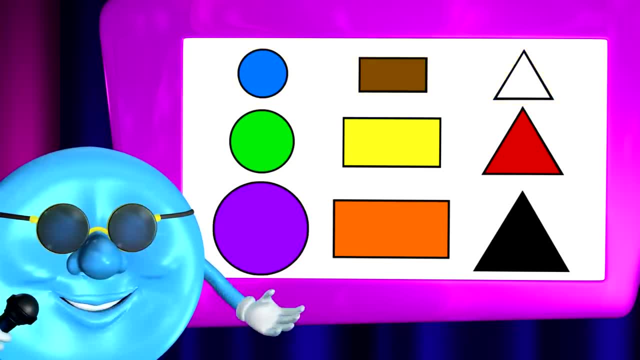 We call the little shapes small, The big shapes are called large And the ones in between small and large are called medium Neato. Now let's play the fun game. What Color Is It? with Trolley, I see a large circle. 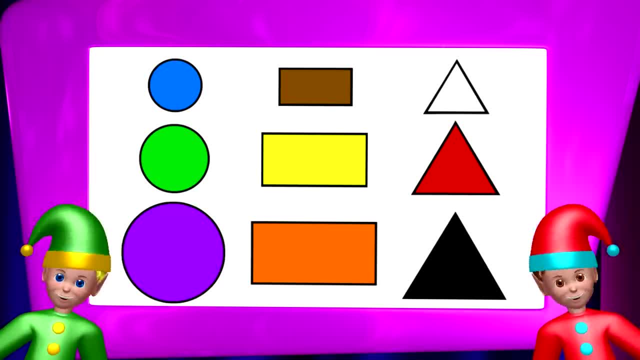 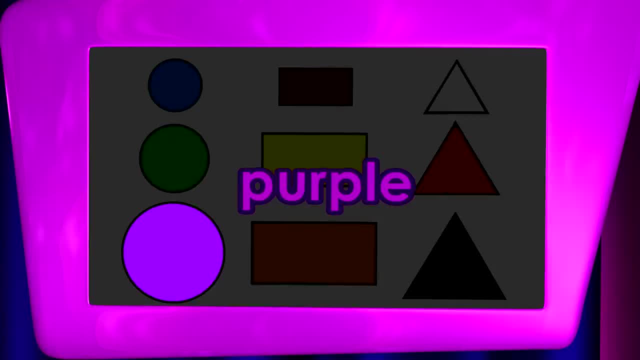 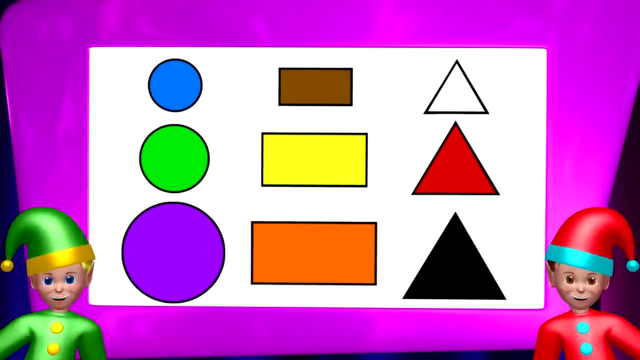 What color is it? What color is it? The large circle is purple. I see a medium triangle. What color is it? What color is it? The medium triangle is red. I see a small rectangle. What color is it? 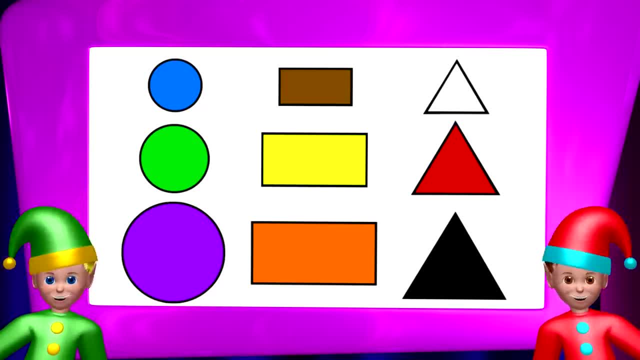 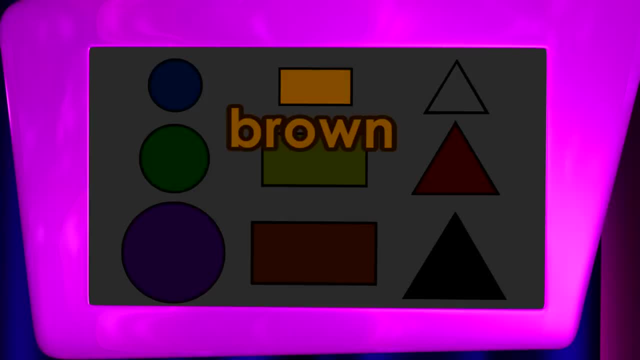 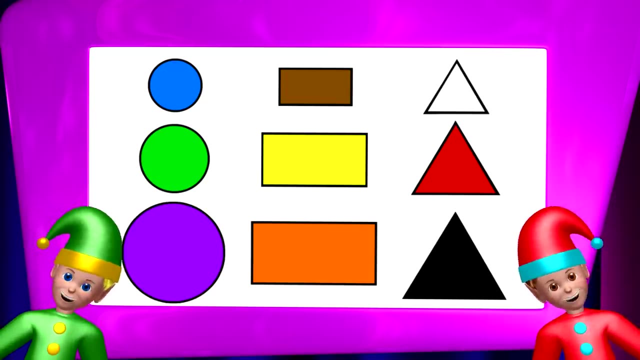 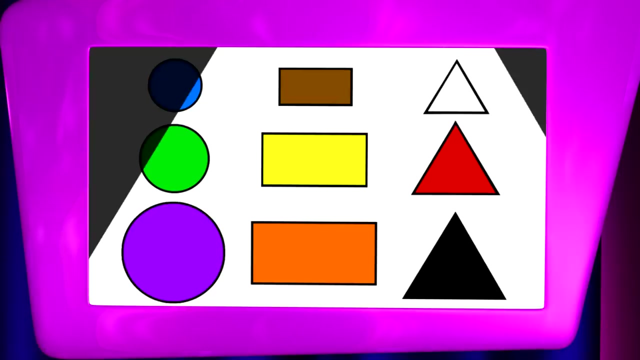 What color is it? What color is it? The small rectangle is brown. I see a large triangle. What color is it? What color is it? The large triangle is black. I see a small circle. What color is it? 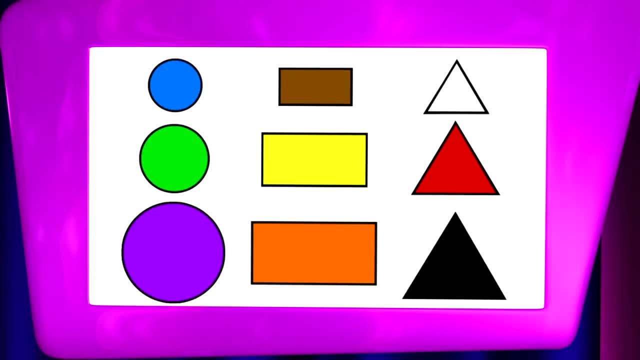 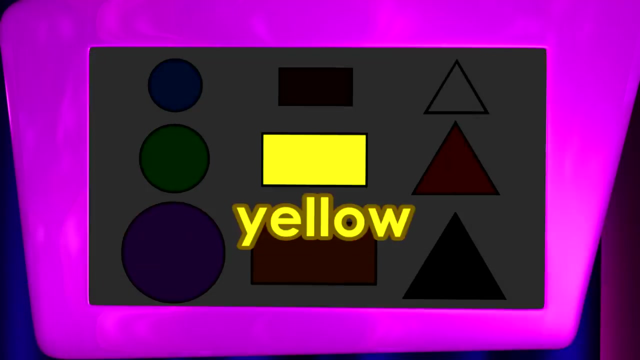 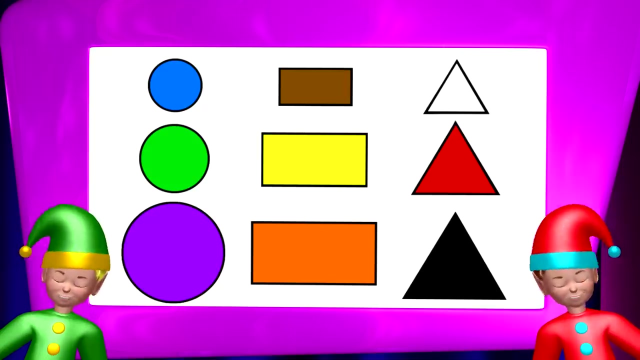 What color is it? The small circle is Blue. I see a medium rectangle. What color is it? What color is it? The medium rectangle is Yellow. I see a small triangle. What color is it? What color is it? 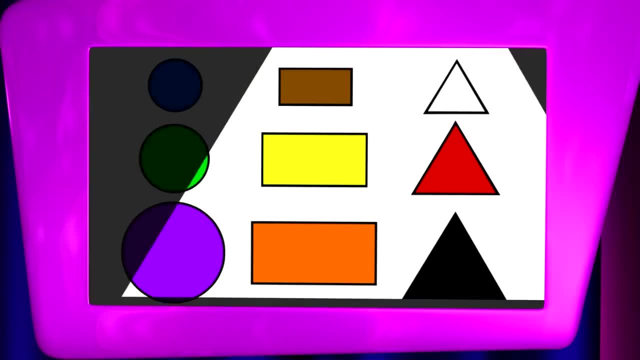 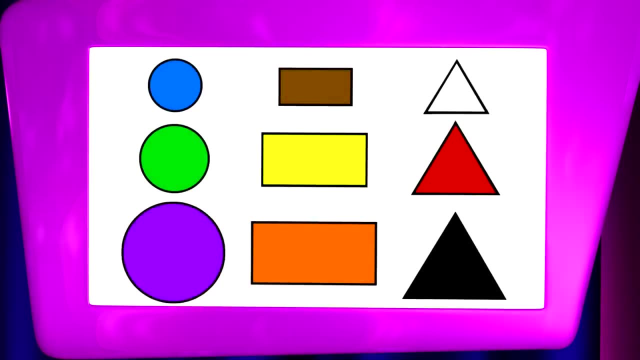 The small triangle is White. I see a medium circle. What color is it? What color is it? The medium circle is Green. I see a large rectangle. What color is it? What color is it? The large rectangle is? 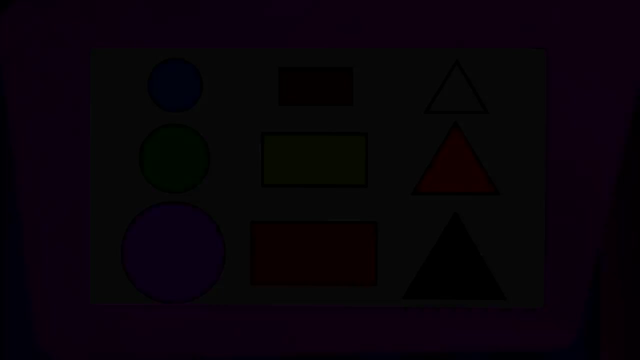 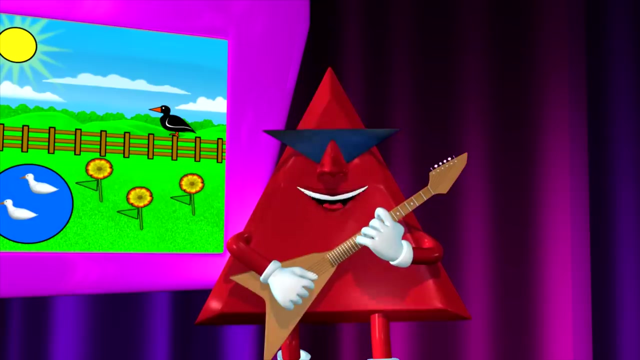 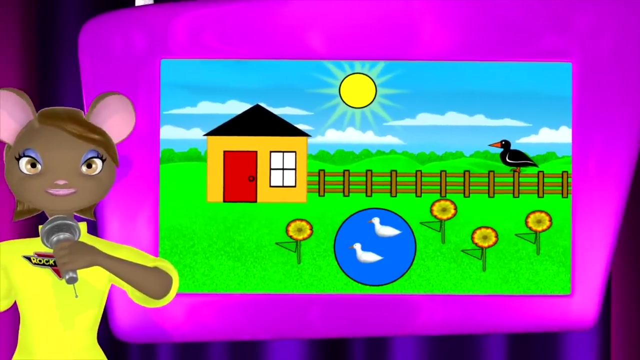 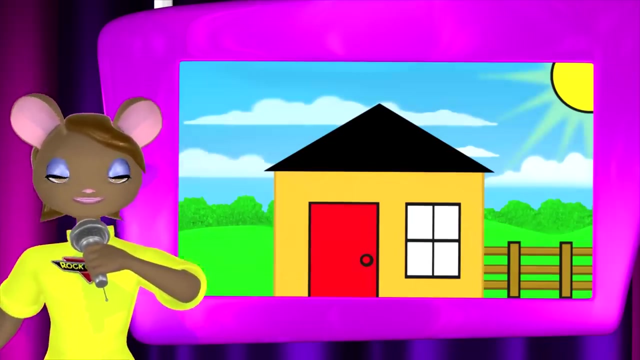 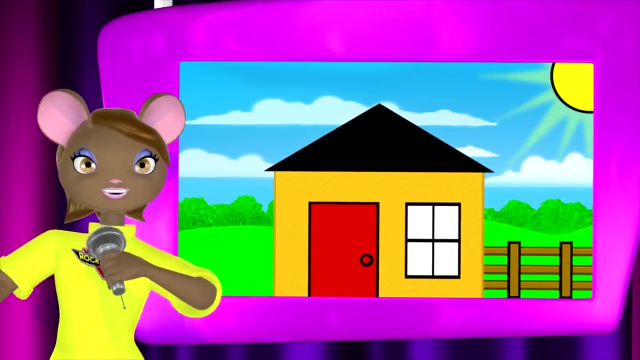 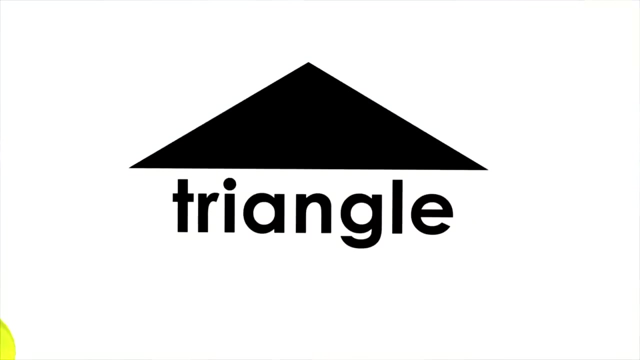 Orange, Orange. Hey, We all came to another astronaut's house. Here's to doing. well, Let's get to it. Hooray, Hooray, Hooray, Hooray. I see a purple ball that rolls around. 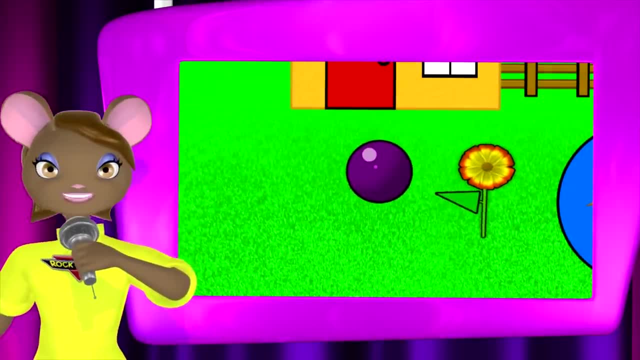 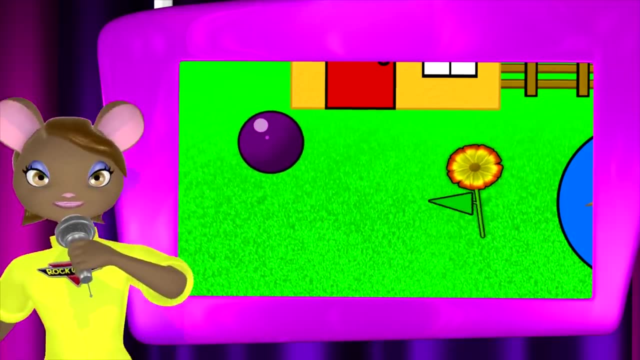 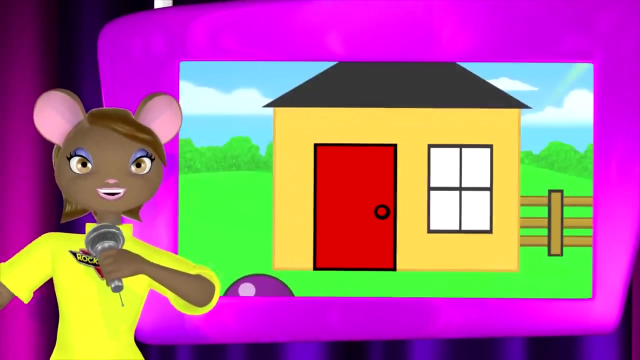 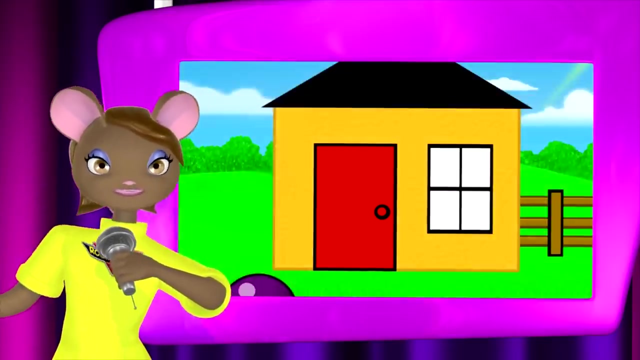 I see a purple ball that rolls around. Can you name that shape? and then touch the ground. The ball is a circle. On the front of the house there is a red door. On the front of the house, there is a red door. Can you name its shape before we sing some more? 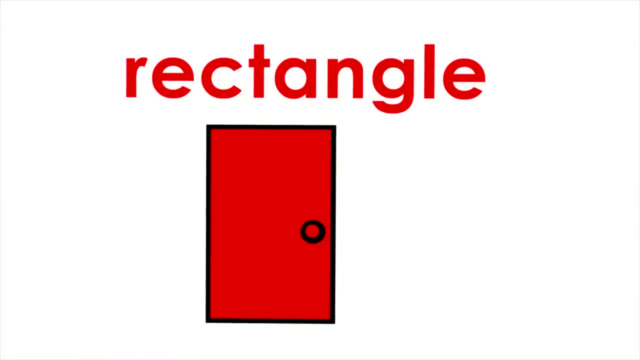 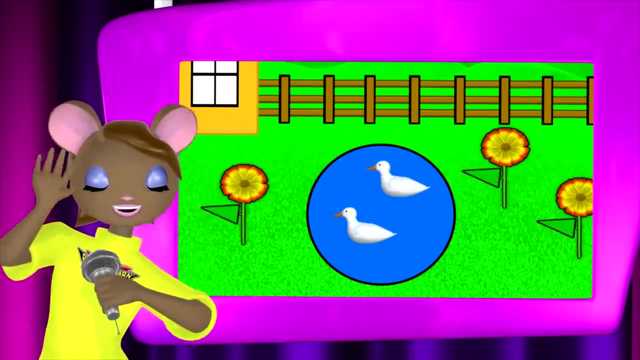 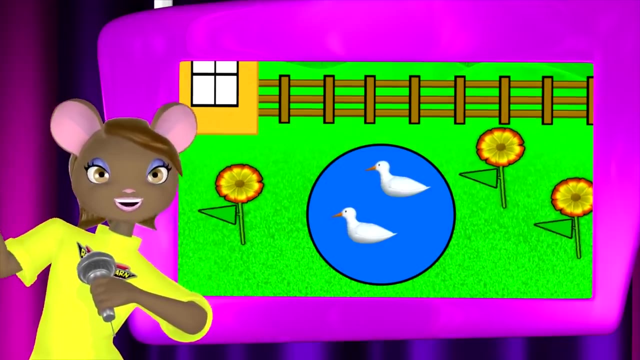 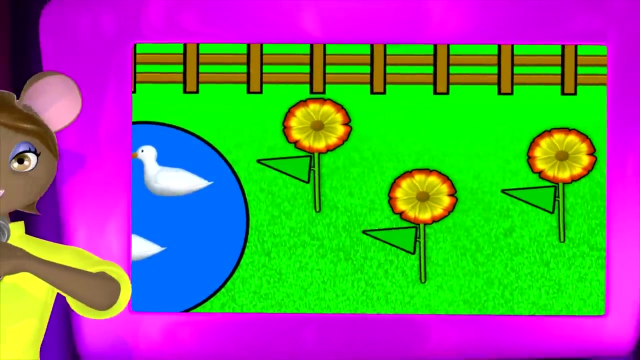 The door is a rectangle. I see a blue pond where the ducks like to swim. I see a blue pond where the ducks like to swim. Can you name that shape before we sing again? The pond is a circle. I see a green leaf growing on a flower. 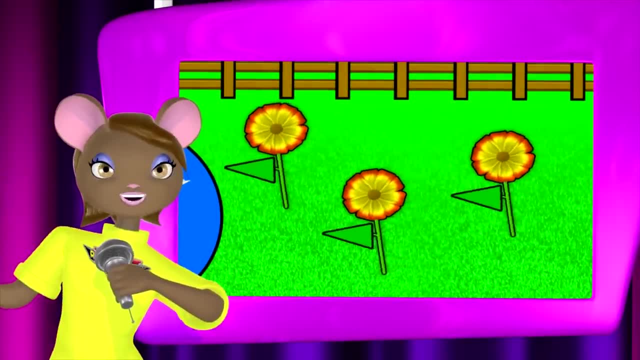 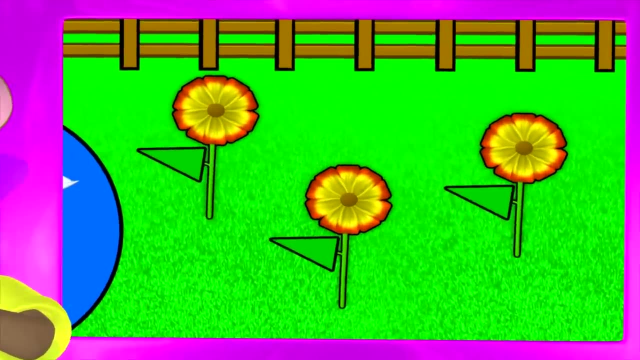 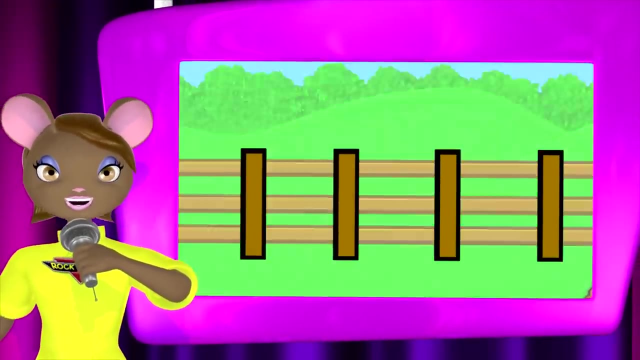 I see a green leaf growing on a flower- Can you name that shape? and stand tall like a tower. The leaf is a triangle. I see a brown post that's stuck in the ground. It's a part of a fence stuck in the ground. 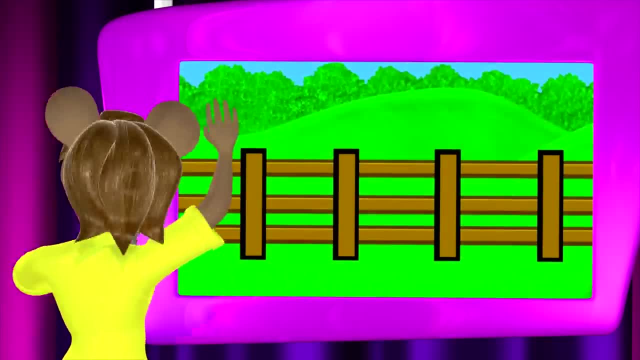 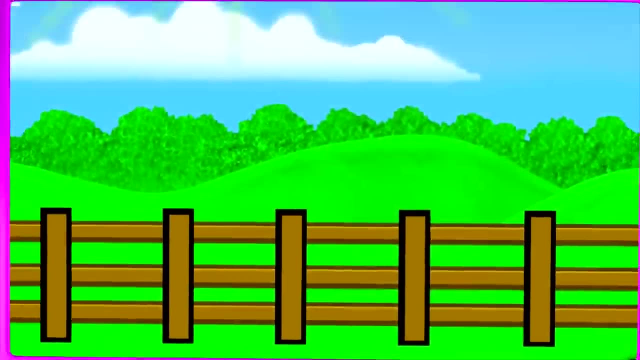 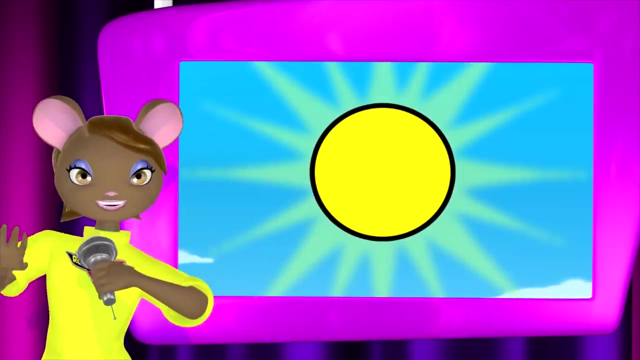 Can you name that shape? Stand up and spin around. The post is a rectangle. There's a yellow sun shining in the sky. There's a yellow sun way up in the sky. Can you name that shape? Then, wink your eye, The sun is a circle. 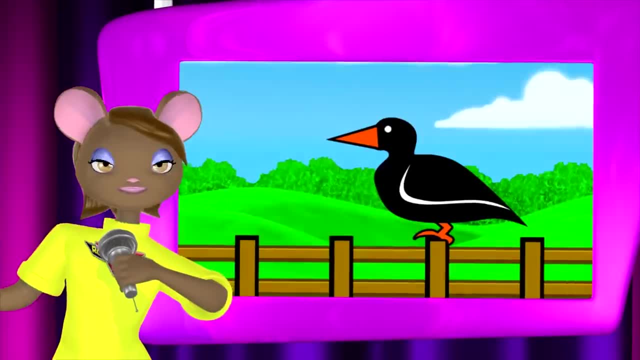 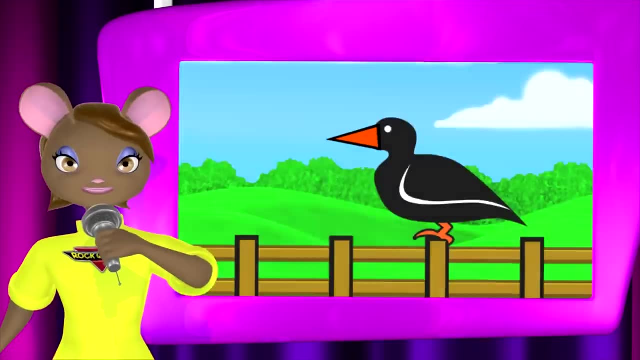 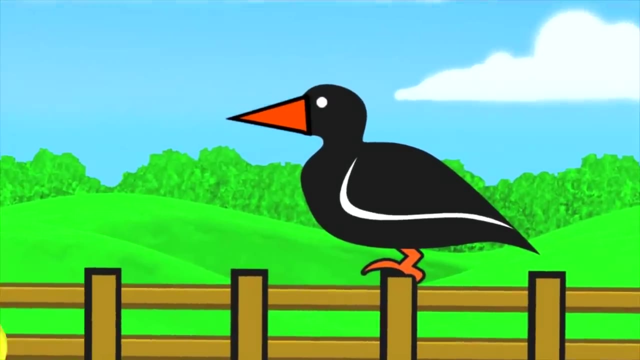 I see an orange bee on a bird that's black. I see an orange bee on a bird that's black. Can you name that shape before the ducks go quack? The beak is a triangle. I see a white window on the house, big and tall. 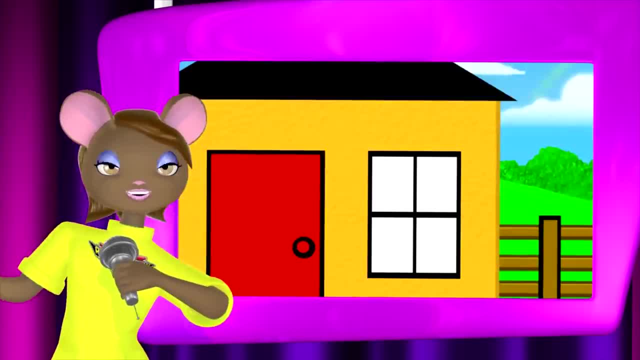 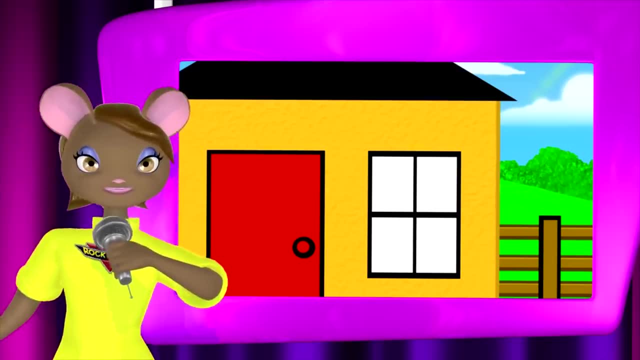 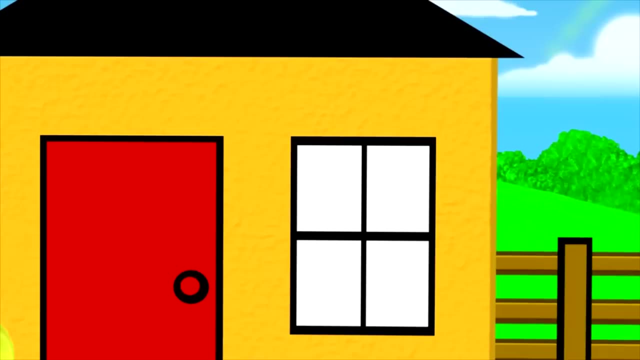 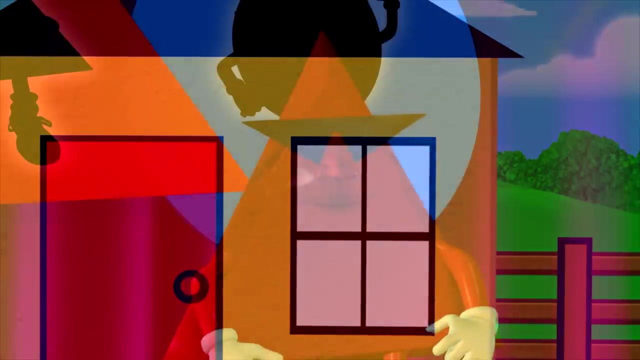 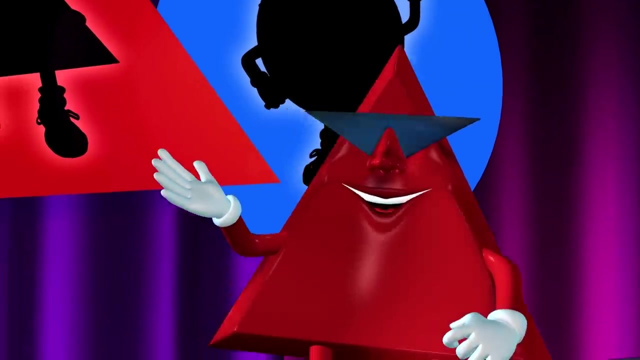 I see a white window on the house, big and tall- Can you name that shape? and stand straight as a wall. The window is a rectangle. The window is a rectangle. Well, I gotta split, But say hello to my good friend Rockford Rectangle. 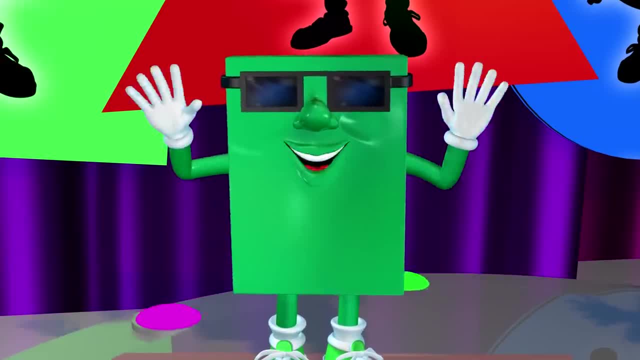 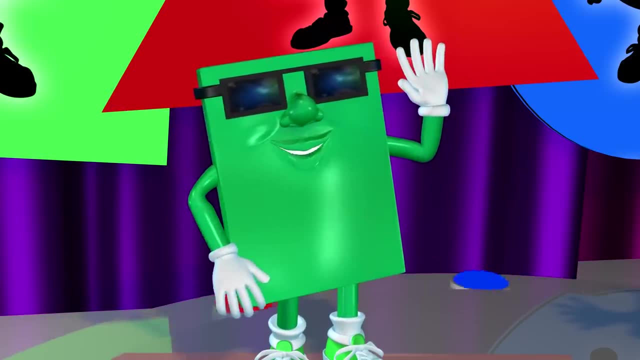 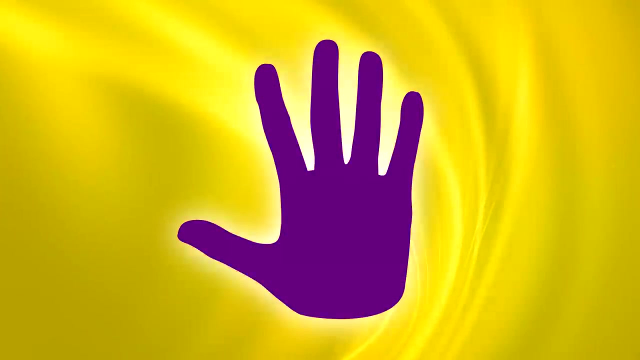 Thank you, Trolley. Pleased to meet you everyone. Now that you know about shapes and colors, let's try something new. Let's learn how to count. Hold up one of your hands and sing along. Music helps me count to five on just one hand. 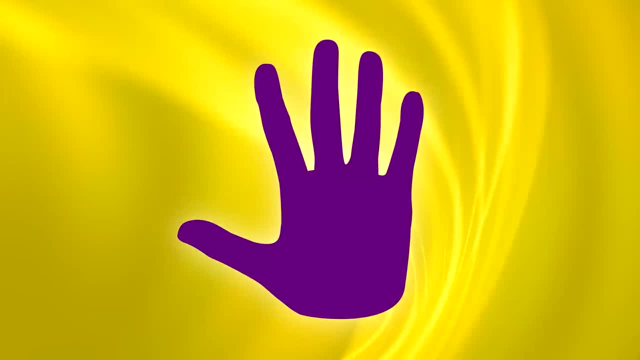 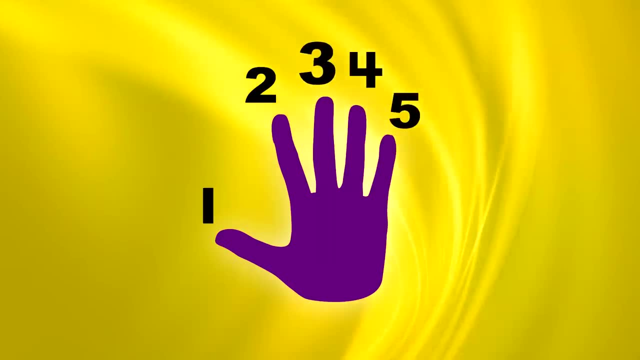 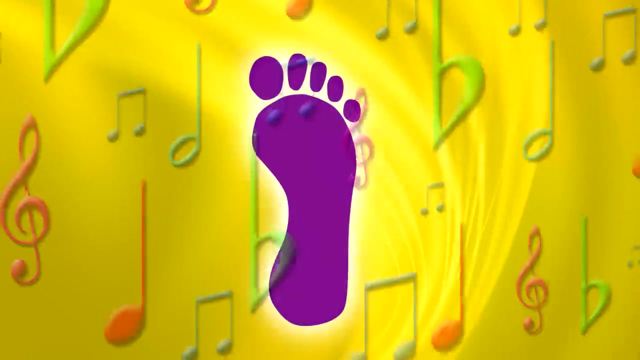 I can count my fingers and then do it again: One, two, three, four, five. Oh such good counting One, two, three, four, five. One, two, three, four, five. Music helps me count to five with one of my feet. 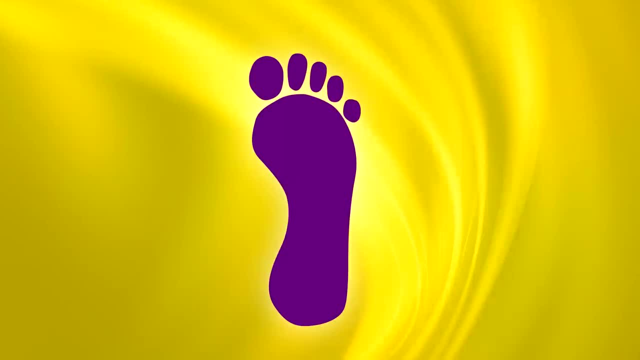 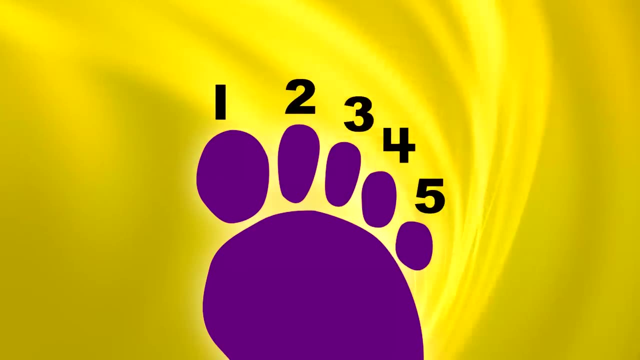 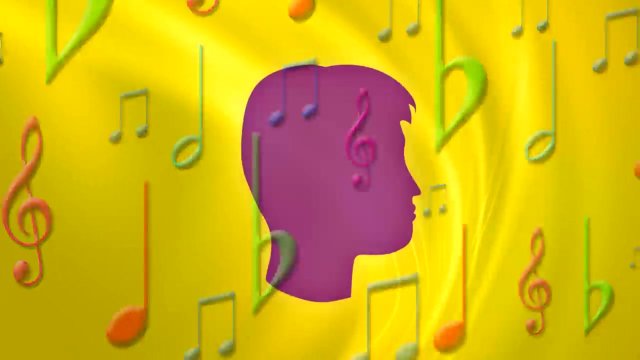 I can count my toes and keep the beat. One, two, three, four, five. Excellent. One, two, three, four, five. One, two, three, four, five. Music helps me count to five using just my mind. 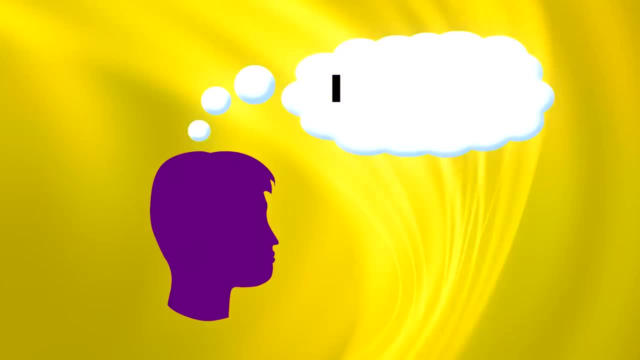 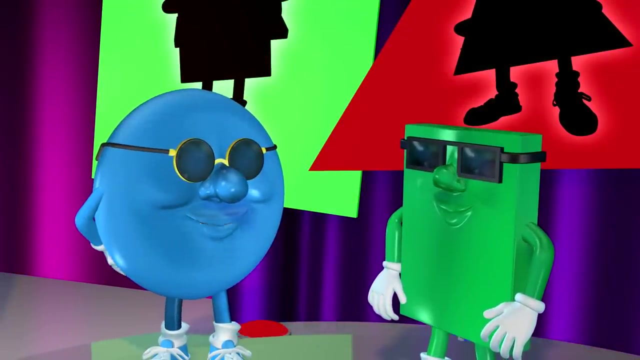 I can keep the rhythm and stay in time. One, two, three, four five. That's the spirit. One, two, three, four five. One, two, three, four five. What if I put my hands behind my back? 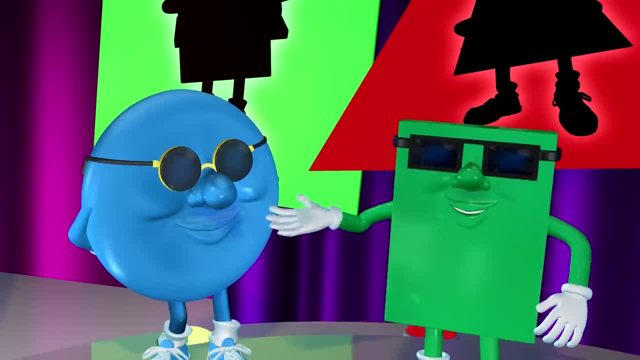 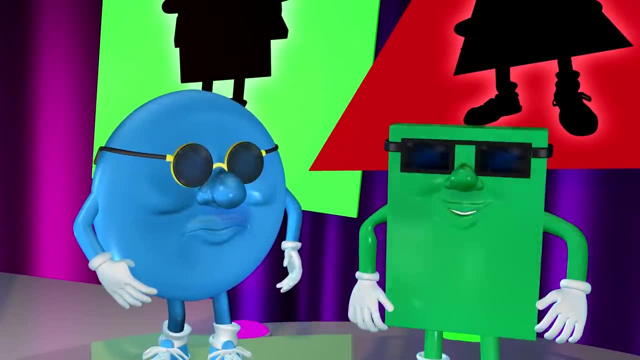 How many fingers can you count then? My good friend, you can't count any fingers. Oh no, What are we going to do now? Do calm down. We can say: we see zero fingers. Zero, That's right, Zero. 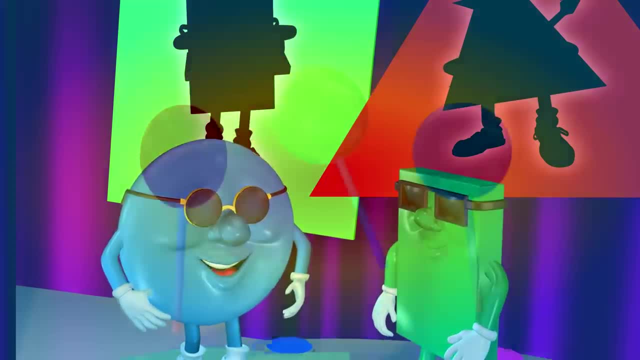 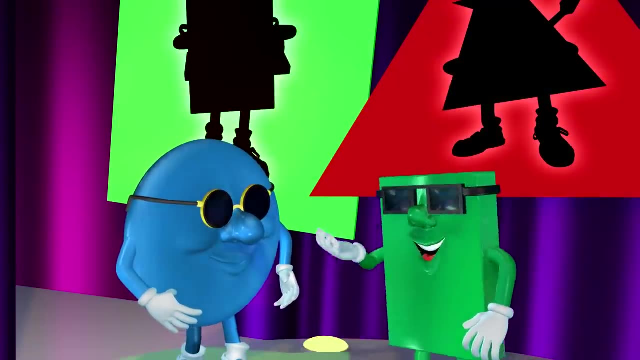 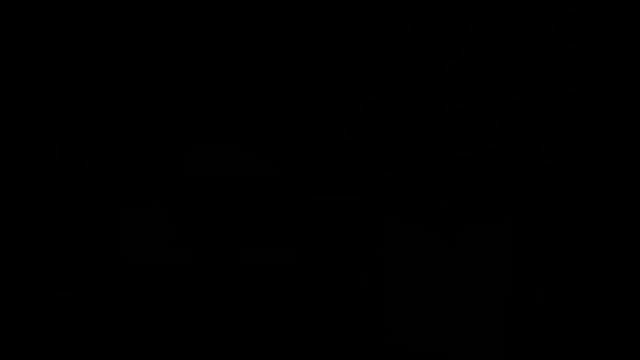 Zero means the same thing as none. Oh, so when I don't have any lollipops, I have zero lollipops. That is correct, Bummer Indeed. Hey Raleigh. what happens when colors get mixed together? 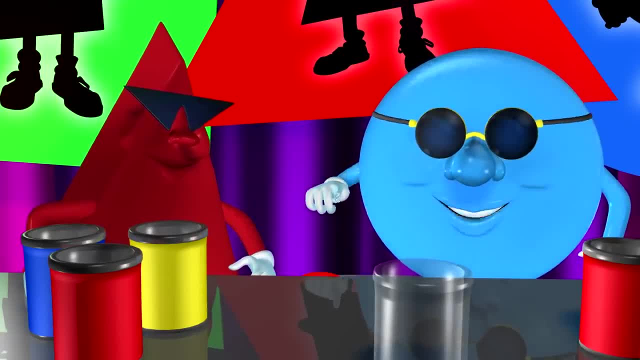 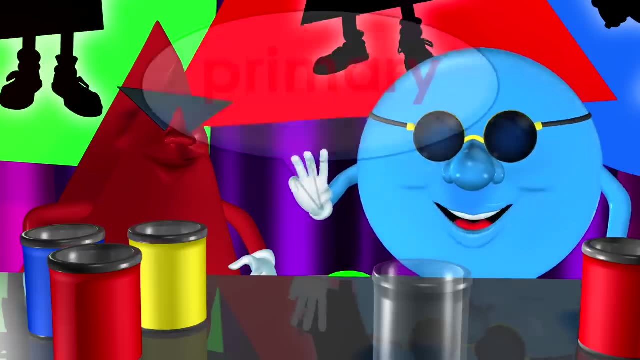 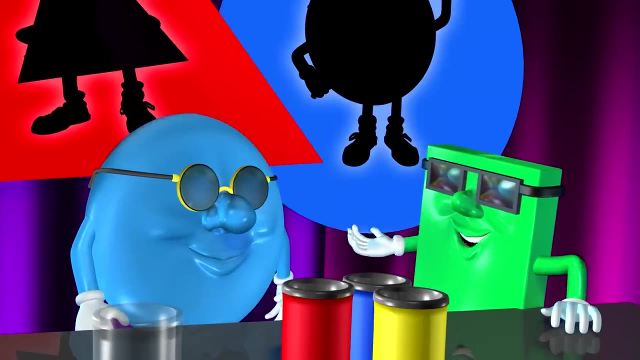 They make other colors. And did you know that with just three colors you can make lots of other colors? Those three colors are called primary colors. Excuse me, my good friend, But what are the primary colors? Red, yellow, blue. 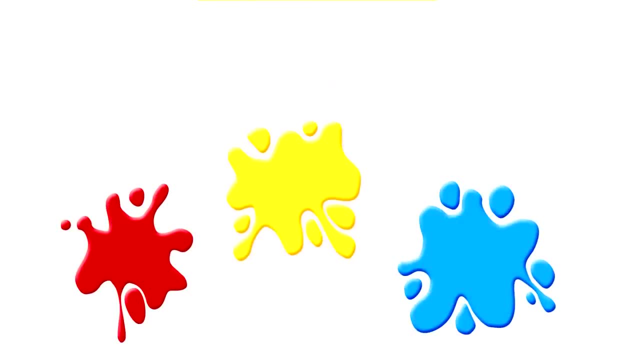 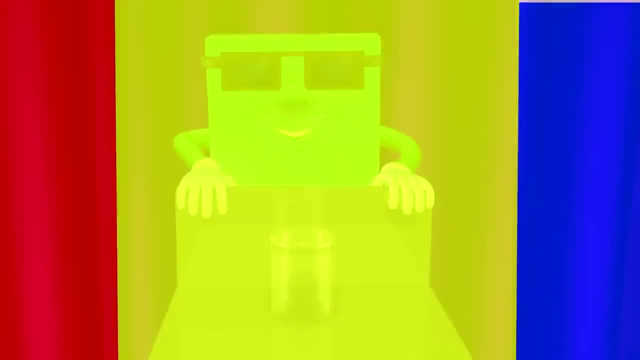 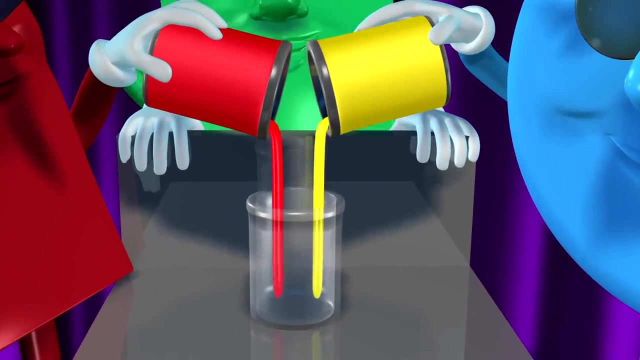 Red, yellow blue. With red, yellow blue. there's so much you can do. Oh goody, Let's mix red and yellow. Red and yellow mix together, make the color orange. Red and yellow mix together- make the color orange. 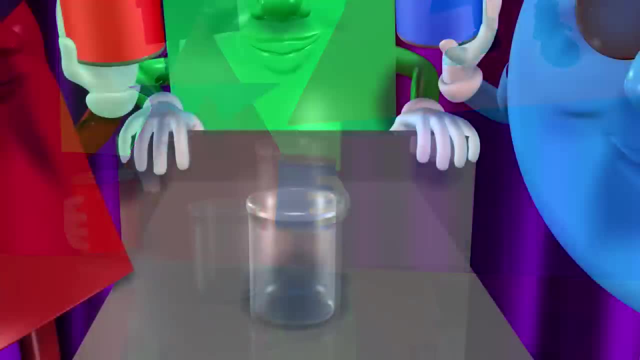 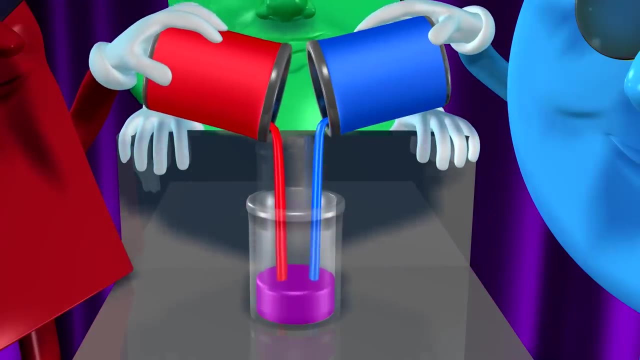 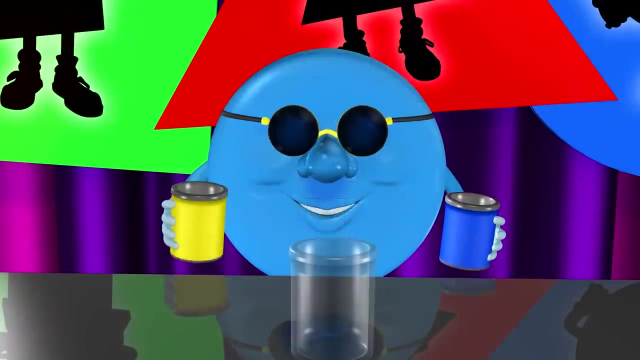 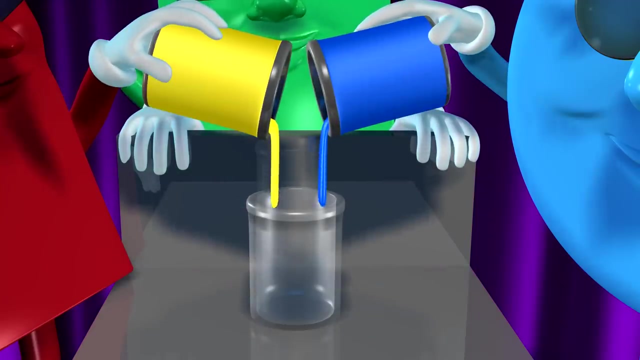 What about the blues man? Red and blue mix together make the color purple. Red and blue mix together make the color purple. Red and blue mix together, make the color purple. And don't forget yellow and blue. Yellow and blue mix together: make the color green. 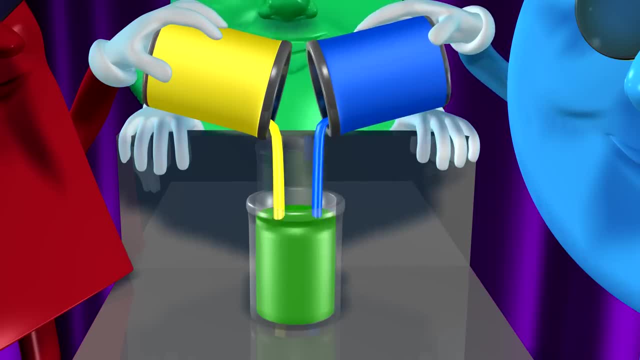 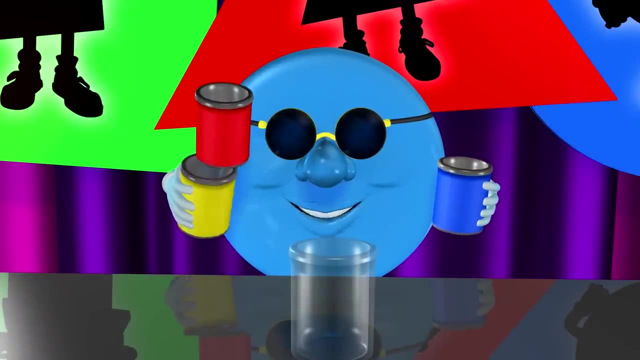 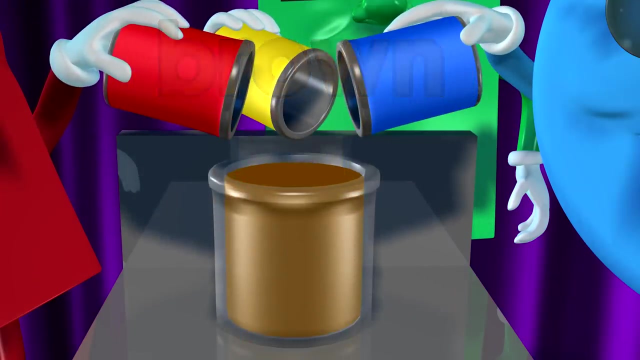 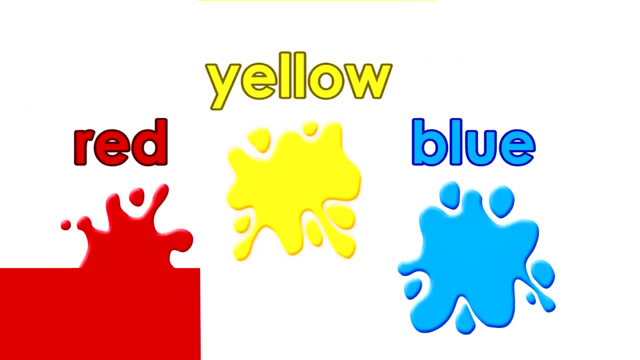 Yellow and blue mix together, make the color green. And if I mix all three together, what color will be found? Red, yellow and blue together make the color brown, Red, yellow, blue, Red, yellow, blue With red, yellow blue. 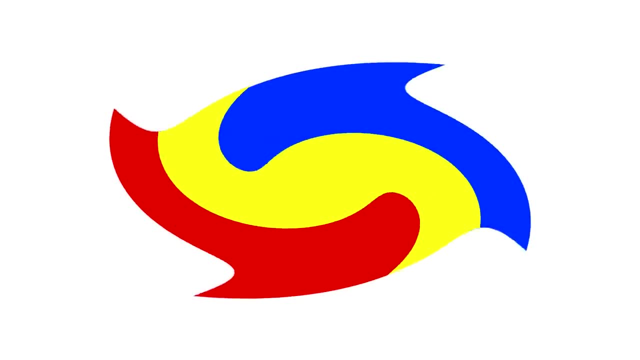 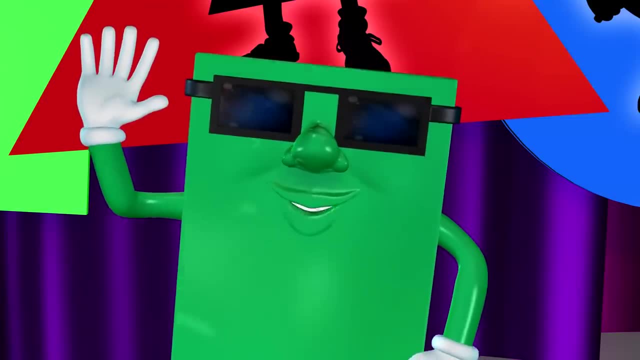 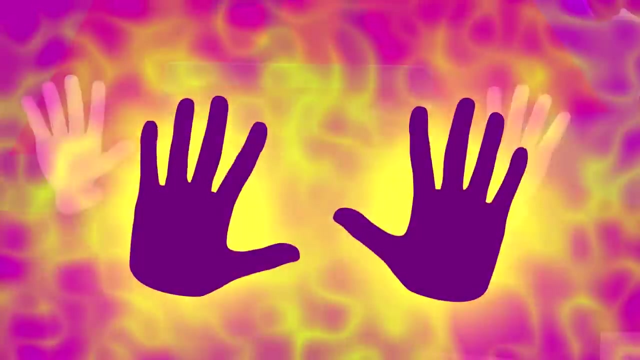 there's so much you can do. I know that you can count up to five and you're doing a wonderful job. Now let's see if we can go up to ten. This time we will use both of our hands Ready: One, two, three, four, five, six, seven, eight, nine, ten. 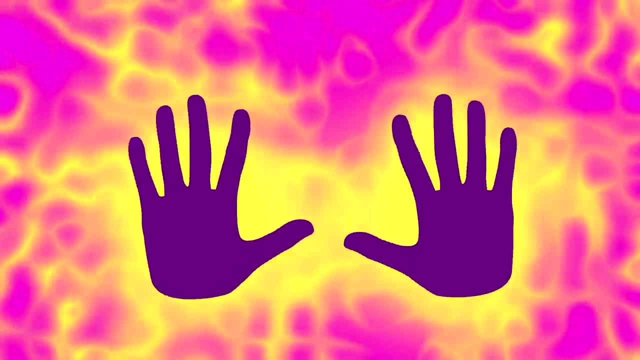 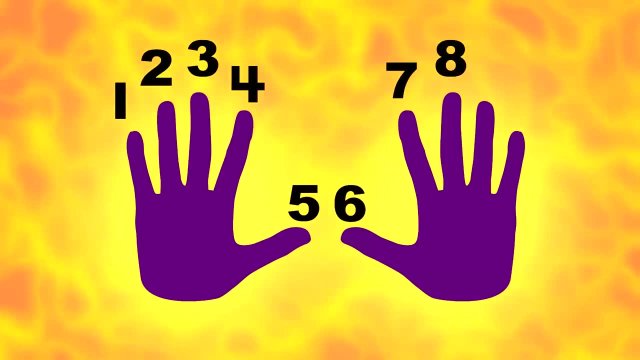 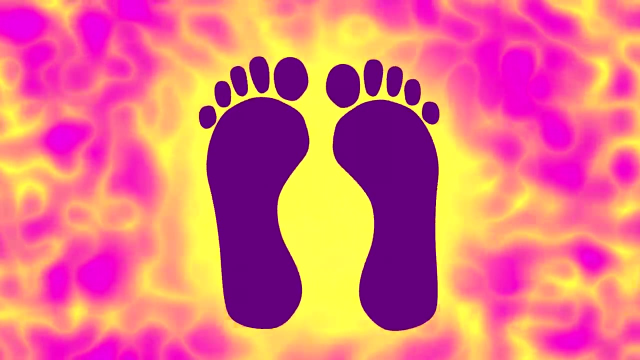 Then stop and count your fingers, and then we'll move our feet. One, two, three, four, five, six, seven, eight, nine, ten. I can dance to the rhythm. I can sing to the beat. Let's learn to count by singing. 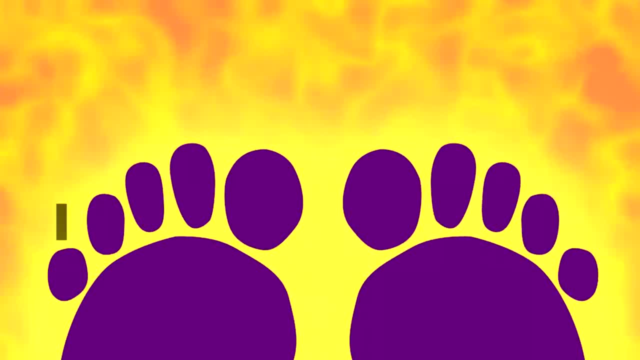 and count toes on our feet: One, two, three, four, five, six, seven, eight, nine, ten, 1,, 2,, 3,, 4,, 5,, 6,, 7,, 8,, 9, 10. 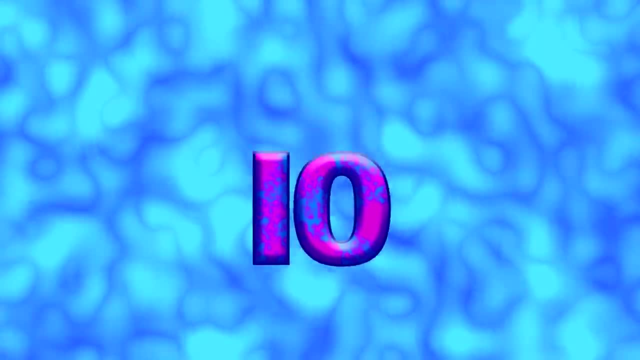 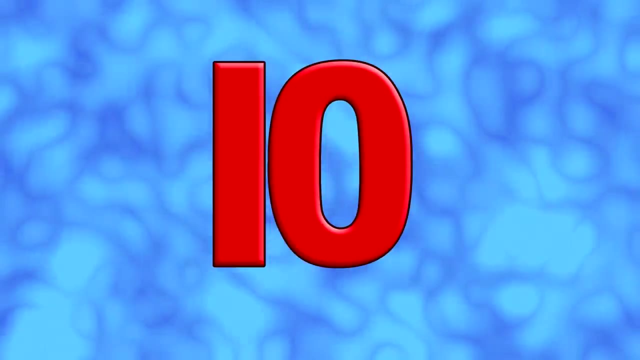 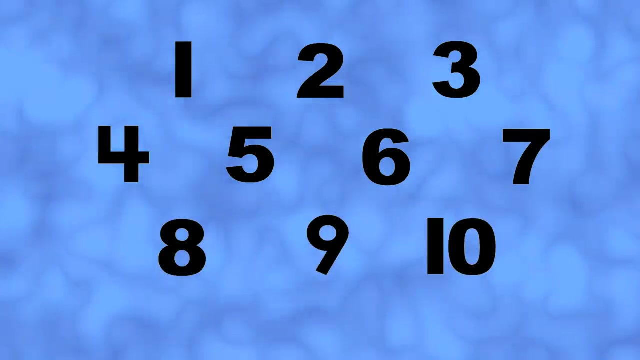 Counting up to ten Is not that hard, my friend, So count along with me. It's easy as can be. 1, 2, 3, 4, 5, 6, 7,, 8,, 9,, 10. 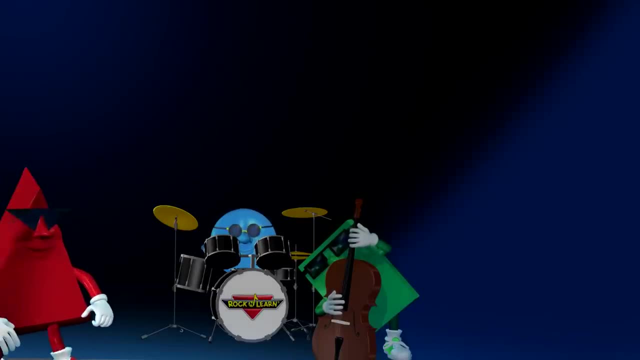 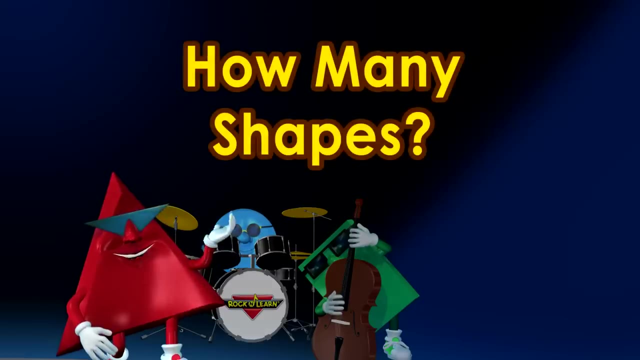 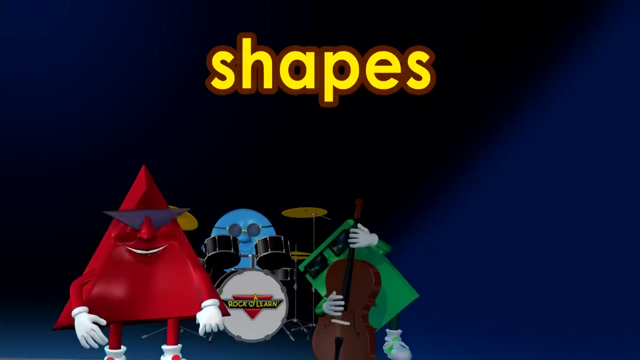 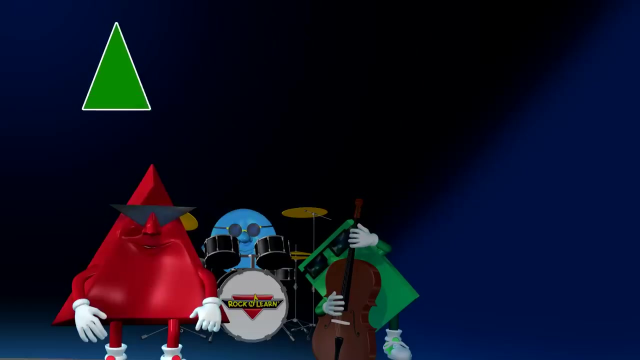 I have a fun game for us to play, Called How Many Shapes. Here's how to play. First, listen for the colors and the shapes in the song, Then count them. Can you say how many there are before I do? Here we go. How many green triangles do you see? 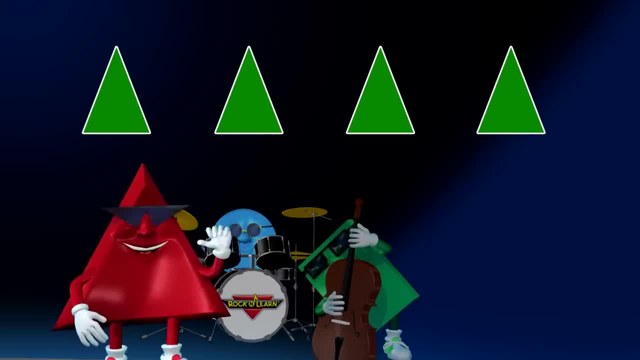 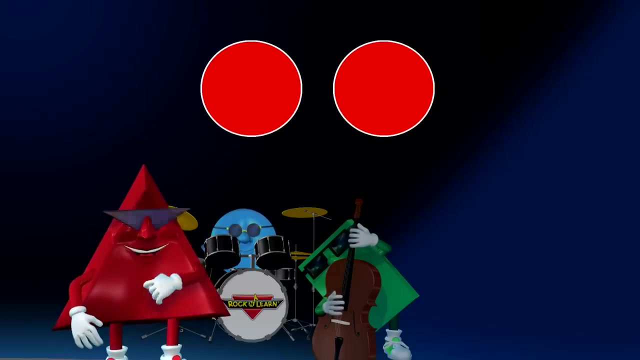 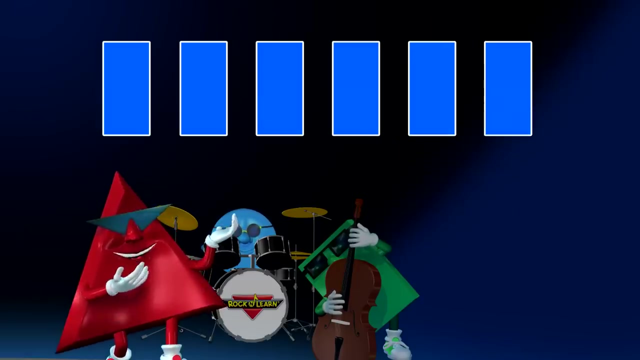 You'd better count quickly if you want to beat me. 4,, 4 green triangles. How many red circles are sitting in a row? Count them fast and let me know. 2,, 2 red circles. How many blue rectangles Are standing straight and tall? 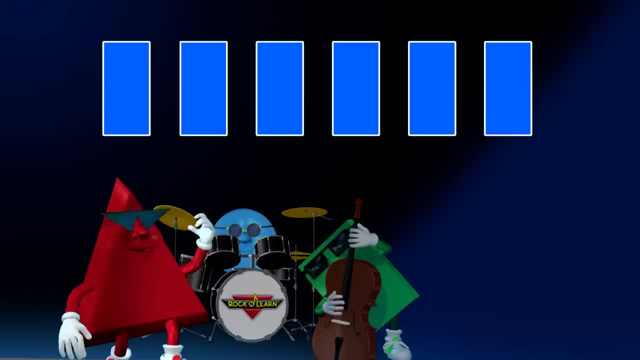 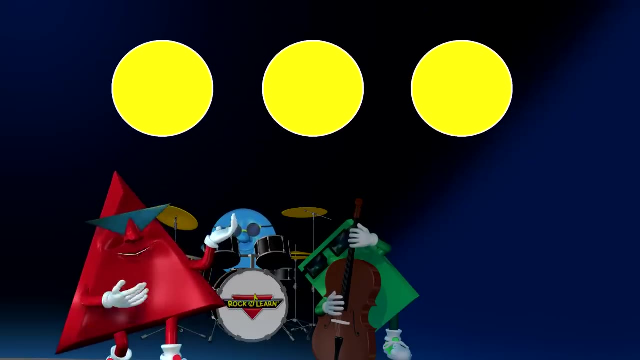 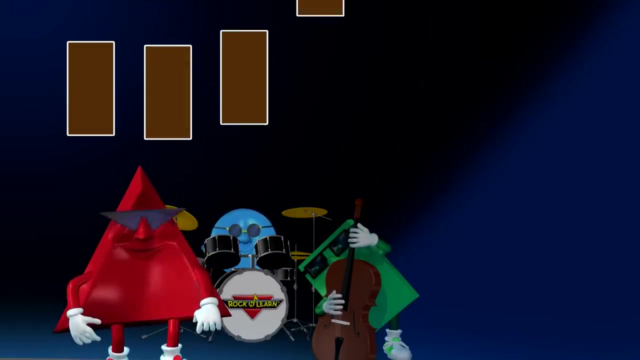 Count them and tell me The number that you saw. 6, 6 blue rectangles. How many yellow circles do you see? You'd better count quickly if you want to beat me. 3, 3 yellow circles. How many brown rectangles Are standing straight and tall? 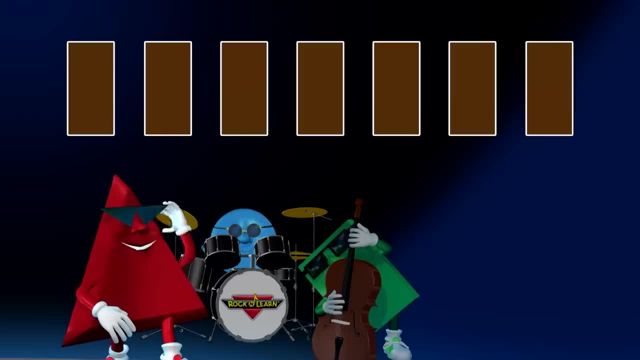 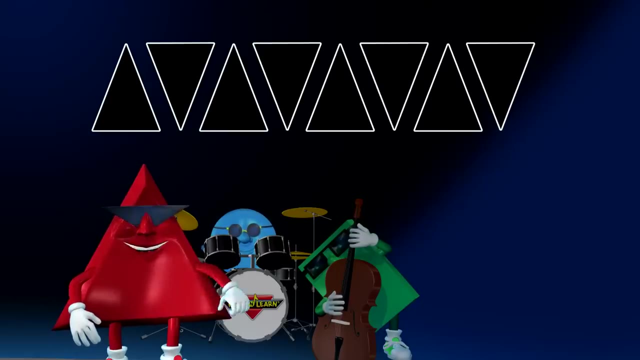 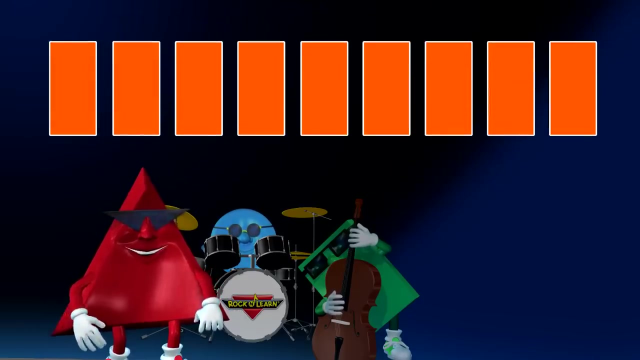 Count them and tell me The number that you saw: 7, 7 brown rectangles. How many black triangles Are sitting in a row? Count them fast and let me know: 8, 8 black triangles. How many orange rectangles Are standing straight and tall? 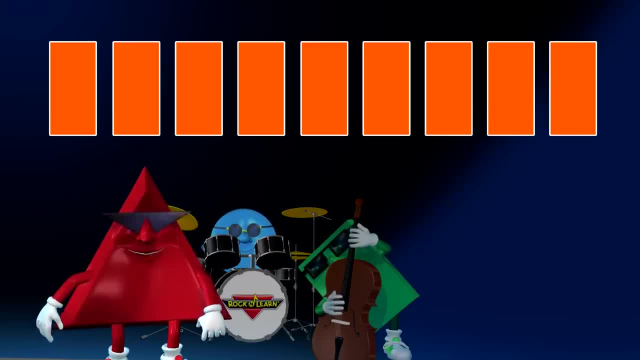 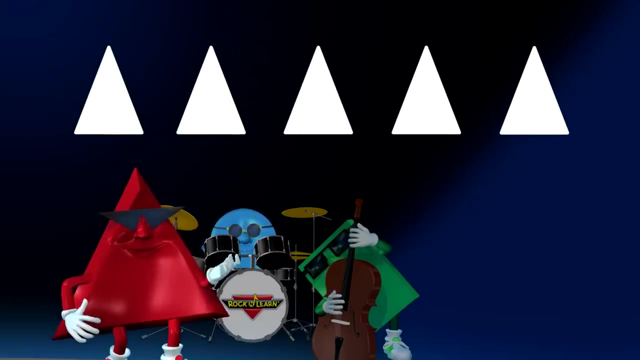 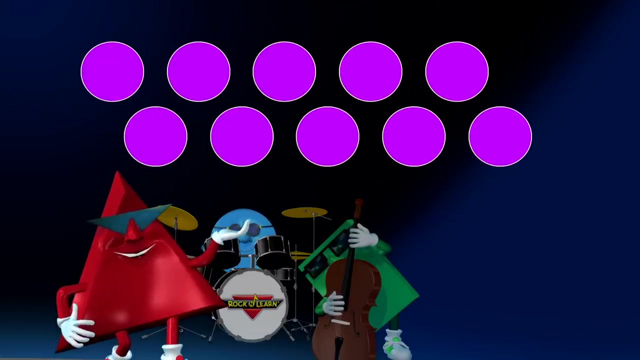 Count them and tell me The number that you saw. 9, 9 orange rectangles. How many white triangles Are sitting in a row? Count them fast and let me know. 5, 5 white triangles. How many purple circles do you see? You'd better count quickly if you want to beat me. 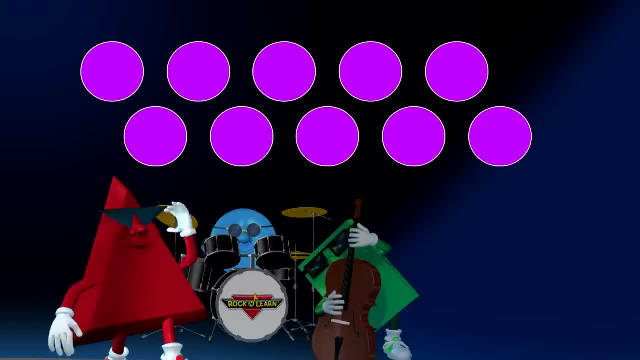 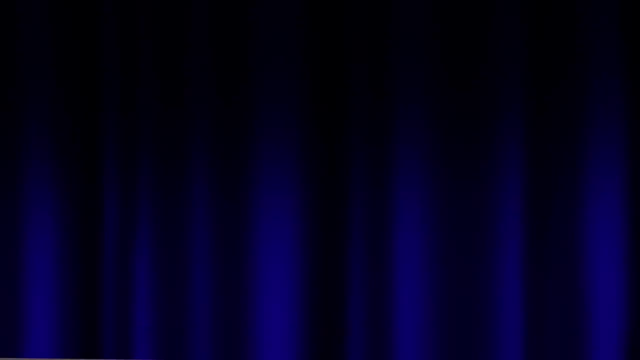 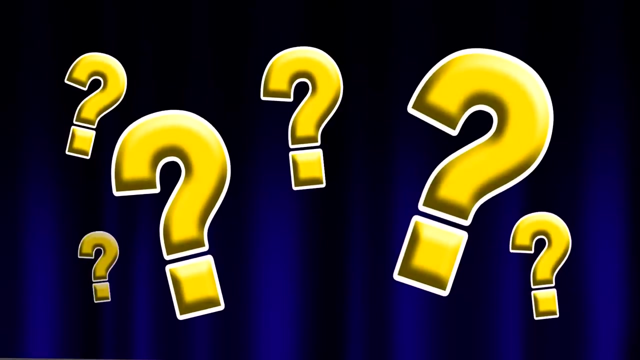 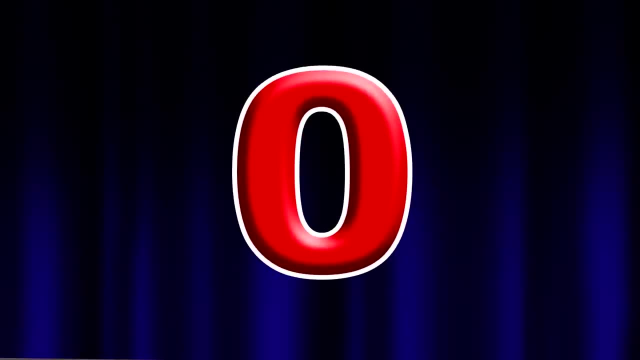 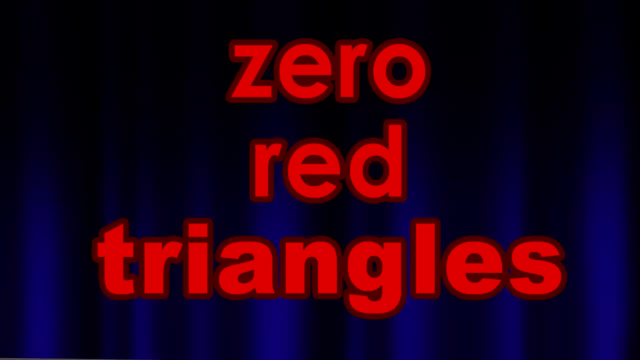 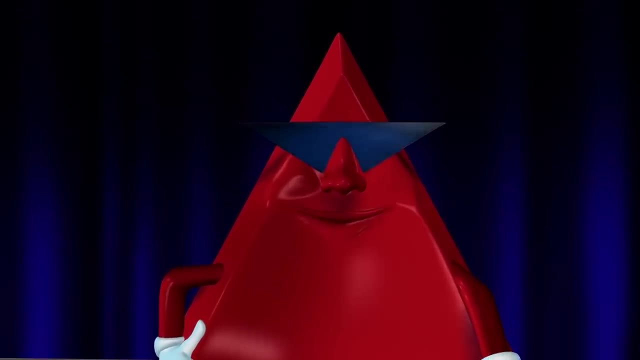 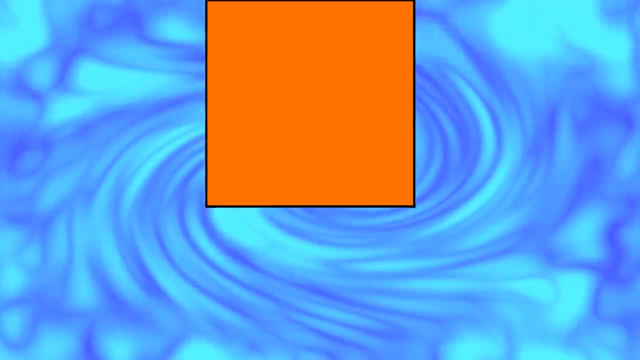 I don't see any red triangles. That means we have zero red triangles, Zero red triangles. Zoe, Not only have you learned some really neat colors and shapes, You can even count to ten. Let's learn some more shapes. There are so many shapes, It's plain to see. 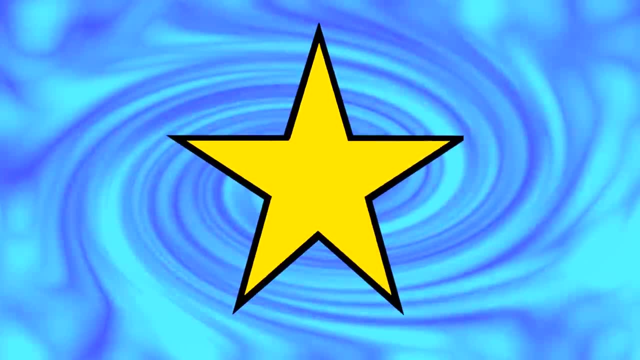 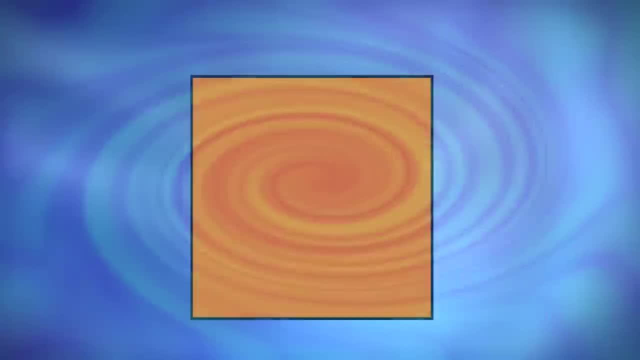 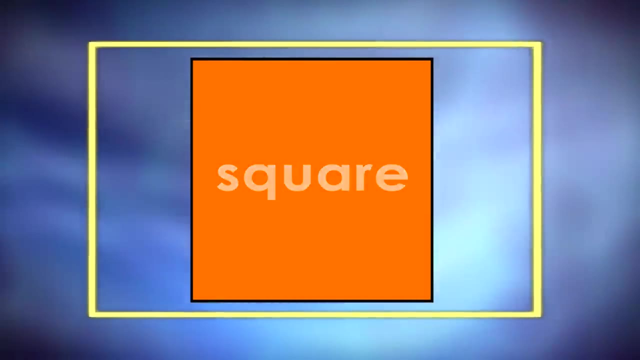 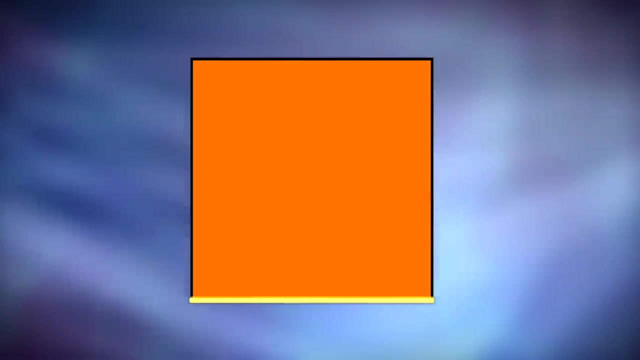 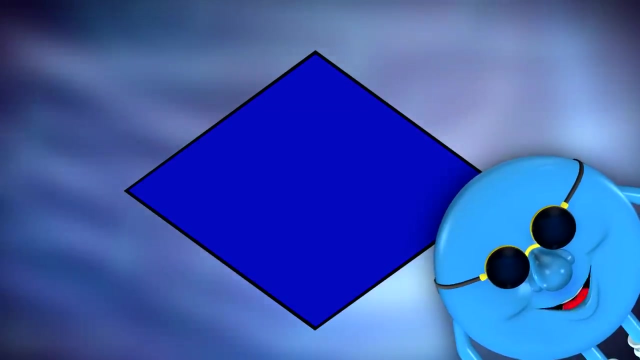 Ooh, ooh, ooh. If you want to learn some more, Then sing with me. Yeah, Look at the orange shape. A square is a special rectangle. Yes, it's true, All four sides are the same length. Now we've learned something new. Look at the orange shape. 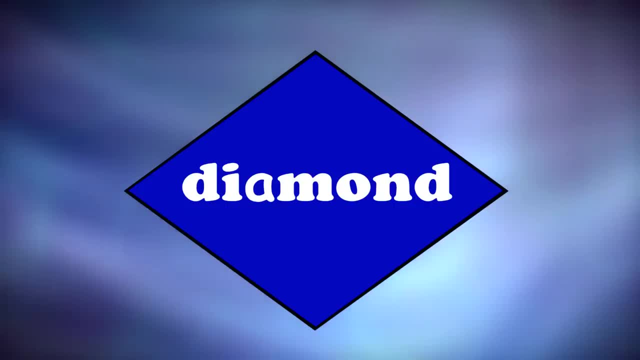 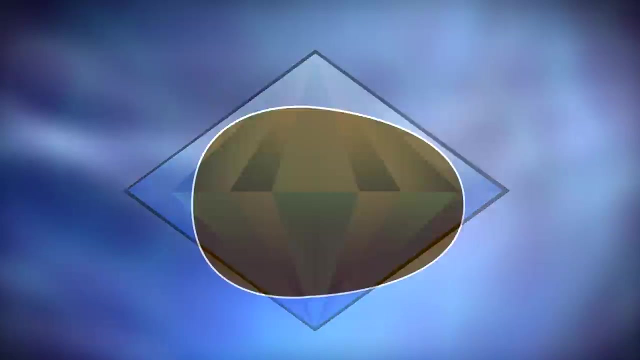 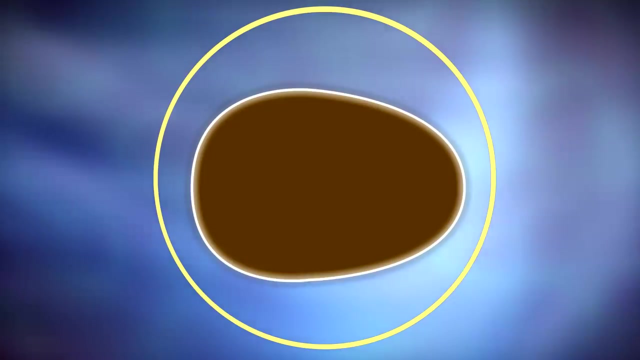 And the blue shape. A diamond has four sides, But that's not the only key. It's not a square or a rectangle, It's something else you'll see. Look at the brown shape: An oval is like a circle That has been squashed down. Wow, It has been squashed down. 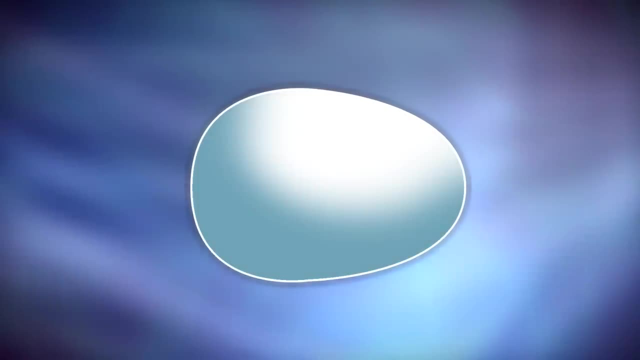 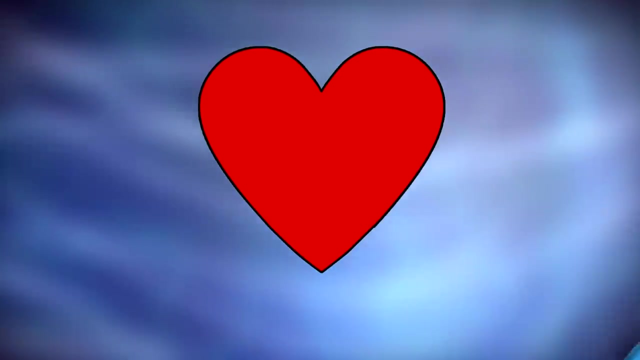 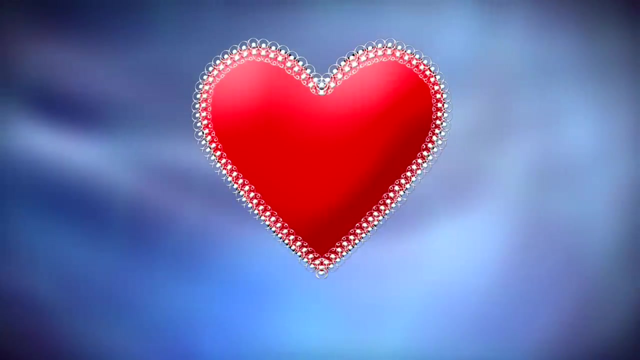 It can look like an egg If it's colored white or brown. Look at the red shape. A heart is what you see On a special Valentine And I'll color one red for you If you promise to be mine. Look at the white shape, And a heart is what you see. 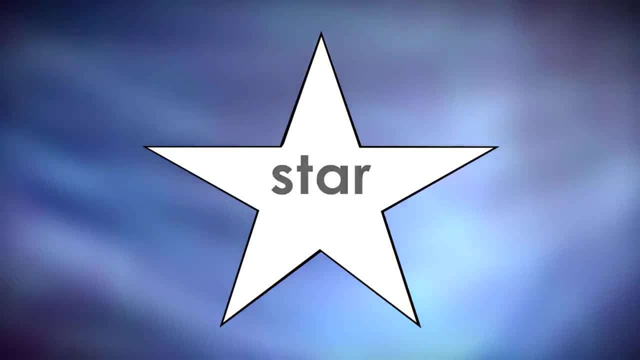 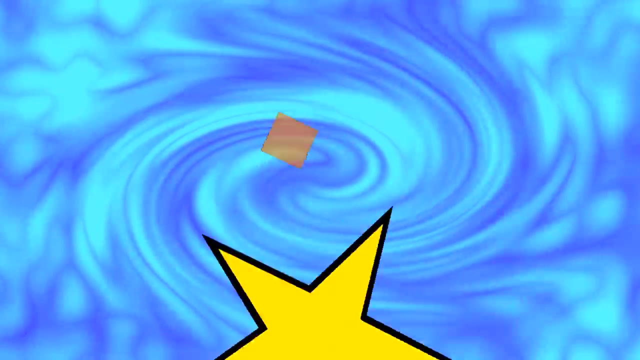 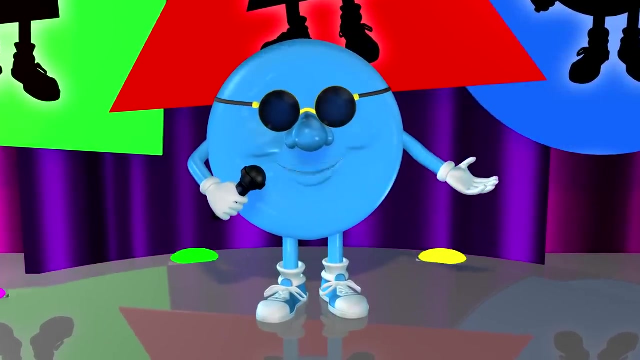 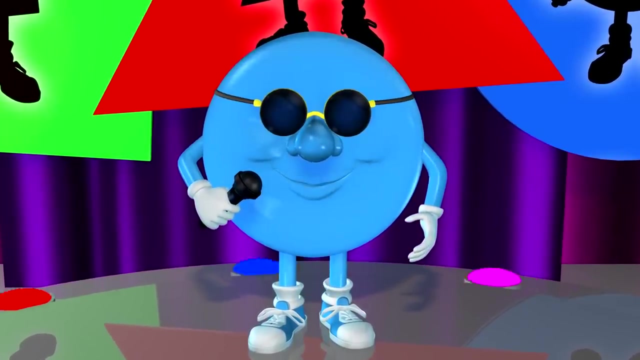 Stars have five points On the flag of the USA. I know you can find some more Almost any day. Yeah, I am impressed. You have learned about some unusual shapes. Now we'll learn some more colors. There are so many colors in the world to see. 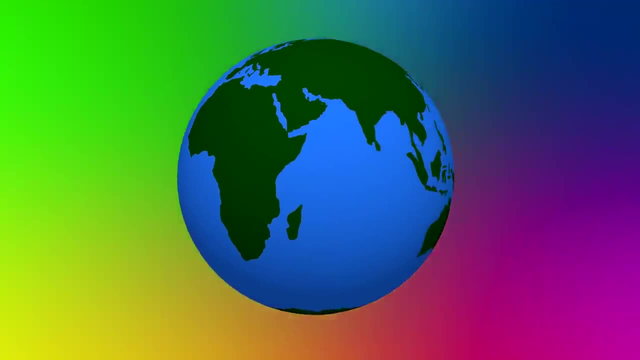 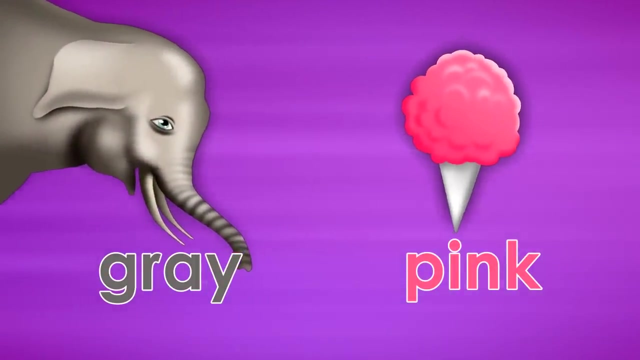 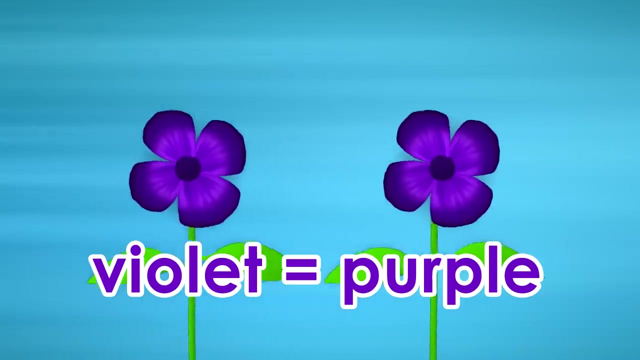 Let's learn a few more color names, Just you and me: Gray as an elephant And pink as cotton candy. I'm learning more colors And I think that's pretty dandy. Violet's the same as purple. Yes, I know that it's pretty dandy. 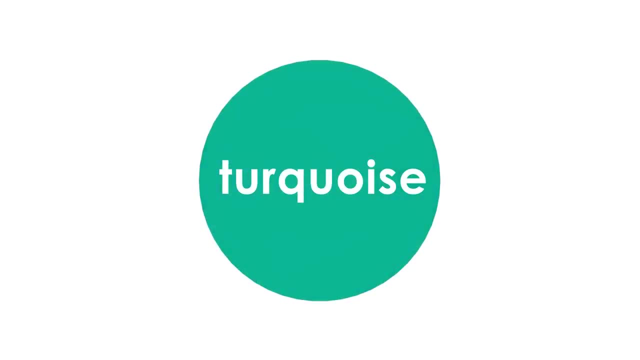 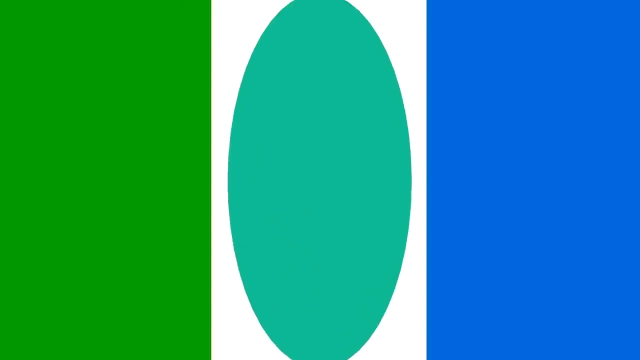 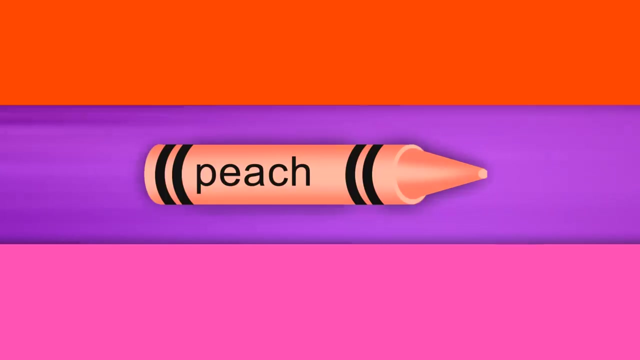 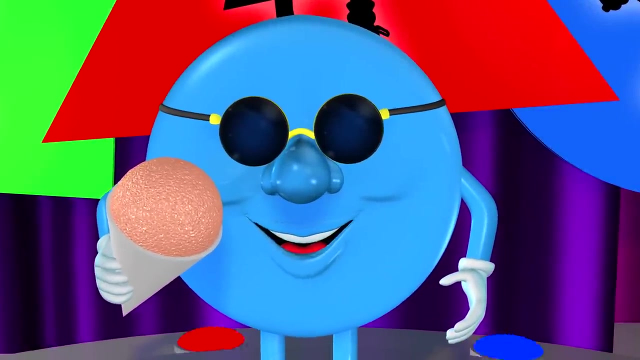 But it is true. And the color of turquoise Is between green and blue. Peach is a color between orange and pink. Just use a peach crayon And tell me what you think. I think I'll have a peach snow cone Maroon is a color that's a deep 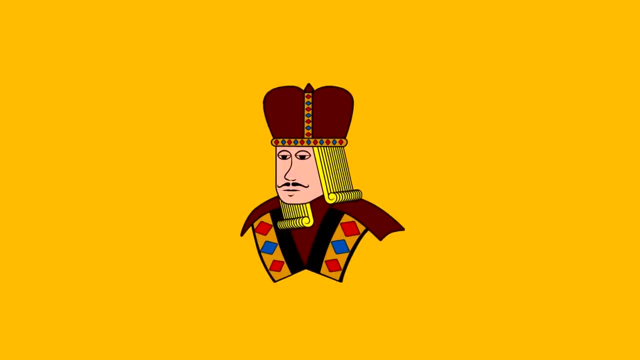 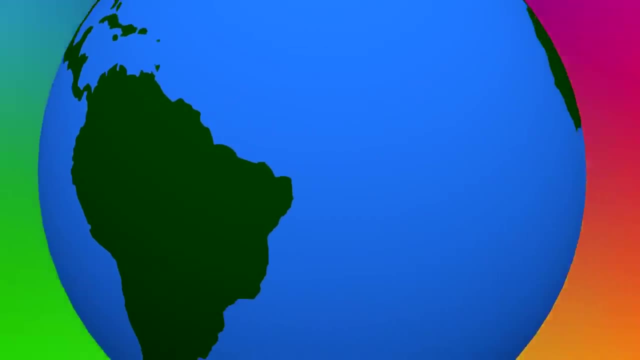 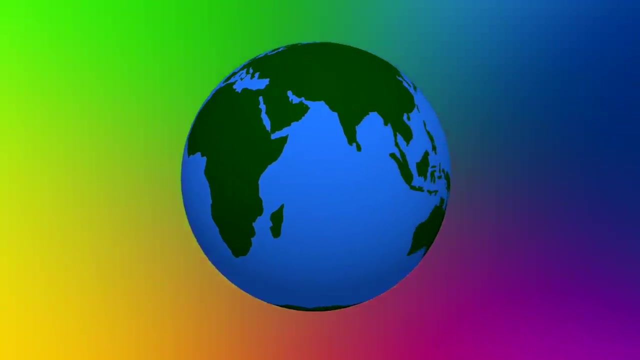 I think I'll have a peach snow cone. Brown is red. It looks just like a color A king might wear upon his head. Yes, there are so many colors In the world to see. We've learned a few more color names- Just you and me, Hey, everyone. 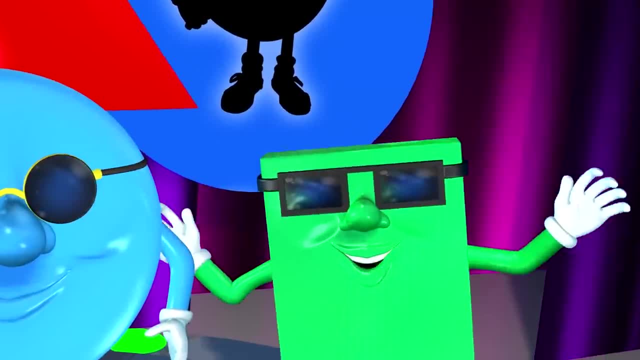 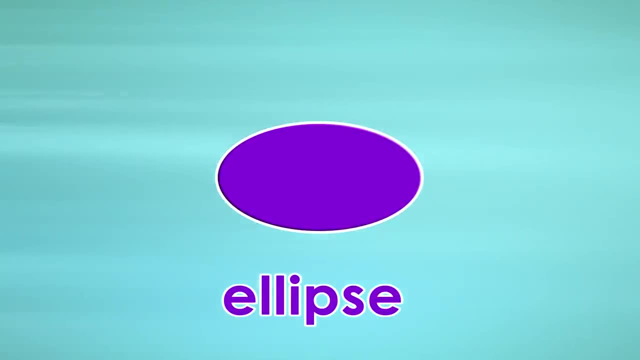 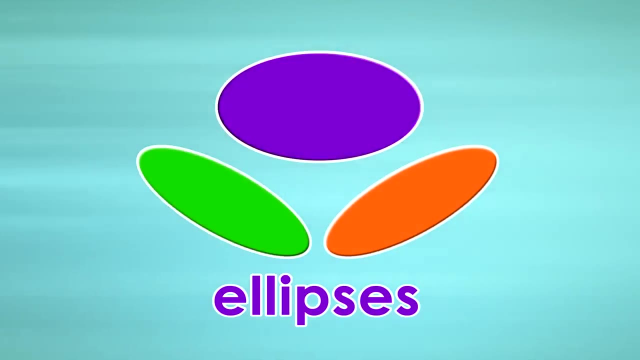 Let's learn about other shapes. All right, Oh goody, All right. The purple shape's called an ellipse. When you have more than one ellipse, You have some ellipses. The green and orange shapes Underneath the purple ellipse Are also ellipses. 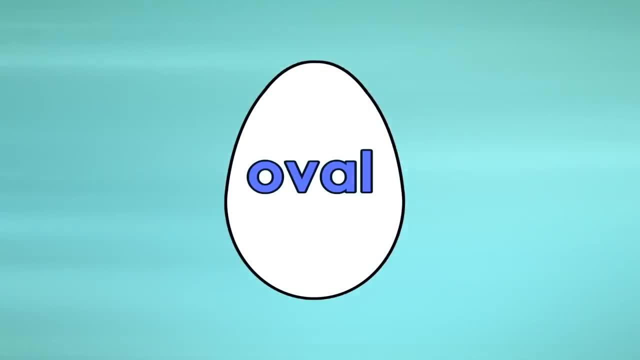 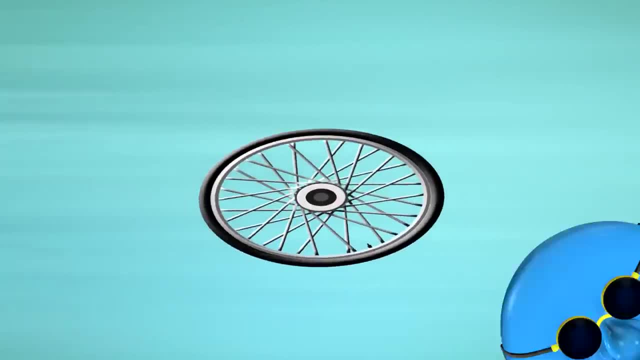 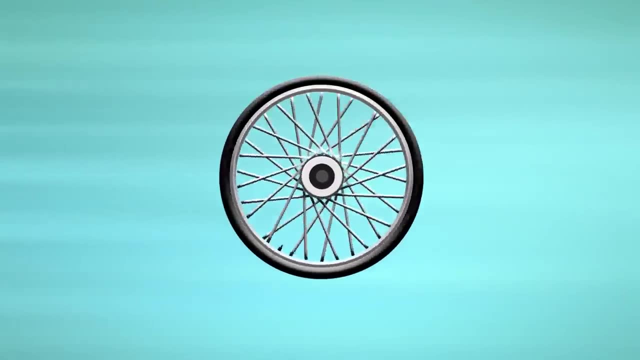 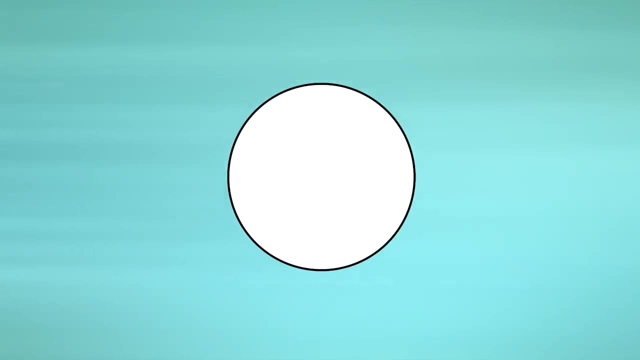 An ellipse is a special oval. An ellipse is a special oval. It's not like the wheel on a bike, Unless your bike's wheel is really broken. Ha ha, ha, ha, ha ha ha. A bicycle tire is shaped like a circle. Ha ha, I guess you could say: an ellipse is like a squished circle. 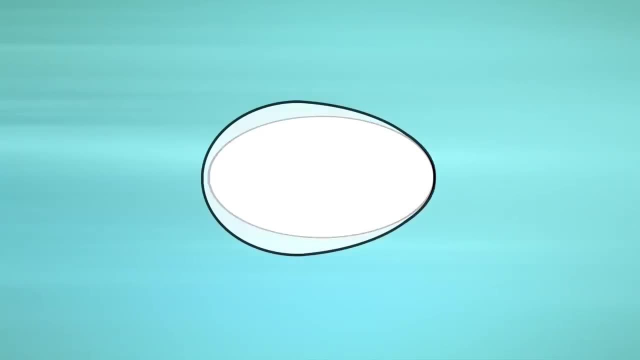 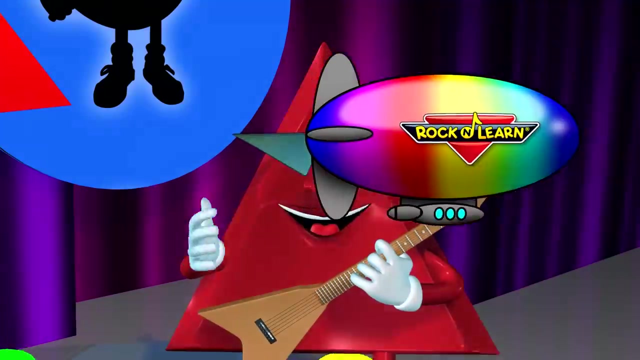 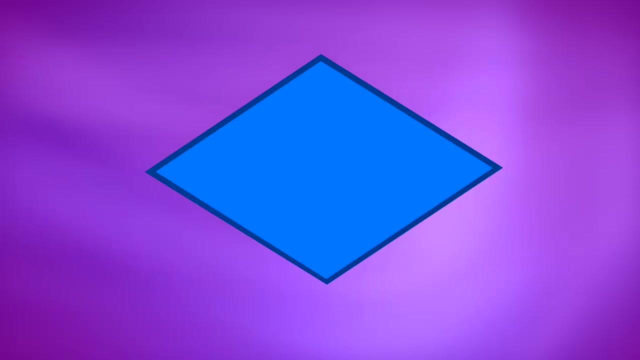 With both ends the same. Remember the shape you see on an egg is an oval. It is not an ellipse Because the two ends are different- different. Can you find other ellipse shapes and things around you? I know you can Look at the blue shape. Remember that shape is called a diamond. You can see the diamond. 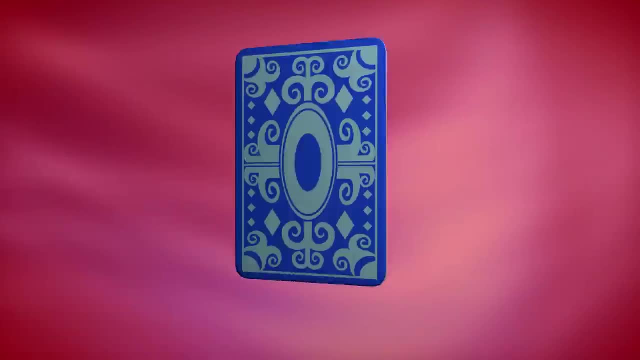 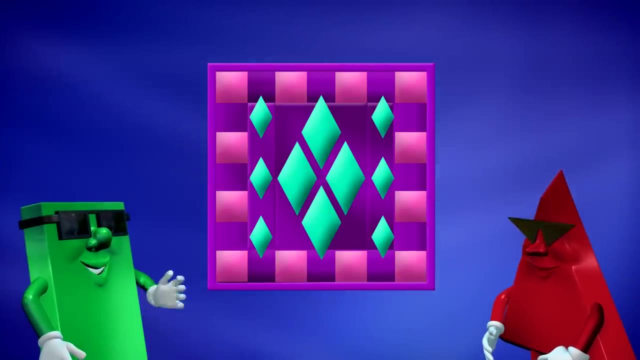 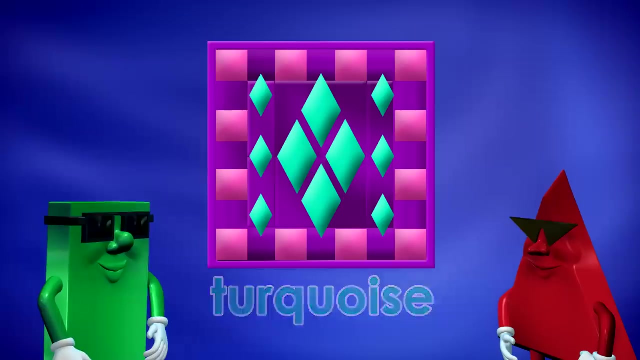 shape on some cards and you might see it with other shapes to make the patterns in a quilt. Pardon moi, Trolley, but what color are the diamonds? They're turquoise. Rockford, my man Cool. blue-green, But Trolley, my good triangle. what about those pink shapes? That's. 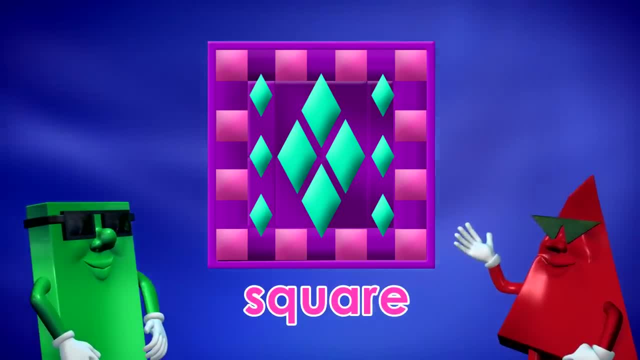 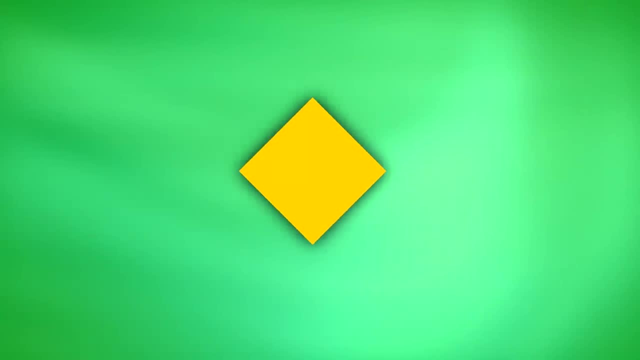 Squaresville man. The pink shapes are squares. A square is different from a diamond even when it is turned on its side. Oh, I see. So the red shape is a diamond Right and the yellow shape is a square turned halfway on its side. Yeah, 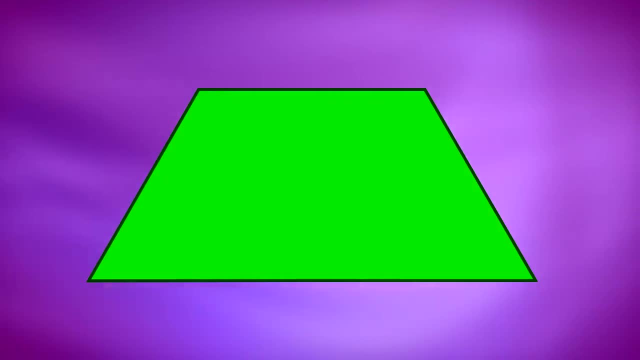 What is that funny-looking green shape? That shape is called a trapezoid. It has four sides, like a square and a diamond, but it is very different from a square or a diamond, or even a rectangle, Square, rectangle, square. 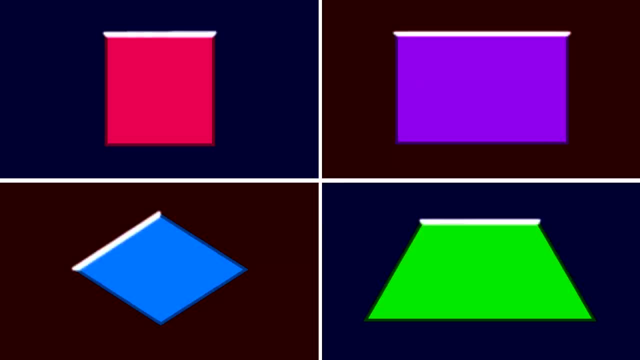 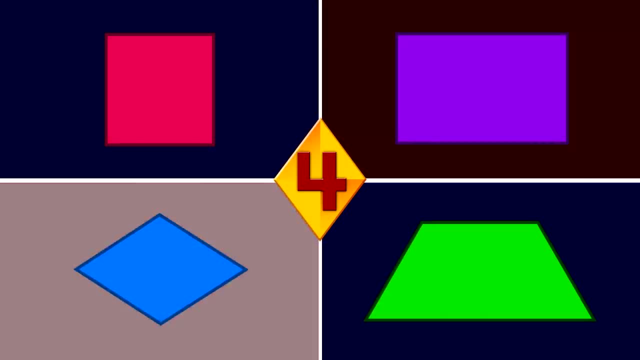 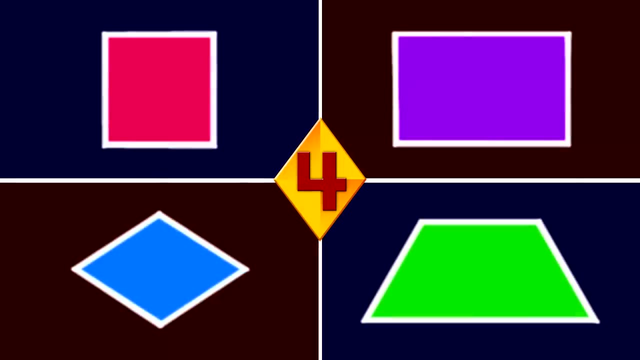 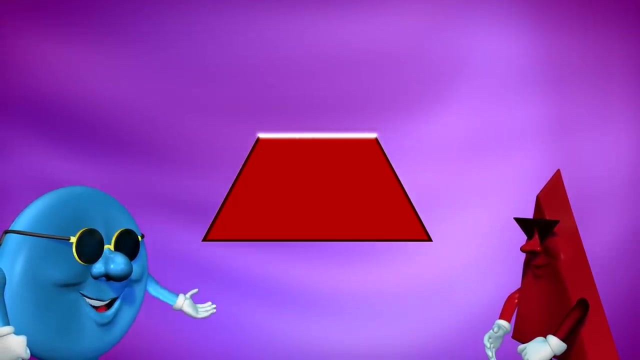 Diamond trapezoid. All these shapes have four sides. Square, rectangle, diamond trapezoid- Four cool shapes with four cool sides. Oh, I see A trapezoid is a shape with a long side and a short side across from each other, Kind of like a triangle with a top cut off. 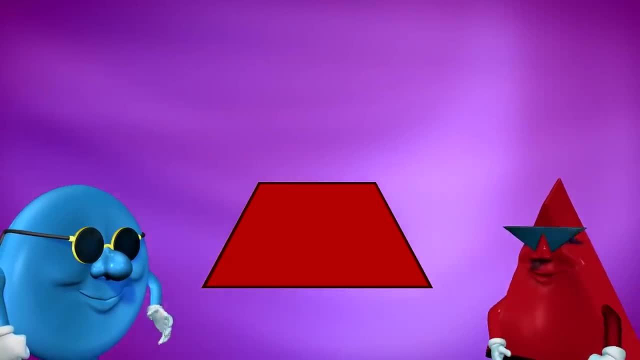 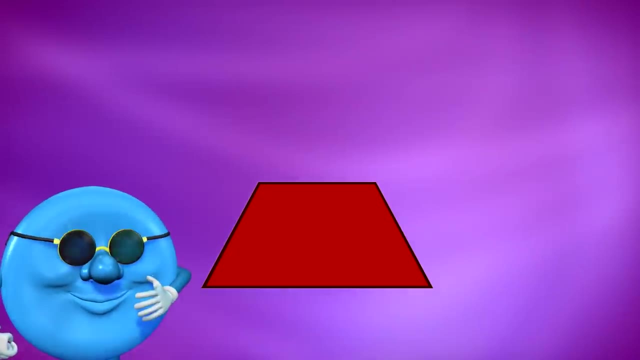 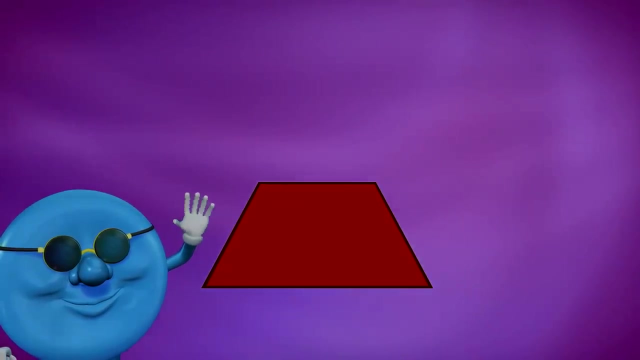 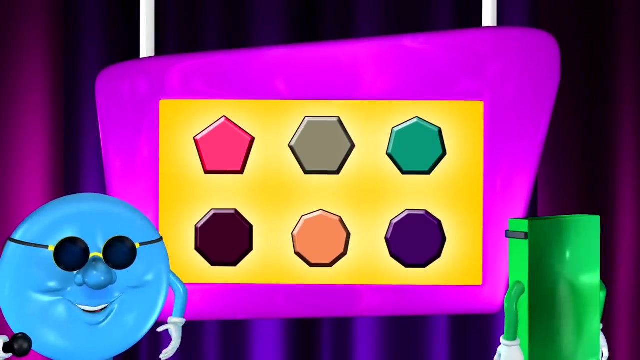 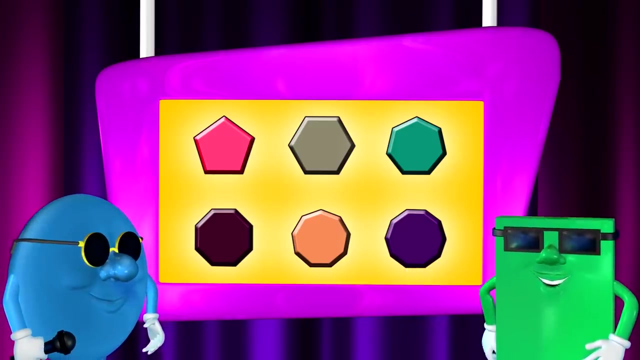 Cut off. ouch, that could hurt. don't worry, trolley, We would never do that to you. Wow, look at all the unusual shapes, and each shape has a different color, Indeed, and each shape has many sides to count. Point to the pink shape. Let's count the size. 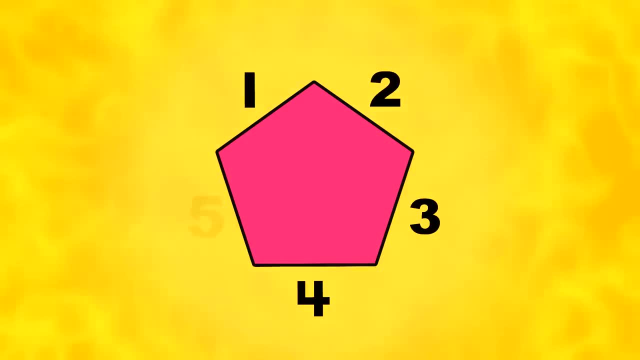 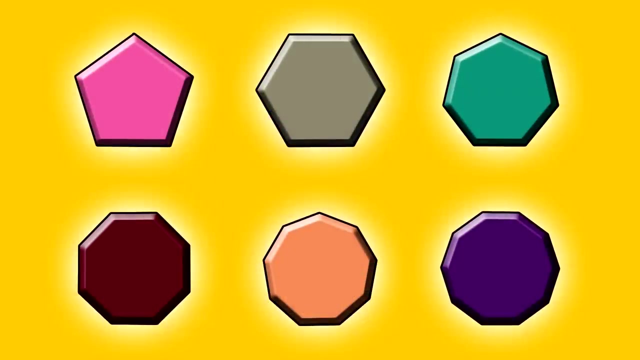 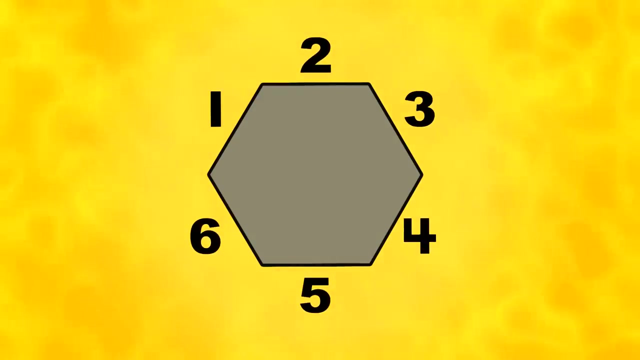 One, two, three, four, five. a shape with five sides is called a pentagon- Pentagon. Point to the gray shape. Let's count the size. one, two, three, four, five, six. a shape with six sides is called a hexagon- Hexagon. Point to the turquoise shape. let's count the size. 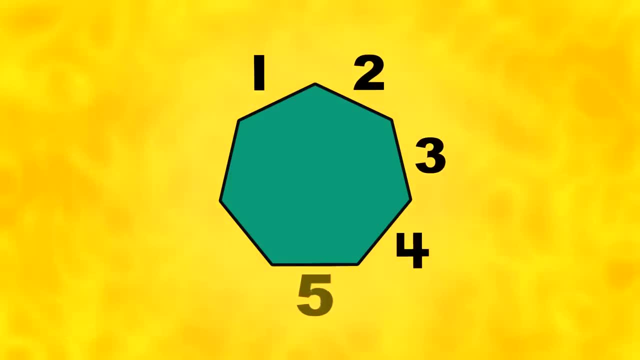 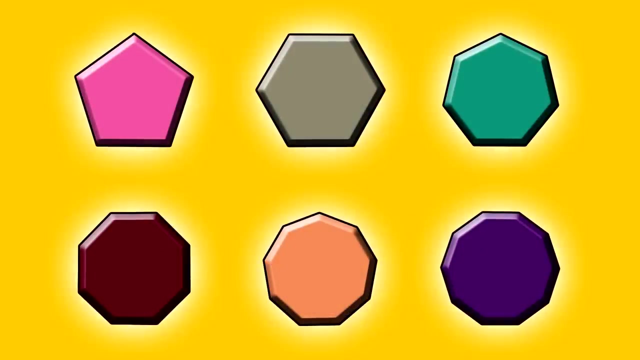 One, two, three, four, five, six, seven. a shape with seven sides is called a heptagon. Heptagon Point to the maroon shape. Let's count the size: One, two, three, four, five, six, seven, eight. a shape with eight sides is called an octagon- Octagon. 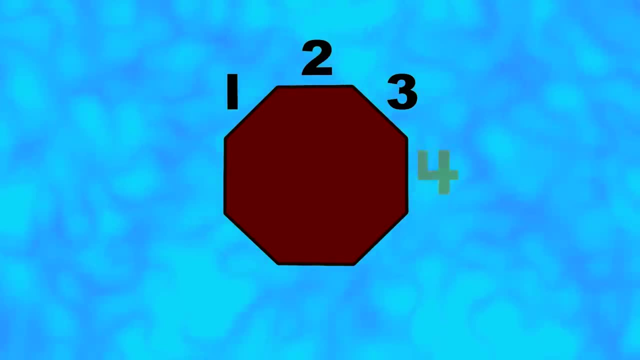 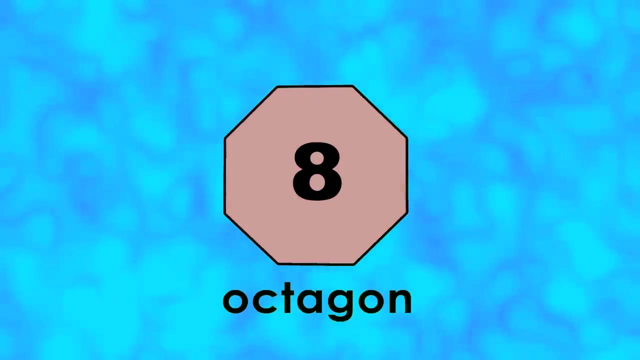 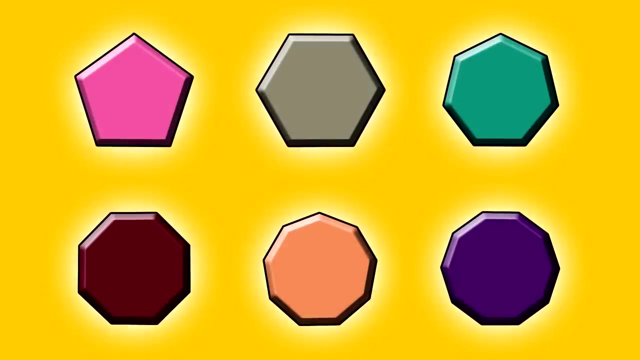 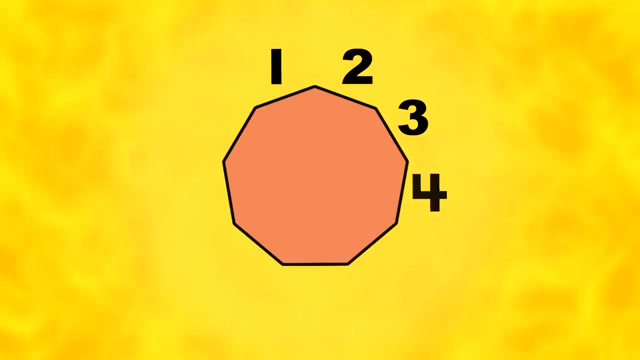 Point to the peach shape. Point to the peach shape: One, two, three, four, five, six, seven, eight. a shape with eight sides is called an octagon. Octagon. Point to the peach shape. Let's count the size: One, two, three, four, five, six, seven, eight, nine. a shape with nine sides is called a nonagon. 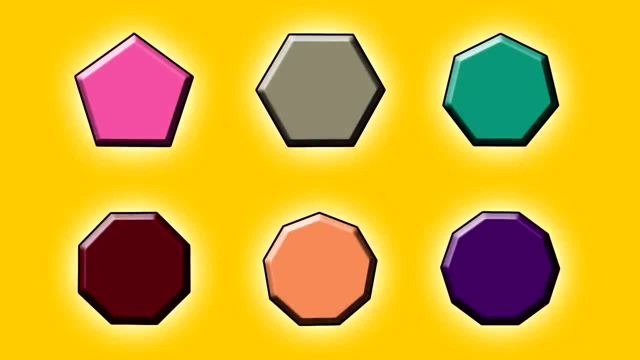 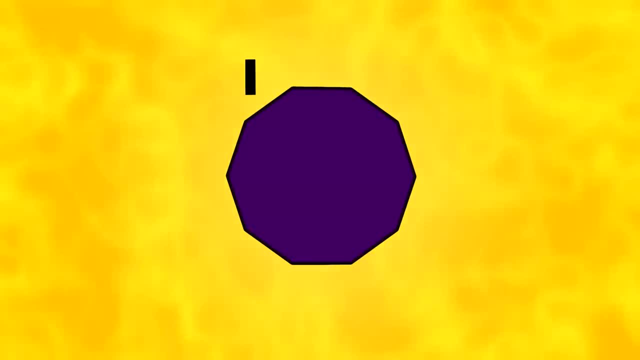 Nonagon. Point to the violet shape. Point to the violet shape. Let's count the size. Let's count the size. One, two, three, four, five, six. a shape with nine sides is called a nonagon. One, two, three, four, five, six, seven, eight. a shape with nine sides is called a nonagon. 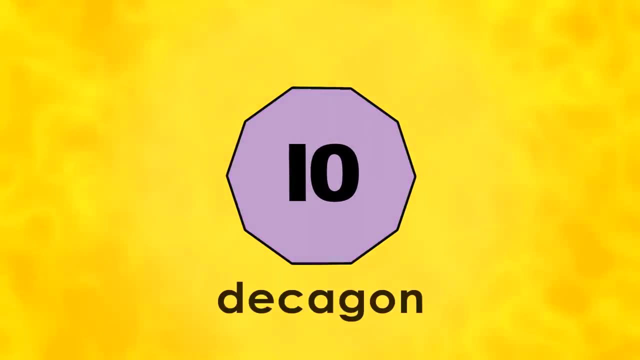 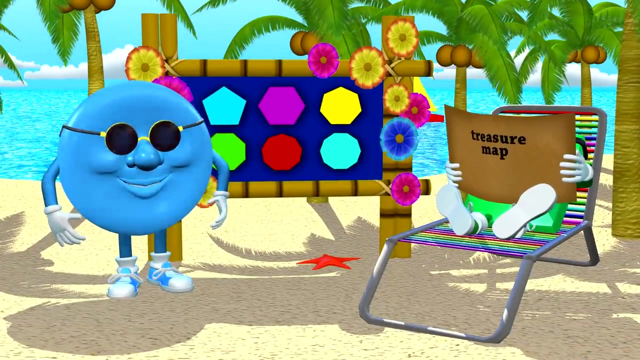 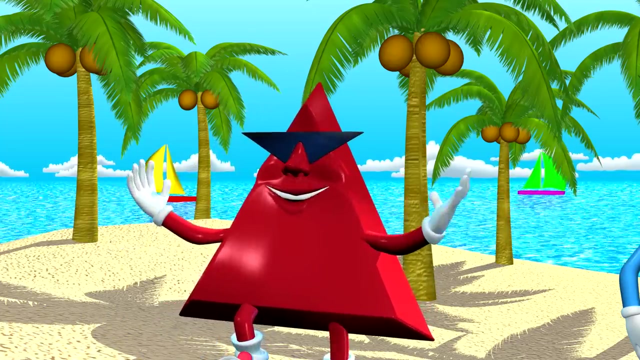 A shape with ten sides is called a decagon. A shape with ten sides is called a decagon- Decagon. Wow, that was fun. but could we sing a song to help us remember all the new shapes? no sweat, Yes, Trolley, could we? No sweat, Let's have a little island music. 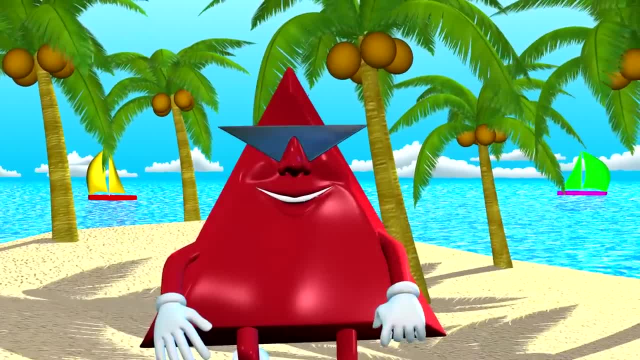 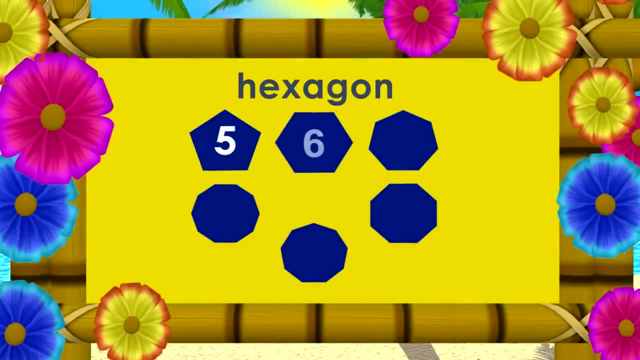 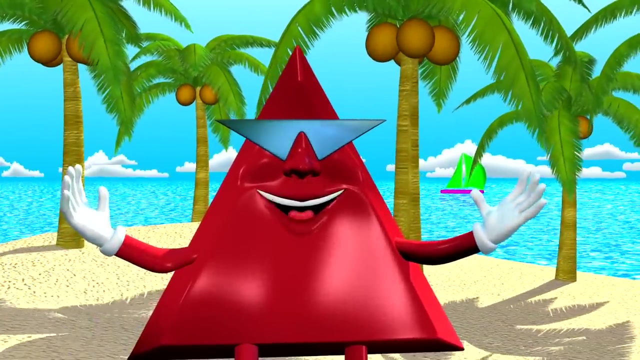 Ah, that's the way. Yeah, Five sides pentagon, Six sides hexagon, Seven sides heptagon, Eight sides octagon, Nine sides nonagon, Ten sides decagon. Ooh, we jammin' man, Let's do it again. 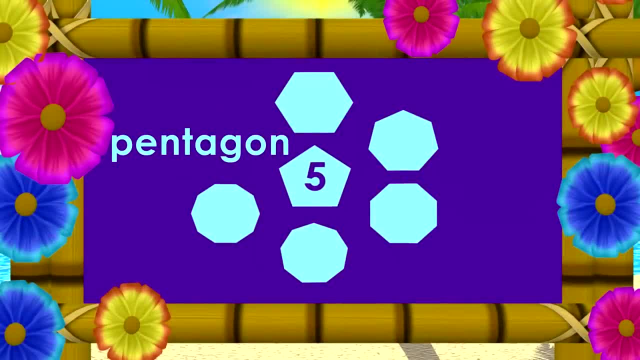 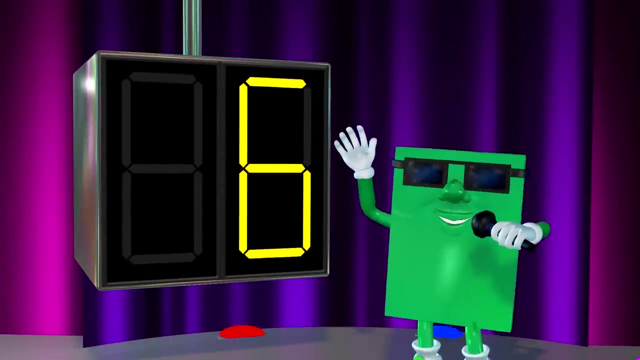 Ha, ha, ha, ha ha ha. Five sides pentagon, Six sides hexagon, Seven sides heptagon. Eight sides octagon. Nine sides nonagon, Ten sides decagon- Let's count to 20.. You know that's plenty. 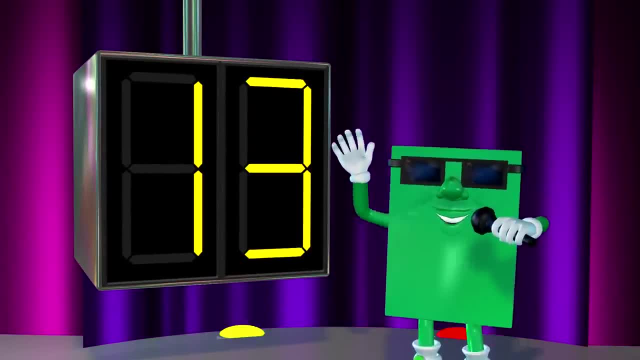 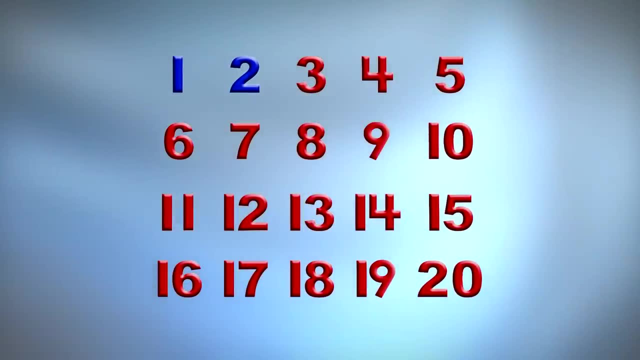 In fact it's many when you count to 20.. If you talk about money, it's more than one penny when you count to 20.. Ow One, two, three, four, five, six, seven, eight, nine, 10,, 11,, 12,, 13,, 14,, 15,, 16,, 17,, 18,, 19,, 20.. 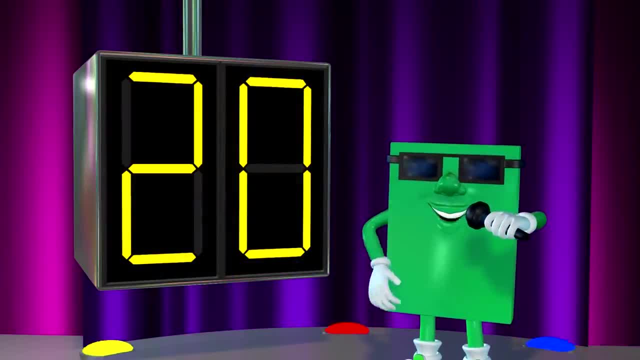 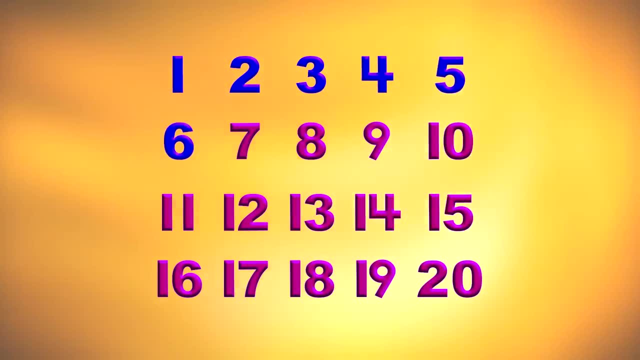 20.. Excellent, Let's count again, but this time a little faster. Let's count again, but this time a little faster: One, two, three, four, five, six, seven, eight, nine, 10,, 11,, 12,, 13,, 14,, 15,, 16,, 17,, 18,. 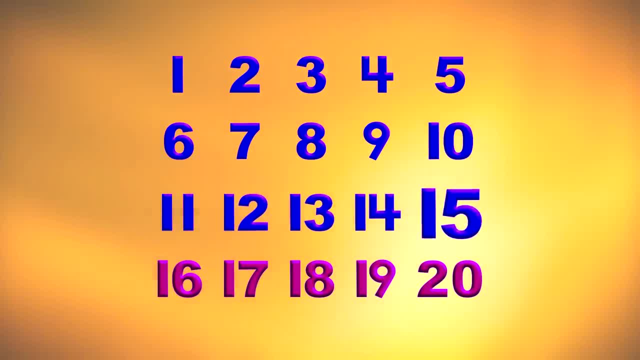 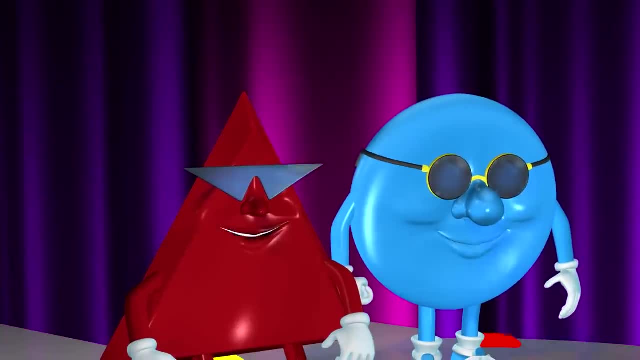 19, 20.. 10,, 11,, 12,, 13,, 14,, 15,, 16,, 17,, 18,, 19,, 20.. Faster, faster, But, Rockford, our tongues are tired. 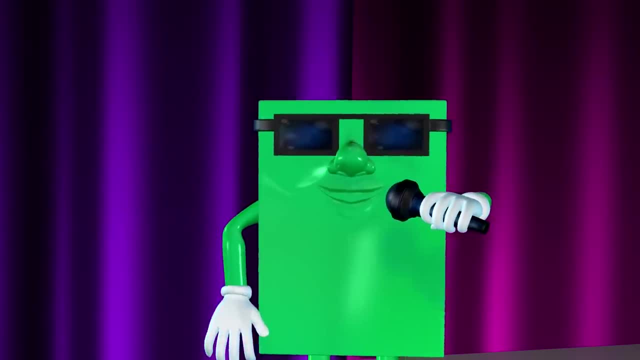 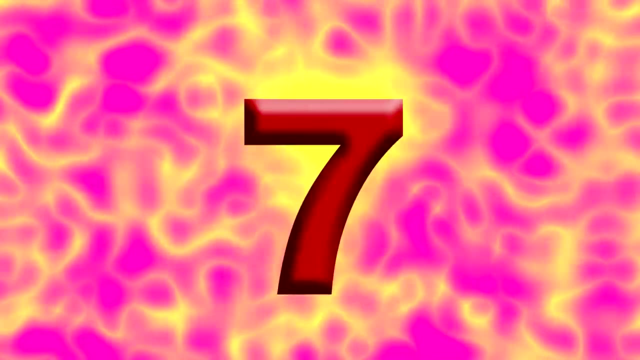 Oh, come now you can do it, faster, faster. But Rockford, our tongues are tired. Oh, come, now you can do it. Oh, pump up the beat. 1,, 2,, 3,, 4,, 5,, 6,, 7,, 8,, 9,, 10,, 11,, 12,, 13,, 14,, 15,, 16,, 17,, 18,, 19,, 20.. 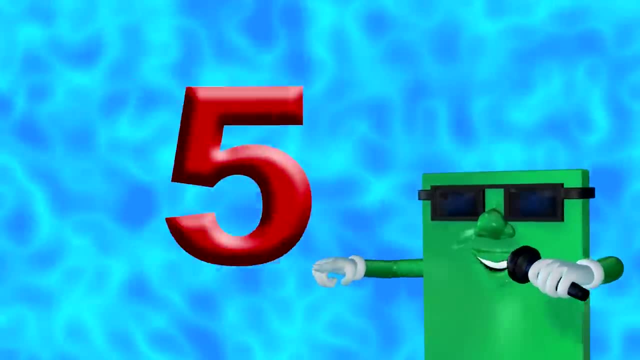 Oh, faster. 1,, 2,, 3,, 4,, 5,, 6,, 7,, 8,, 9,, 10,, 11,, 12,, 13,, 14,, 15,, 16,, 17,, 18,, 19,, 20.. 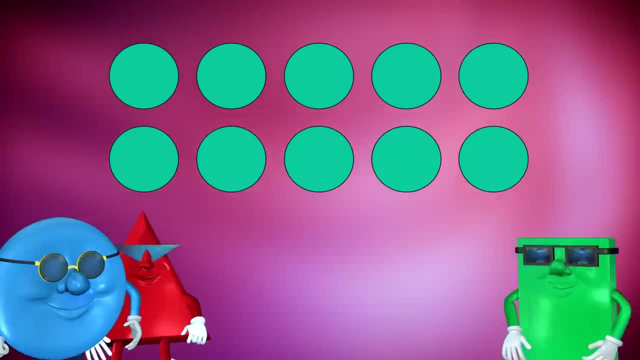 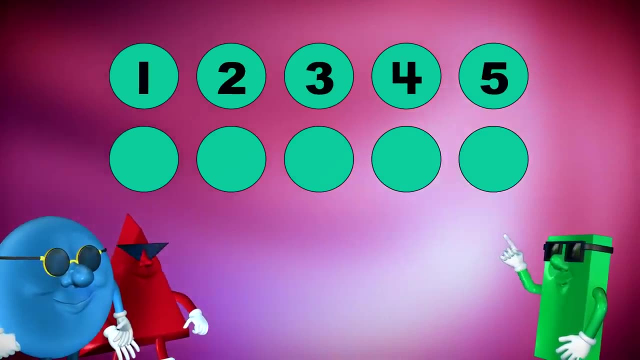 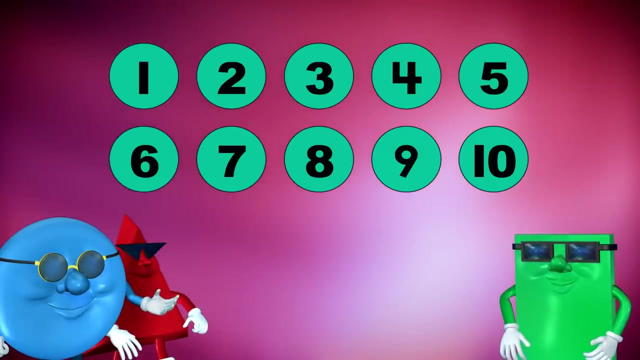 See the circles. Let's count them with Rockford: 1,, 2,, 3,, 4,, 5,, 6,, 7,, 8,, 9, 10.. What color are those circles? That's right, they're turquoise. 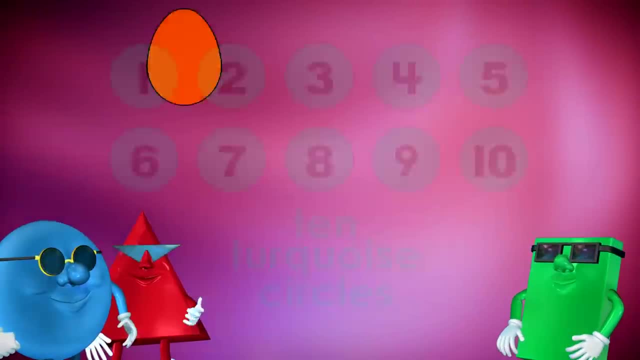 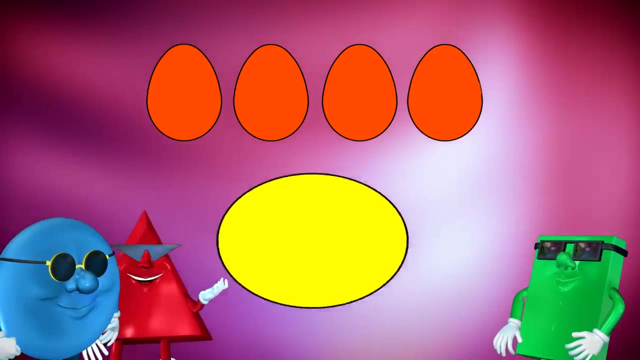 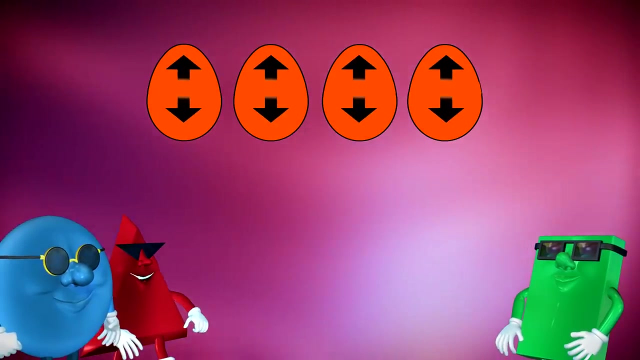 There are 10 turquoise circles. Let's look at the orange shapes. What shape are they? Hmm, let's see A squished circle Shape. might be an ellipse, but they have to be ovals because they aren't the same on both ends. 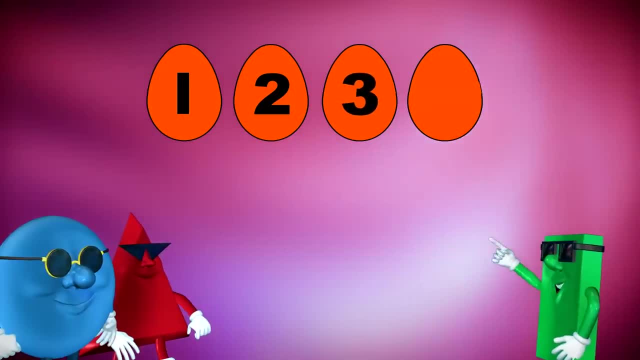 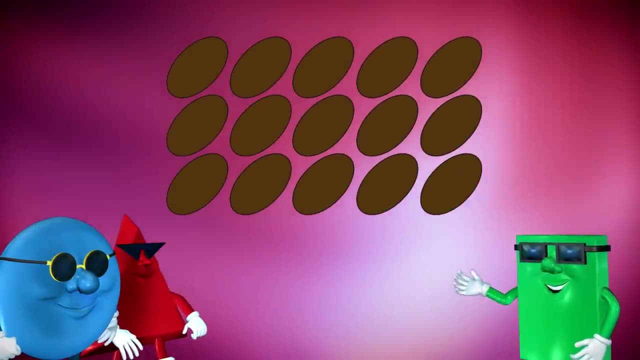 How many ovals are there? 1,, 2,, 3, 4.. Ah, four orange ovals. Let's look at the brown shapes. What do we call that shape? They look like ovals. I beg your pardon, I believe they are ellipses. 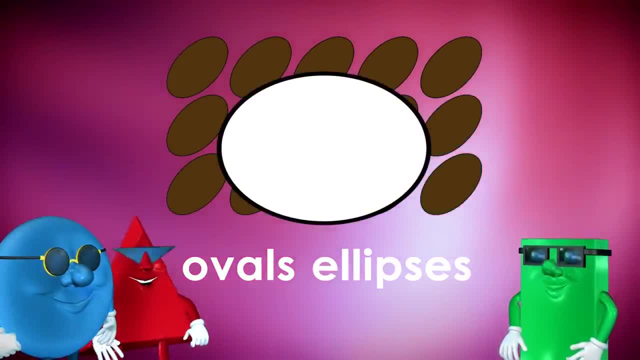 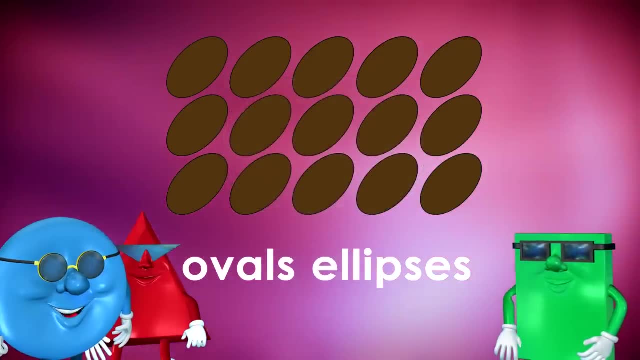 Cool down. you are both right. Remember, an ellipse is a special kind. It's the same kind of oval that is the same on both ends. That's right Now we remember How many ellipses or ovals are there. 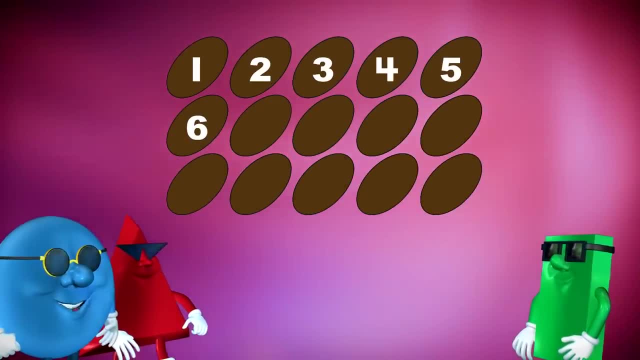 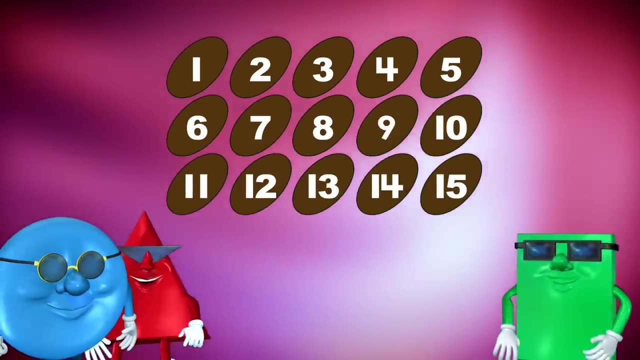 1,, 2,, 3,, 4,, 5,, 6,, 7,, 8,, 9,, 10,, 11,, 12,, 13,, 14, 15.. Far out, 15 brown ellipses: How, totally elliptical. 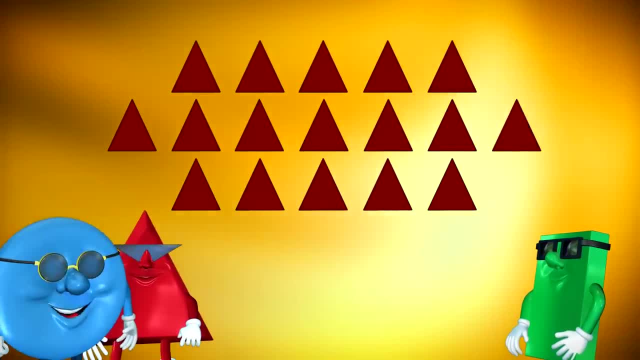 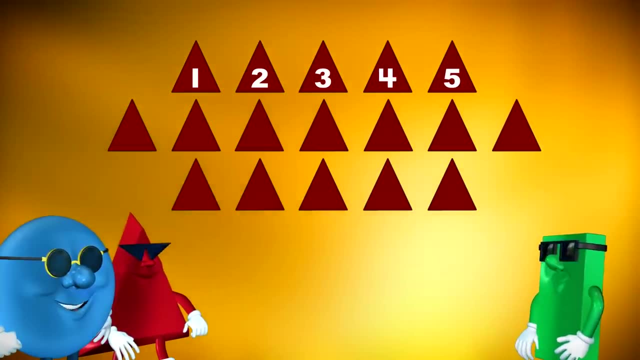 Wow, this is really fun. Let's do some more. Let's count the triangles 1, 2, 3, 4, 5, 6, 7, 8, 9, 10,, 11,, 12,, 13,, 14,, 15,, 16, 17.. 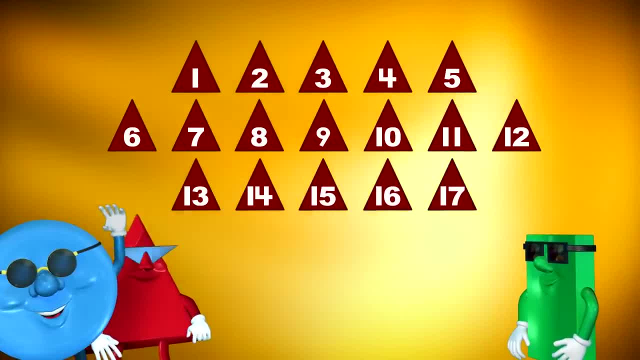 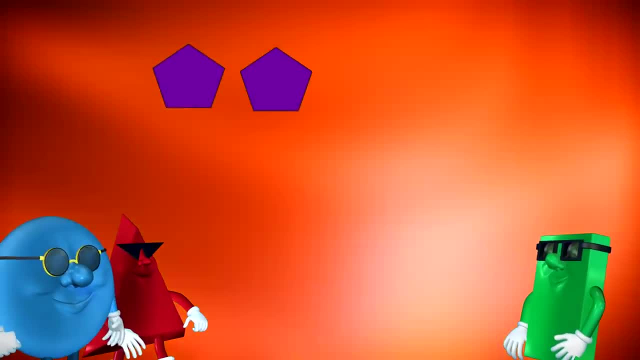 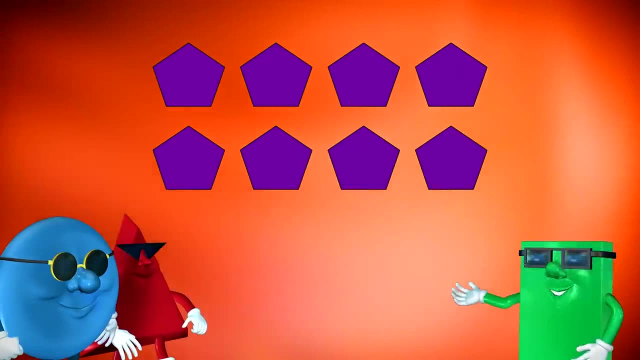 But what color are those triangles? I know they're maroon. I see 17 maroon triangles. Do you remember what the purple shapes are called? I believe we need to count the sides on one of these shapes, don't we? 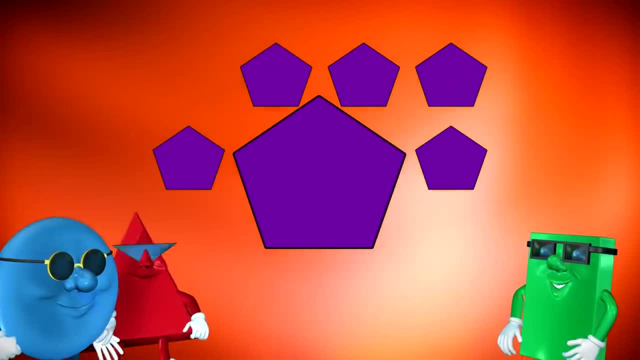 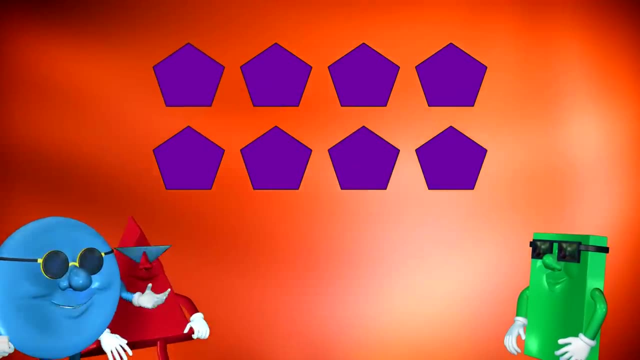 Sounds cool to me. Oh, splendid, let us proceed. 1,, 2,, 3,, 4, 5.. There are five sides, so they must be pentagons. All right, you got it. Now let's count the pentagons to see how many we have. 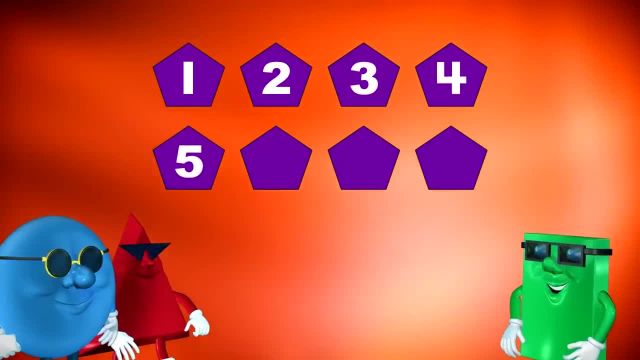 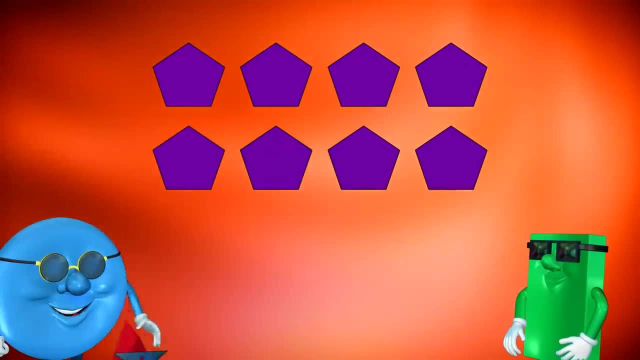 1,, 2,, 3,, 4,, 5,, 6,, 7, 8.. Neat, We have eight purple pentagons. Each one has five sides. And remember, sometimes the color purple is called violet. 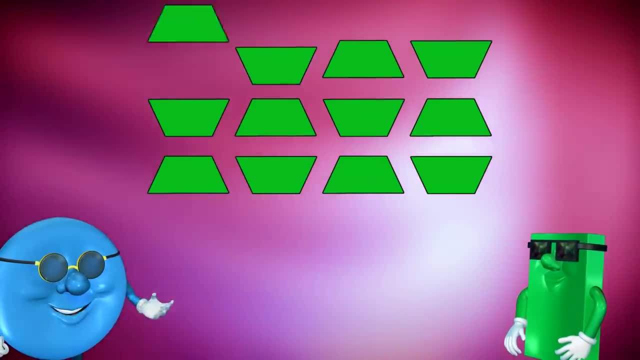 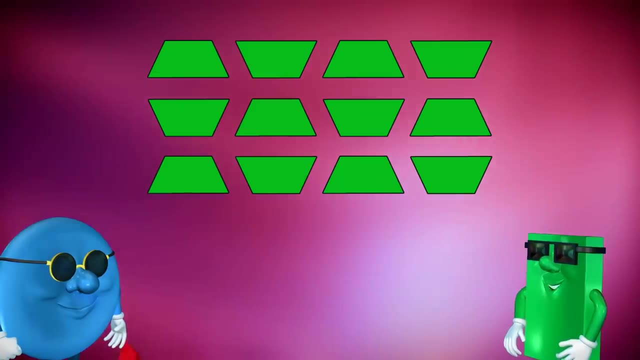 Next, let's look at the green shapes. Oh, what shape are they? This is a tough one, but I think they are those tricky trapezoids. That's right, they are trapezoids, But how many trapezoids are there? 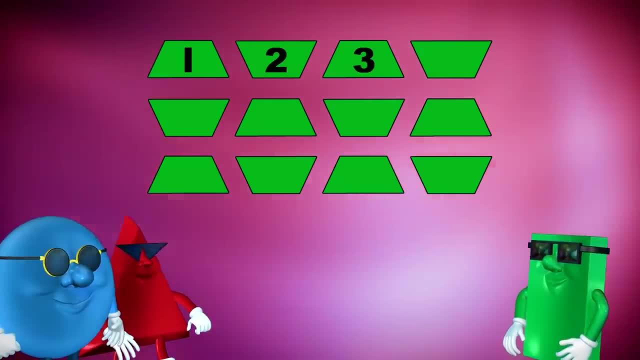 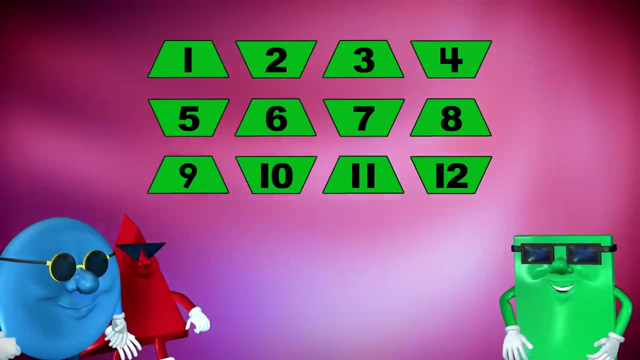 1,, 2,, 3,, 4,, 5,, 6,, 7,, 8.. 9,, 10,, 11,, 12.. Yes, there are 12 green, trapezoids. Stay cool people. 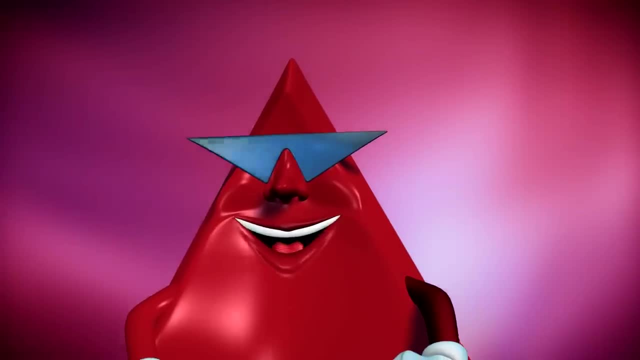 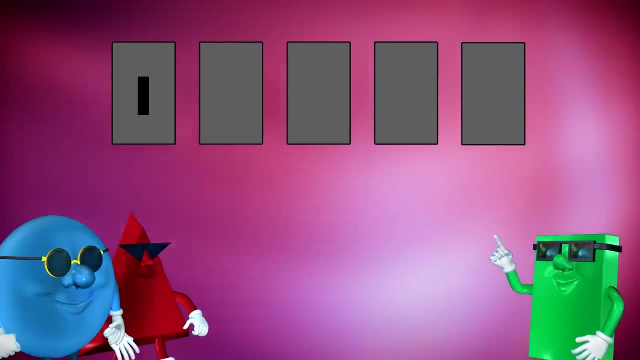 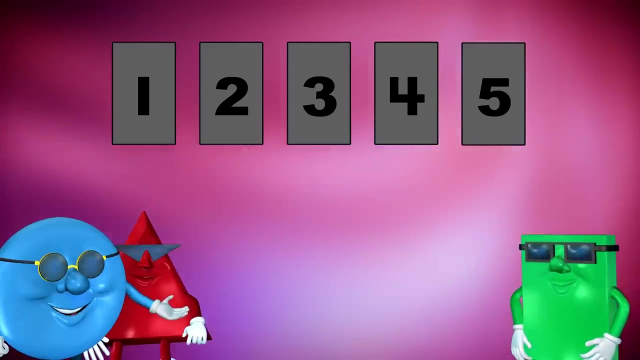 We're just getting started. Let's count the rectangles. But of course 1,, 2,, 3,, 4, 5.. And what color are those rectangles? They're gray like an elephant. They're green like an elephant. 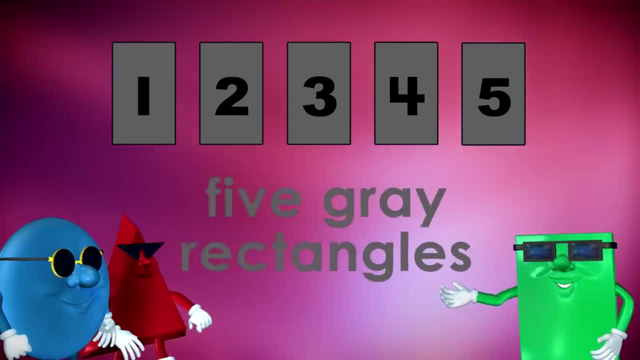 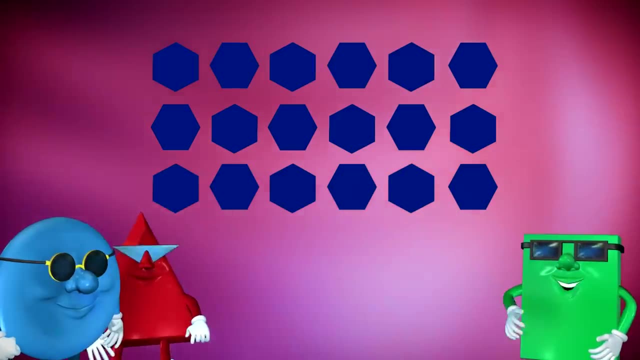 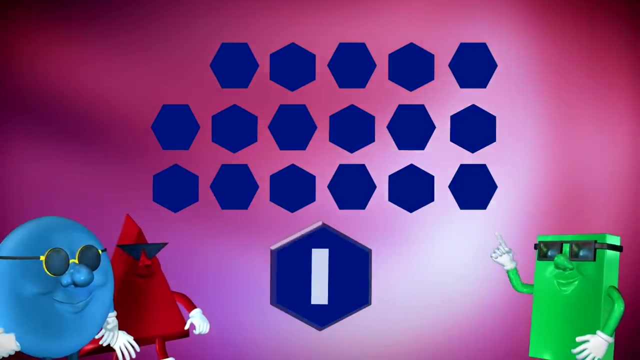 Therefore, we have five gray rectangles. I say, what do you call those blue figures? Remember, man, you need to count the sides on one shape. Why, that's wonderful, Let's count them 1,, 2,, 3,, 4,, 5,, 6.. 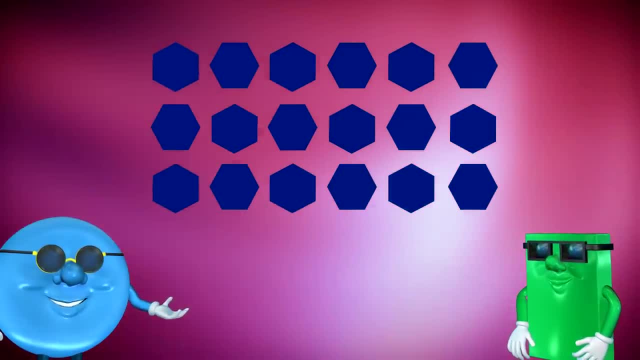 Six sides on each shape. That means they must be hexagons, Right, Trolley, That's right Blue hexagons. But how many blue hexagons are there? There are so many of them. Let's see if we can count them all. 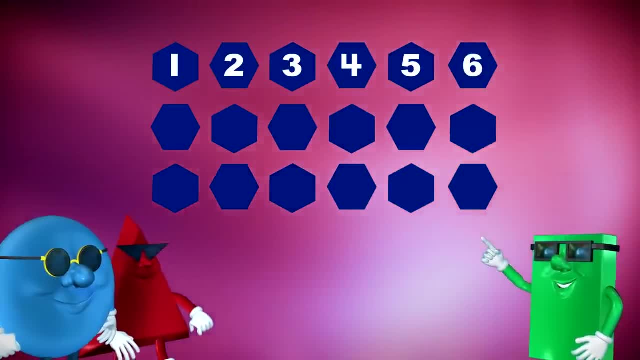 1,, 2,, 3,, 4,, 5,, 6,, 7,, 8.. 9,, 10,, 11,, 12,, 13,, 14,, 15,, 16,, 17, 18.. 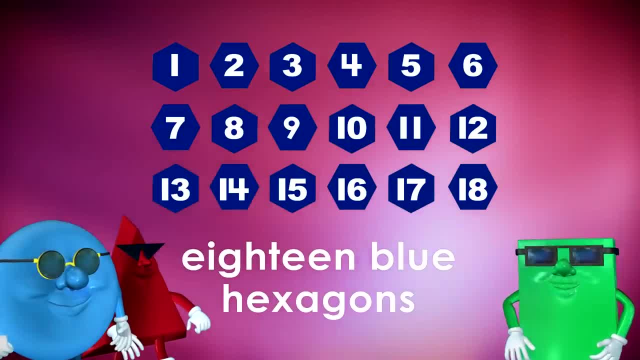 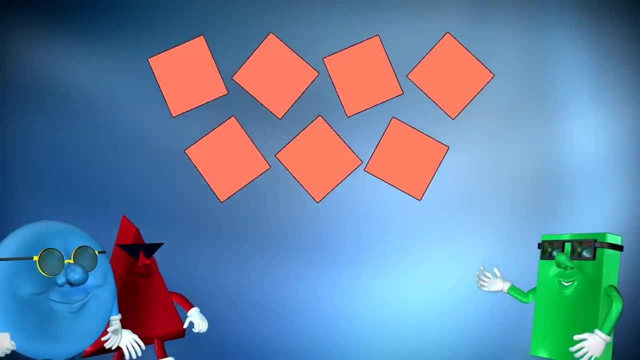 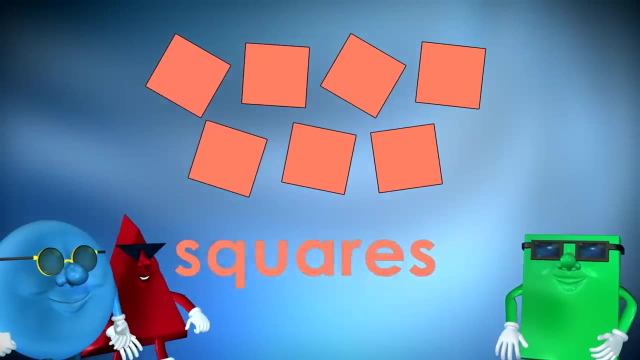 There are 18 blue hexagons. Ooh, Look at the peach shapes, Oh dear, They're turned all different directions. Yeah, man, But no matter how you look at them, those shapes are squares. Let's find out how many peach squares there are. 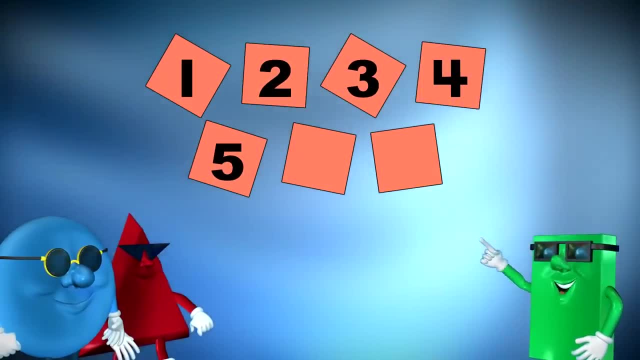 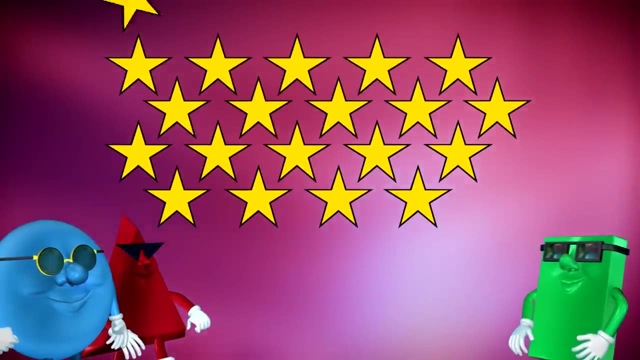 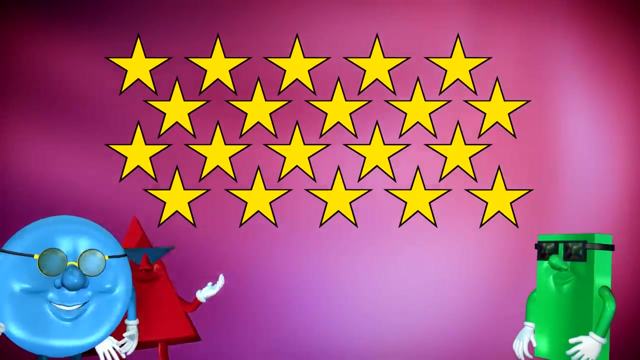 1,, 2,, 3,, 4,, 5,, 6, 7.. Seven peach squares- Oh my, I think I'm seeing stars. You are? What color are they? They are bright yellow And there are so many of them. 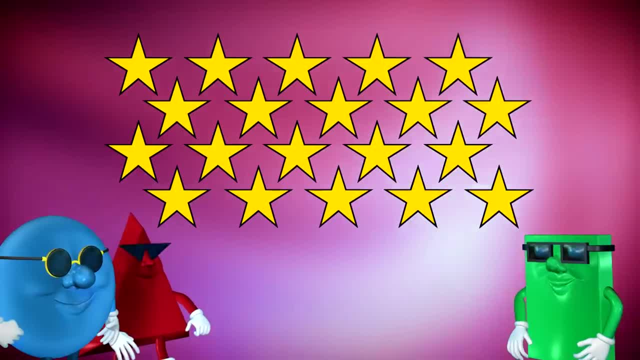 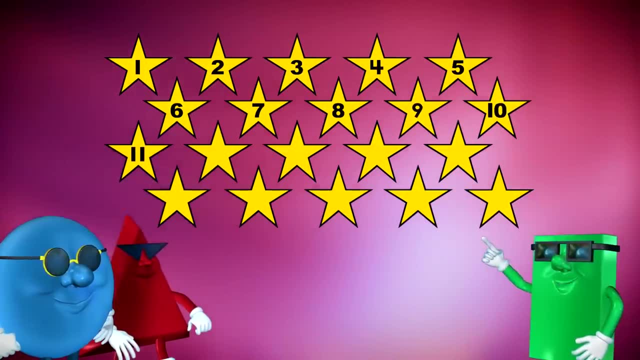 Don't fret, I'll help you. count them all: 1,, 2,, 3,, 4,, 5,, 6,, 7, 8.. 9,, 10,, 11,, 12,, 13,, 14,, 15,, 16,, 17,, 18,, 19, 20..